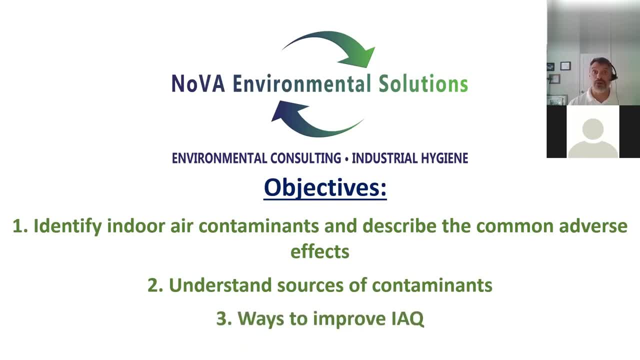 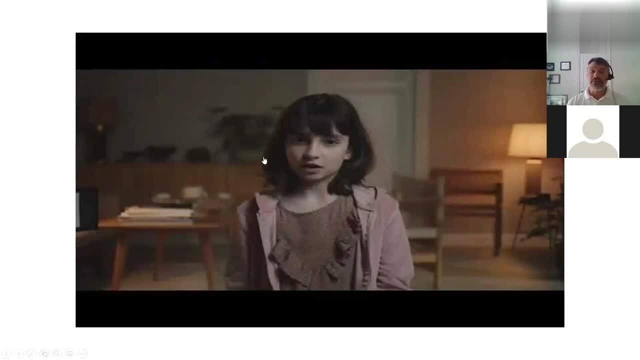 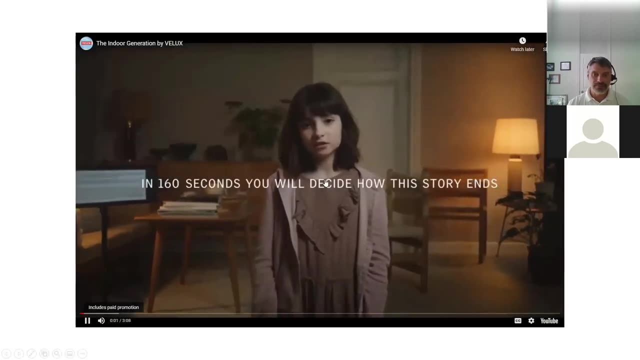 And then also the most importantly, are ways to improve our indoor air quality and help to prevent or improve our indoor air quality. We're going to start off with this short video. hopefully It will get rolling, and it should. In 160 seconds, you will decide how this story ends. 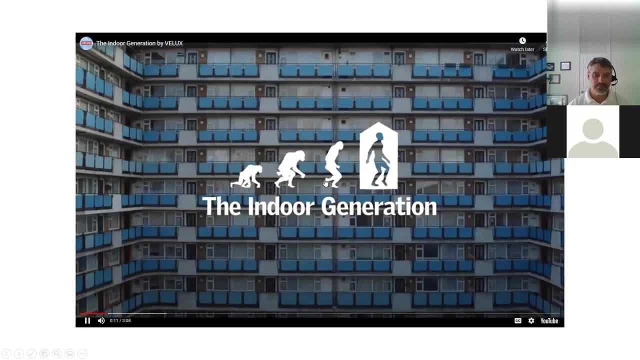 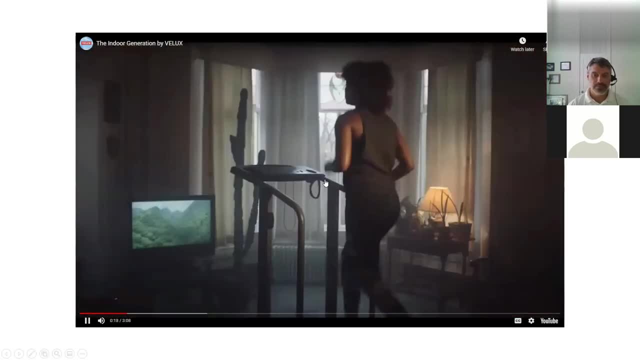 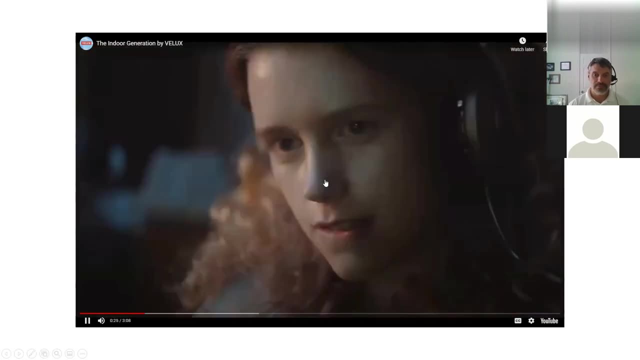 This is a story about us, the indoor generation, a generation that spends 90% of its life indoors. It all started the day we left nature behind. We filled our homes with lovely things and all the stuff we wanted. Our homes became places you would never want to leave. 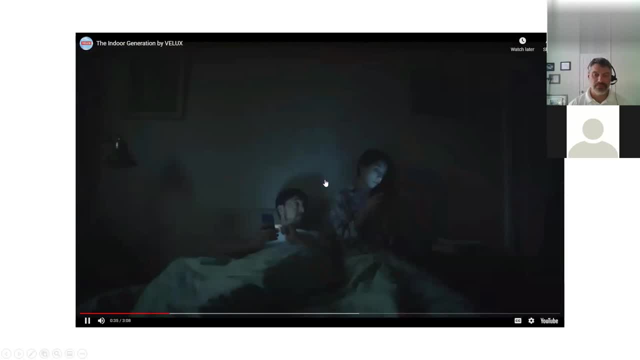 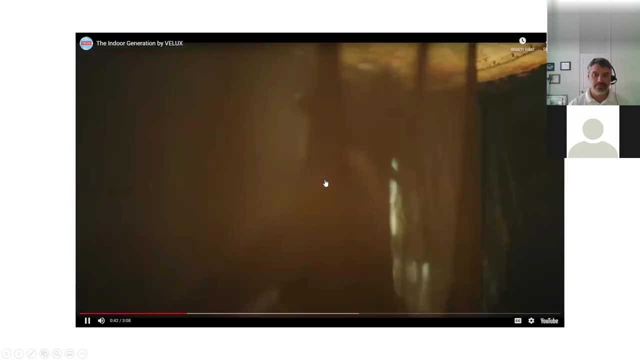 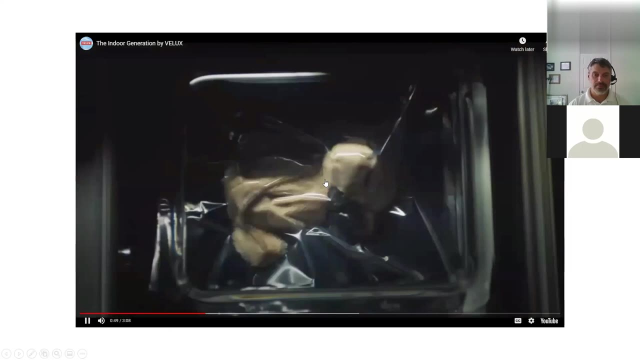 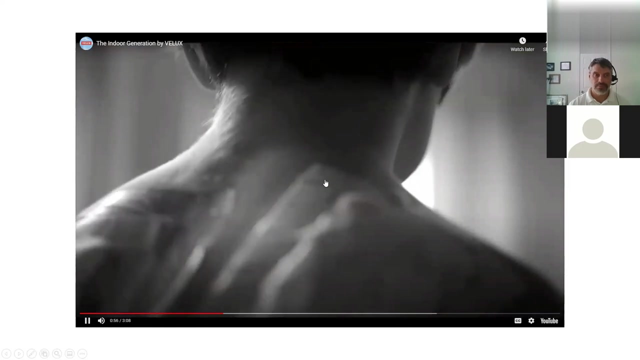 Artificial light replaced daylight And we built our houses so that nothing could escape. We cooked and showered, breathed and prayed, slept and sweated. We had closed ourselves in to a point where nothing could get out, But our house was always a place where we found our sense of presence. 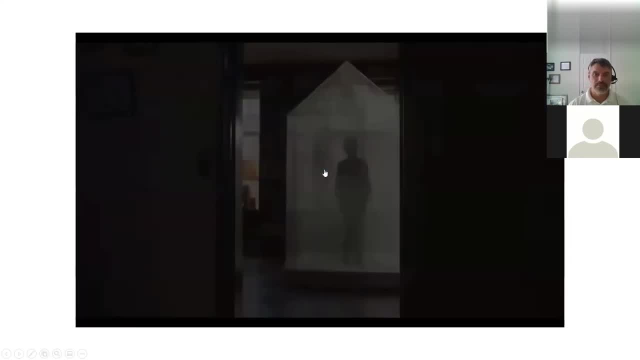 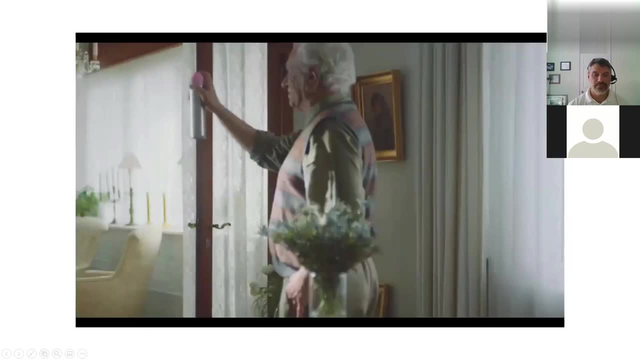 Like our home. It was our home, Like our life. We're not alone here. We're hanging out together. It's never school. We are not alone. We are not alone. We are not alone. We have created spaces for learning, for learning for our kids, for teaching and for. 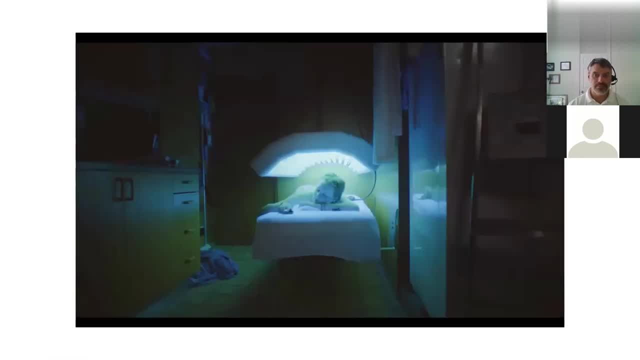 our kids to grow. We are not alone here. We are not alone. We are not alone here. We are not alone to learn. So when the air turned bad inside, we tried fixing it with chemicals. We went to school. We put in little artificial suns everywhere to make the darkness bearable. 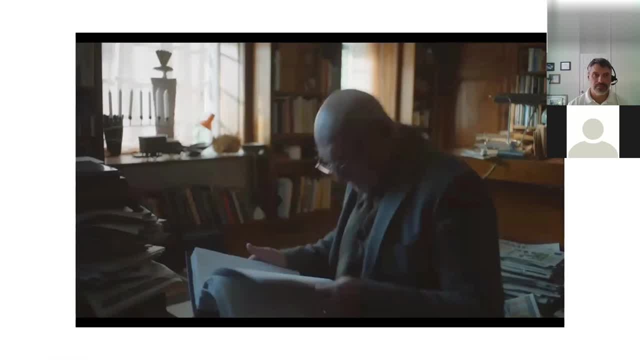 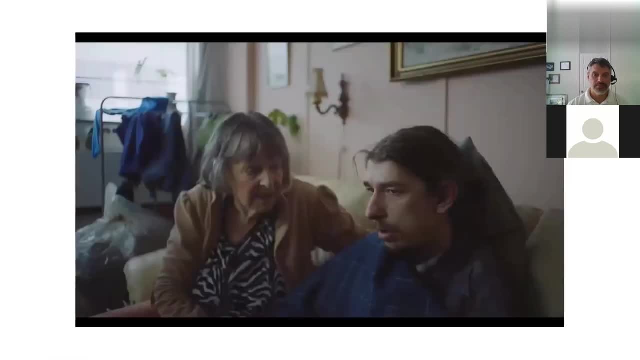 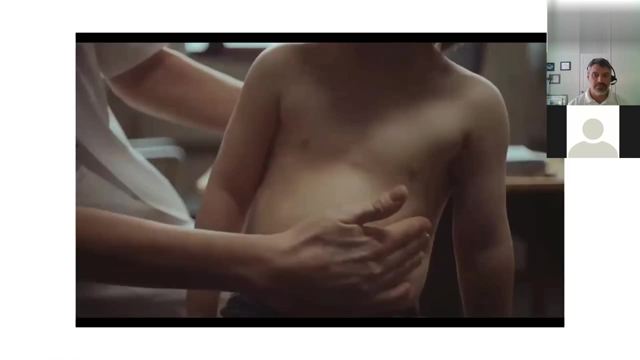 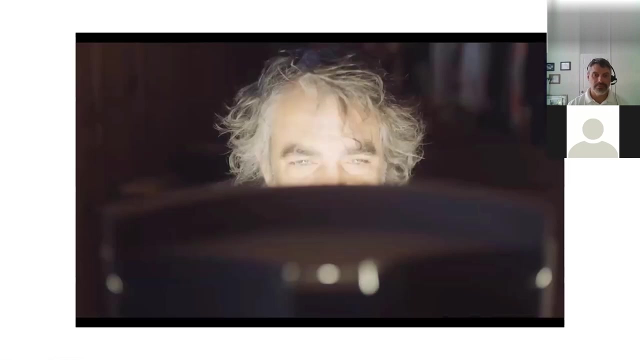 That's when things started to happen, Hard to notice in the beginning, Until we found out that they didn't exist before. some needed help to sleep, to breathe, to not itch. many of us even started to feel sad. so we turned on happy lamps to make the sadness go away. 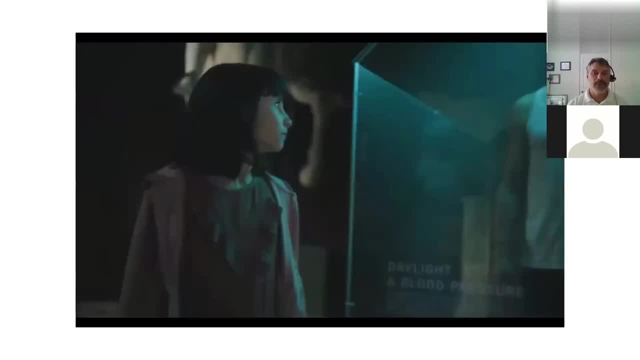 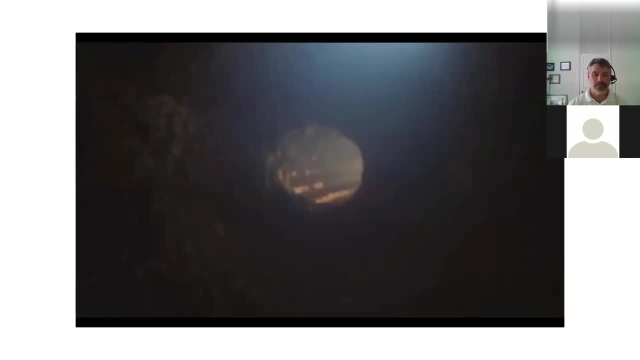 then scientists discovered that the air inside our homes is up to five times more polluted than the air outside, and that the lack of daylight can affect children's learning and increase blood pressure. it turns out that kids rooms often have the highest concentration of toxicants in the 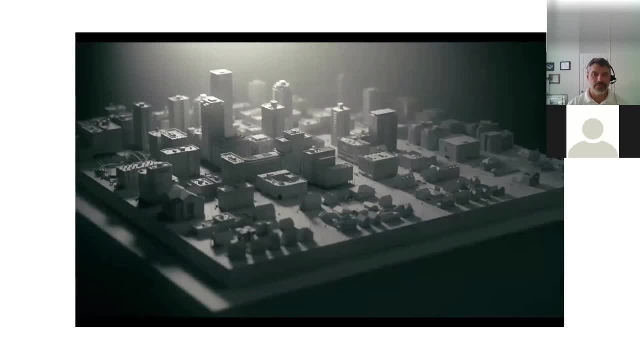 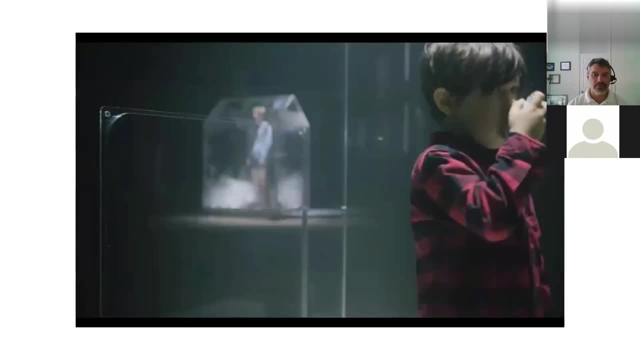 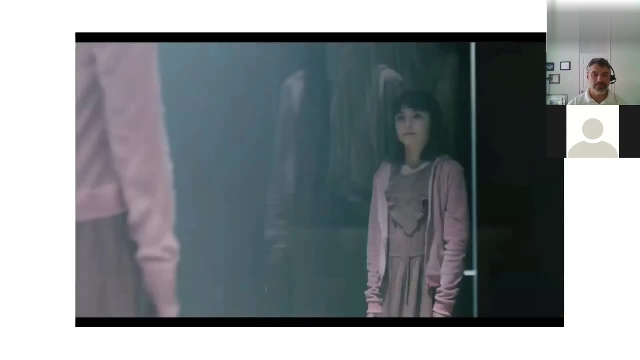 house. in fact, millions of homes are unhealthy to live in. they discovered that the air inside our homes is up to five times more polluted than the air outside. they discovered that living in damp and moldy homes increases the risk of asthma by 40, and i learned that millions of people like me suffer from asthma and allergies caused by a bad indoor environment. 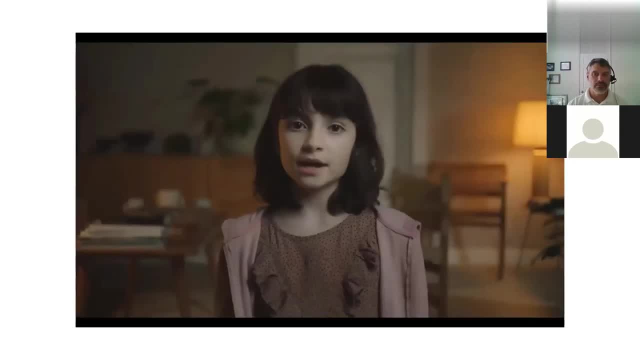 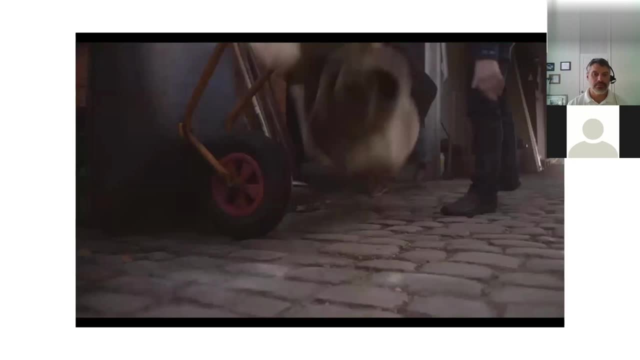 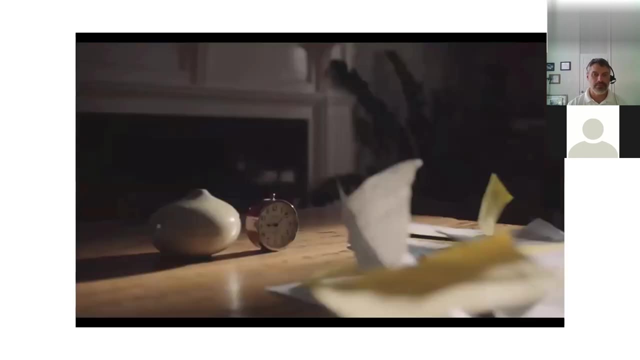 and so here we are. how this story ends is up to you, because it's not written yet. if you care about the inner generation, do something again to think and live differently. let light and fresh air into your life again. even small changes can make a huge difference for coming generations. learn how at theindoorgenerationcom. 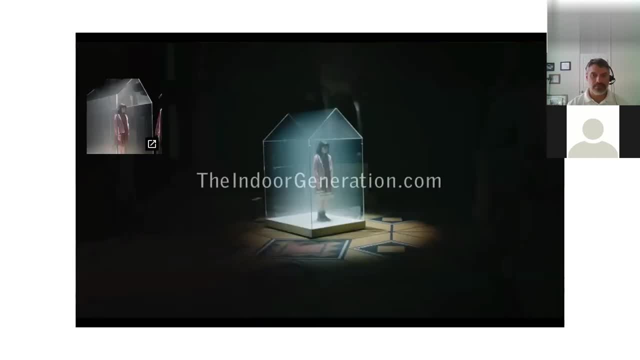 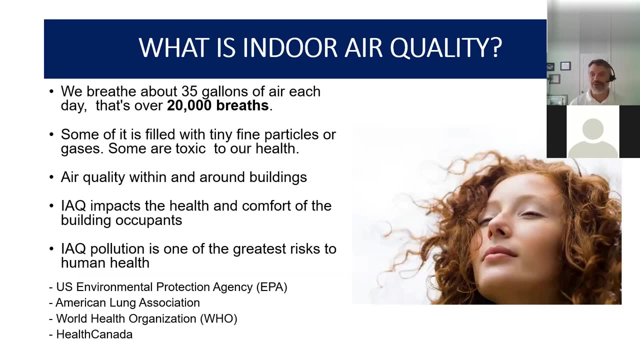 so that video is actually viewed. i think right around four million times now, but it's just a nice powerful video in my opinion. uh, to kind of get a give, give you a feel of you know what we're really dealing with in many cases. so what is indoor indoor air quality and what's it all about? 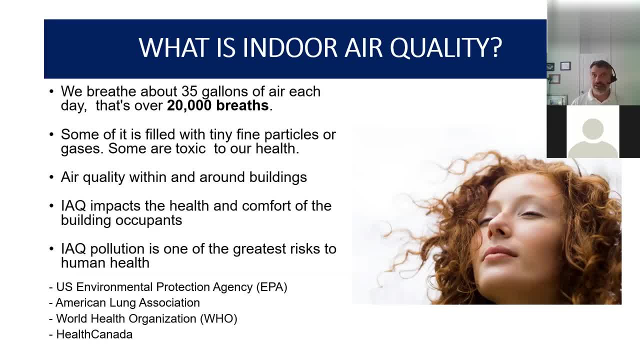 so we breathe roughly about 35 gallons of air every day. that's about 20,000 breaths, and a lot of it is filled, or air is filled with tiny particles, some uh gases- and we're always around something in the air uh- and some are toxic and can be toxic to our health. so but air quality is uh. 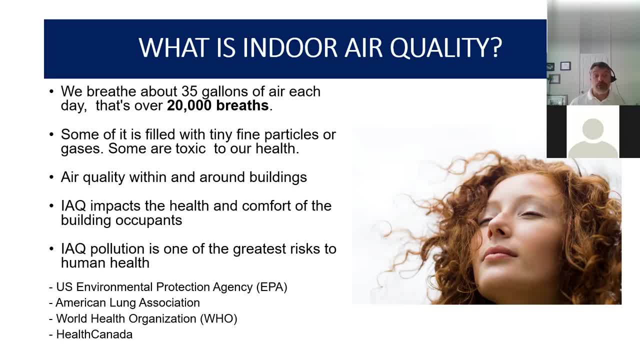 is when we're assessing air quality. it's both the air quality within and around our buildings and our houses, uh, but indoor air quality does impact and can impact the health and comfort of building up occupants and, according to the uscpa, american lung association, world health organization, health canada- indoor air quality pollutants are one of the greatest risks. 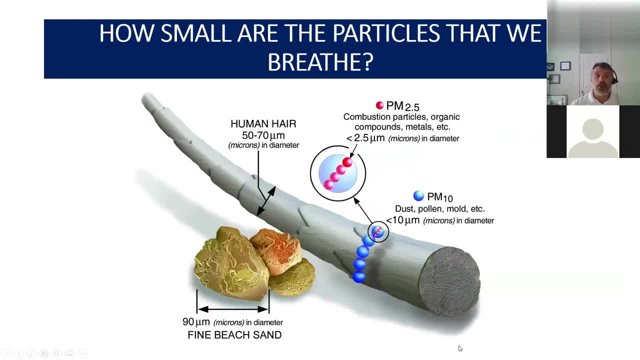 to human health. um so, how small are what are we breathing? how small are these things? so i'm going to try to use- hopefully this works- a little laser pointer here. so right down here, this is about the size of a grain of sand, which is 90 microns in. 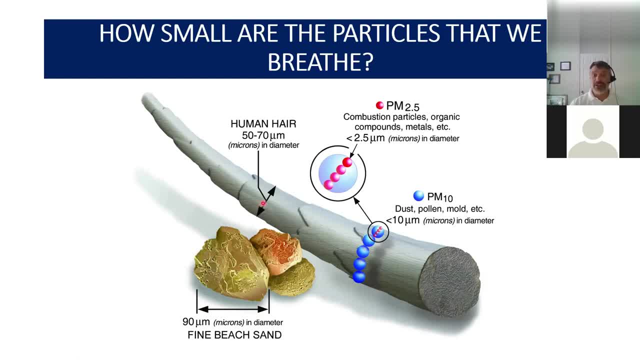 size. a human hair- that's what this represents- is about 50 to 70 diameters in uh microns in diameters. so a lot of the stuff that we're breathing every day- dust, pollens, molds, mold spores and other uh- other common uh particles. they're generally what's referred to as pm10 or 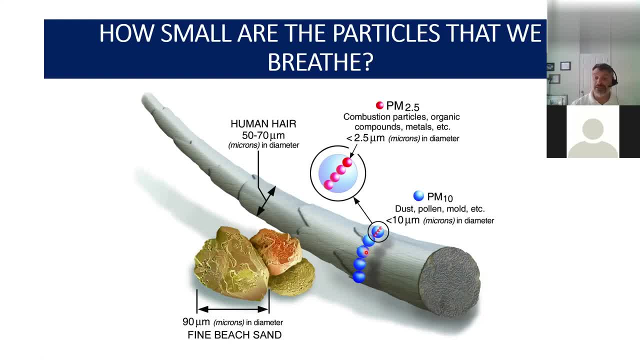 a particulate matter that's about 10 microns in size or or lower. and that's right here, these little blue balls, and then you'll see these little pink dots. those are what's called the tiny particles, or pm 2.5, and we are breathing those every day and that could be, uh, combustion. 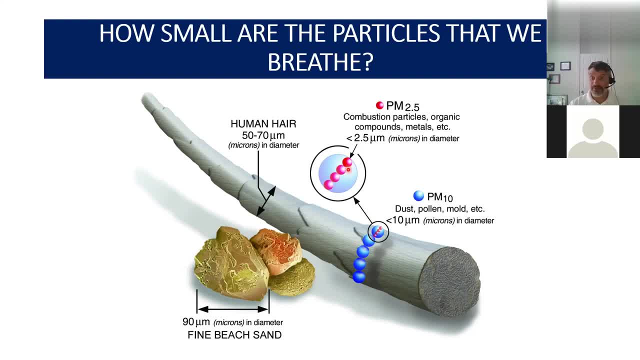 particles, uh. organic compounds, uh, volatile organic compounds, other metals? i can't say that. going back to molds, um, specifically for mold spores, they could range generally range between two microns to 10 microns in size, depending on the species and the types of molds. uh, so that just kind of gives you. 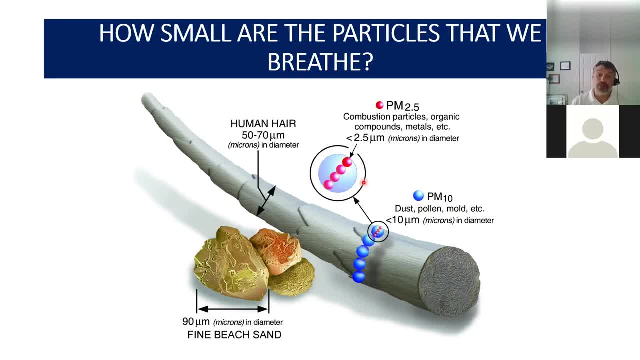 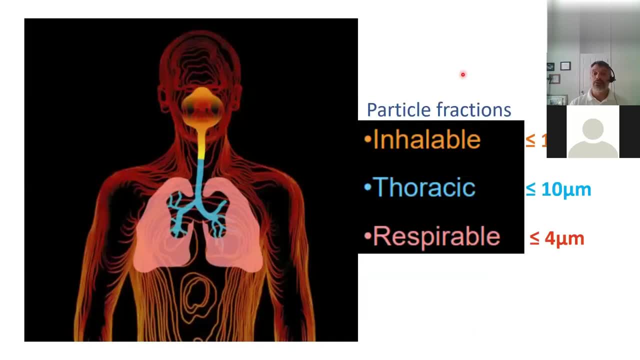 a reference of the size of the particles and the size of the stuff that we're breathing in every day. so i'll move into the, the next slide, which goes into where these, where these particles end up and where all these uh, uh uh articles and fragments end up. so 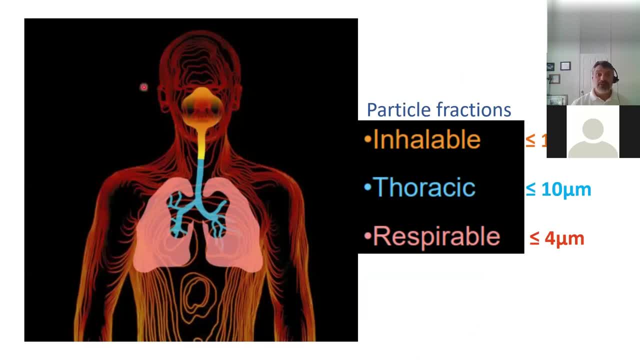 the particle fractions, so the inhalable ones. those end up, yeah, in our nose and our mouth and generally, uh right up in here, and those are the larger particles which our body gets rid of naturally, uh easily. the smaller particles, uh, which are known as the thoracic fractions, if you will. 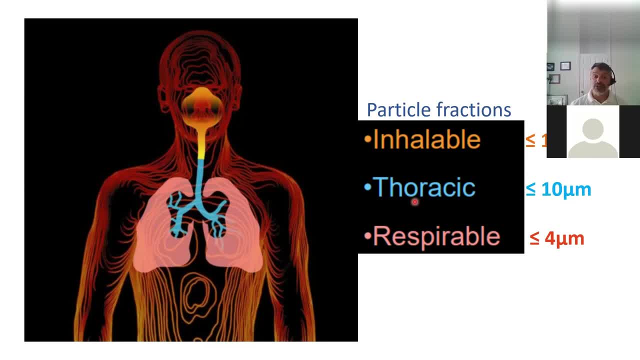 uh, those are ones that are generally about 10 microns or smaller. so those could get past the larynx and into this area of the of the lungs, of the um, in here into the lungs and then into the cilium and then finally the tiniest particles are the respirable particles. those are the less 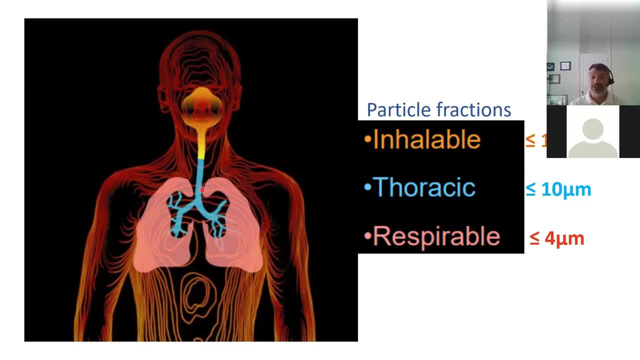 than four microns. generally is is the is the fractions uh for respirable respirable particulates, and some of those can include mold spores and then other other part uh, other tiny particulates. those are the ones that can get embedded into your actual lungs. go past the cilia. 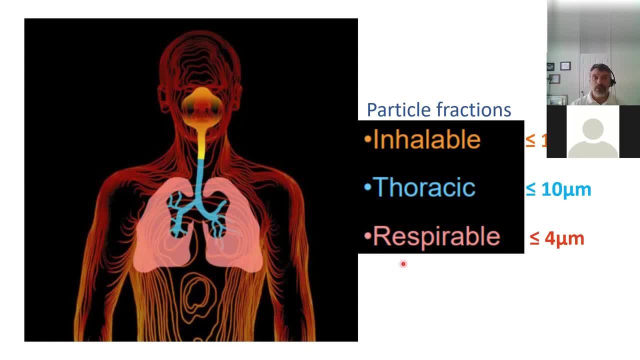 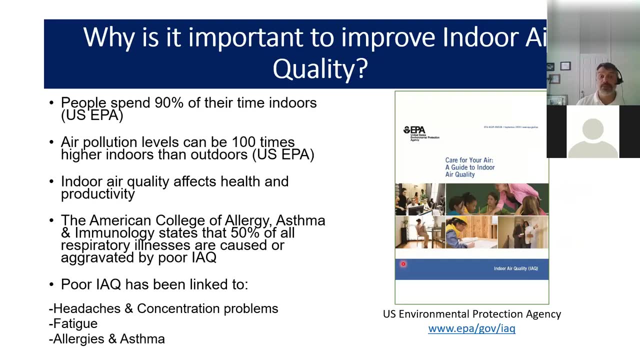 and get inside of your lungs. so why is it important to get into your lungs? important to improving indoor air quality and we'll get into that. so people spend about 90 percent of their times indoors. uh, air pollution levels um in the videos and they said like five times. 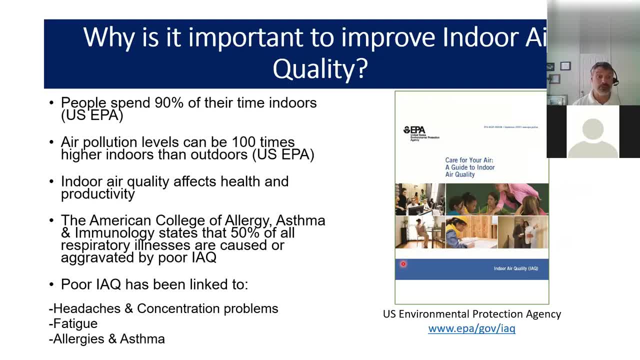 well, epa has done a study not too long ago that air pollution indoors can be sometimes up to 100 times higher indoors than outdoors, and indoor air quality not only affects health, but it can affect productivity of your children, of you at work, um and uh. so that's why uh. 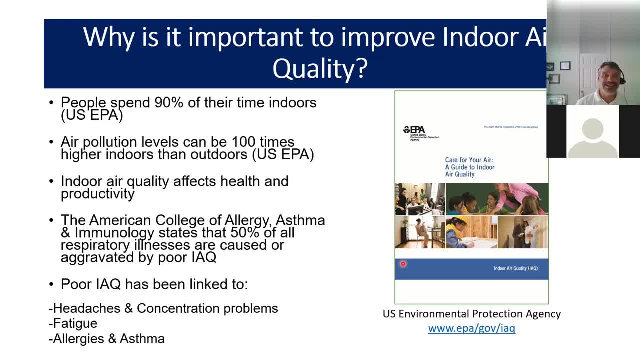 not just immediate health effects, uh, but also again your, your productivity um. the american college of allergy, asthma and immunology states that 50 of all respiratory illnesses are caused or aggravated by poor indoor air quality, and indoor air quality has been linked to various health effects. most common symptoms, or, i'm sorry, the most common adverse health effects, are: 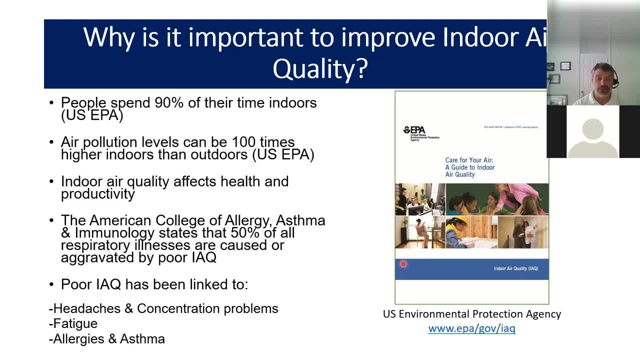 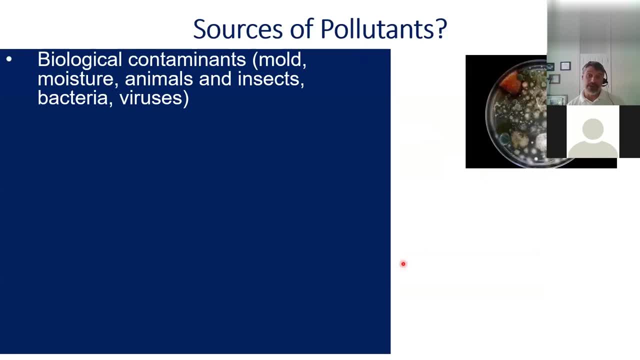 allergies and asthma, fatigue, headaches, concentration problems. so what are sources of pollutants? and this is the uh where we're going to get into some of the uh contaminants. we've got biological contaminants, molds and moisture, animals, insects, bacterias, viruses, uh. those are biological contaminants. uh temperature, relative humidity extremes- they are major functions of indoor air quality and i'll get into that next. 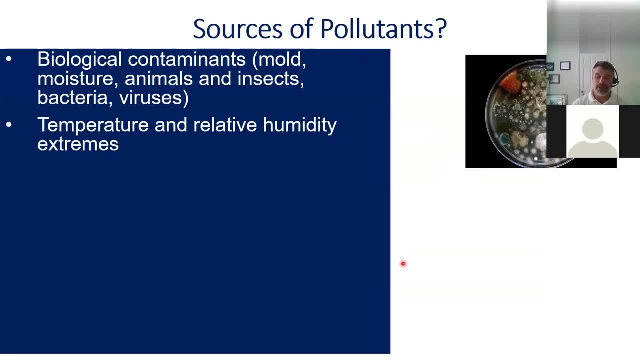 but uh, they, they certainly play a major role in indoor air quality. uh, particulates from smoke outdoor air, uh, cleaning supplies, uh or just cleaning in general. and it can be smokes from burning candle, burning incenses or other smoke fireplaces, things of that nature. inadequate air circuit, air circulation and. 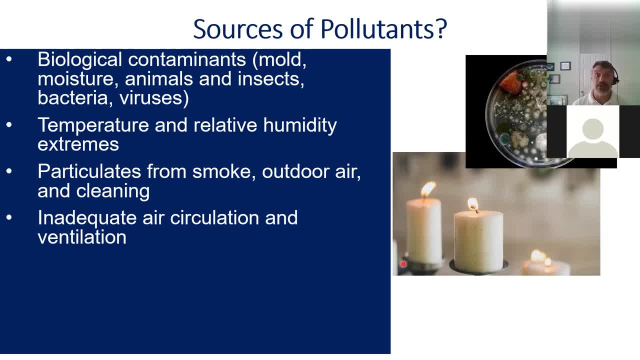 ventilation. are you getting enough fresh air in the house? is there enough, uh, air circulation in your building where you're working? fresh air in your building? is there enough fresh air in your building? so, uh, if there's inadequate air circulation or ventilation, that could increase the indoor air. 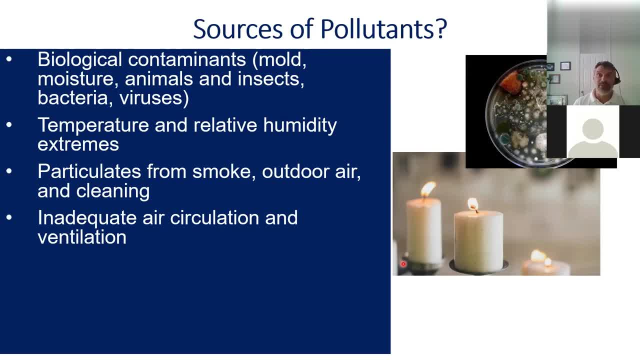 quality pollutants and actually can create an environment that may make it more conducive for biological contaminants to exist and thrive. carbon monoxide is a major pollutant source that i'm sure many or most of you are aware of and have heard of, and volatile organic compounds that you just had a little picture and there's. we're going to get into that in a moment, but i'm 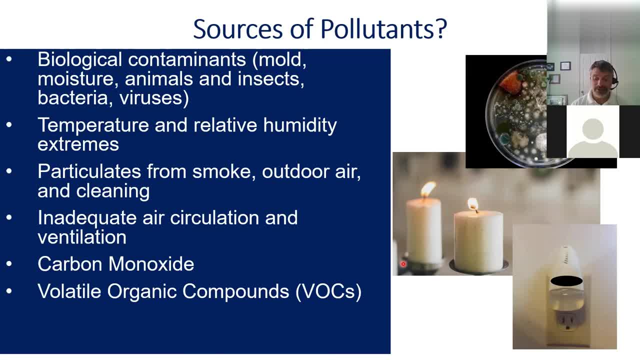 going to get into that in a moment. but i'm going to get into that in a moment, but i'm going to get into that in a moment. volatile organic compounds- um in this, in this presentation. and then radon is another major pollutant source, especially in this region. so i wanted to get into how i talked about temperature. 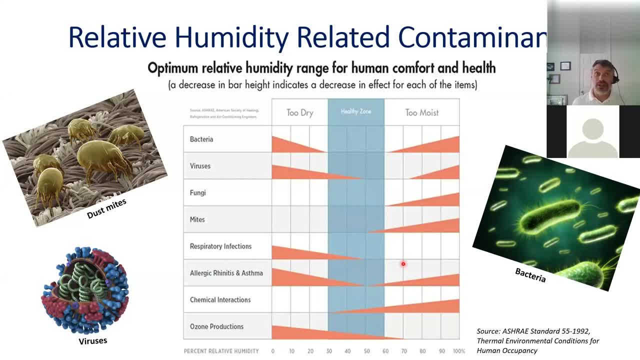 temperature and relative humidity and how their major functions of indoor air quality. but this chart, which is supplied by the american society of heating, refrigeration and air conditioning engineers, gives us a pretty good sense as to how relative humidity is going to affect the air quality. humidity uh can affect not only human comfort but if increase or or affect other contaminants. 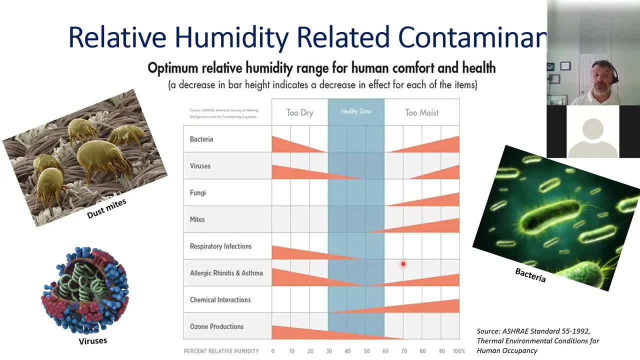 the general recommendation is to keep humidity between generally between 30 and 60 percent indoors all year round. optimal is right around 50 percent at all times, even if you're away from the house, keeping humidity around 50 percent year round. so what? this graph? or this, this table? 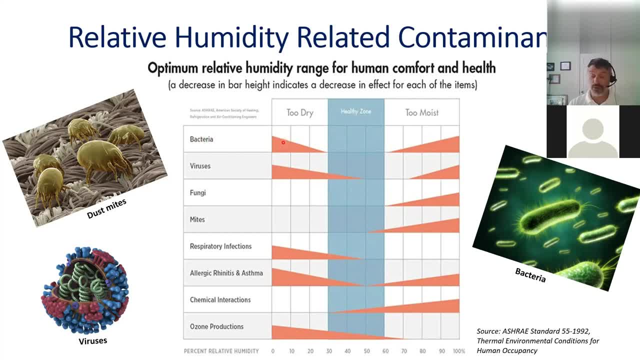 shows is like for bacteria, which we do uh quite a few of uh bacteria assessments- um, the higher the the tear, i'm sorry, the uh, the higher the bar, the higher the the activity for those contaminants. so bacteria can thrive in relative, in really low um uh humidity, as well as really. 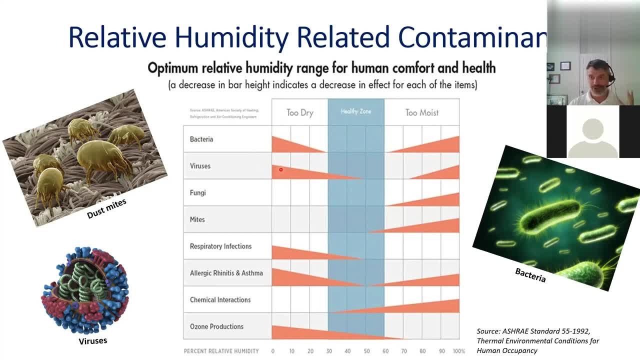 high humidity viruses, and i'm sure we're all virused out, but viruses certainly can thrive um when it is really extremely dry and when humidity is really starting to get 80, 90, 100 percent humidity. yes, there is some viral activity um between 30 and. 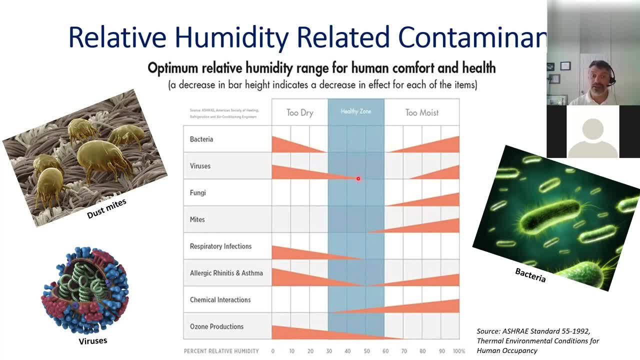 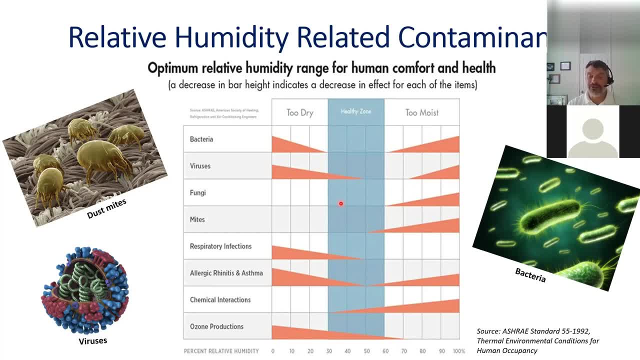 dry fungi molds are not really uh affected. but once we start getting humidity, uh starting to get above 60 percent, and especially, you know, the 70, 80, 90 percent range, that is really conducive uh for fungal activity, uh, mold activity, dust mite activity as well, um around 50 percent we start. 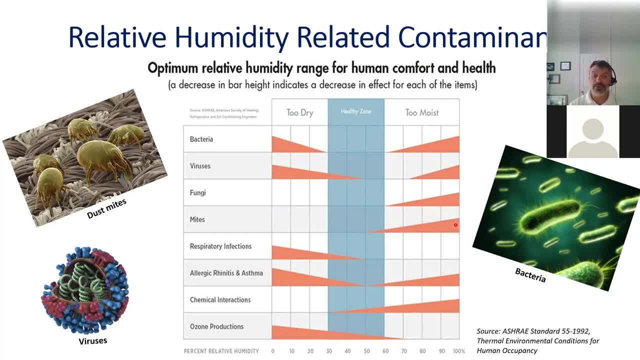 seeing an increase of dust mites and then again once it gets more humid, and then i'll briefly go through the the bottom ones. but respiratory infections can start when it's too dry, mostly because your mucus membranes are not are drying out, so you're not uh, your body's not able to expel as much of the the other uh, particulates and and stuff that. 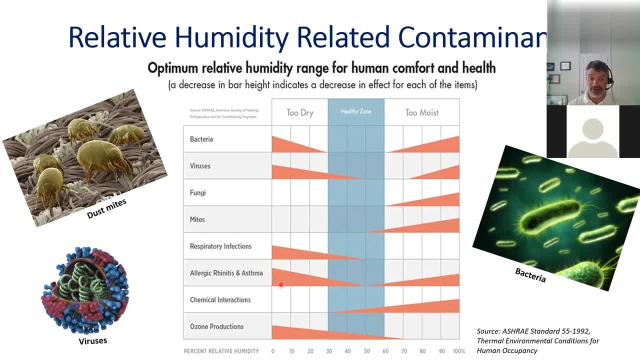 we're breathing in um and the uh. allergic and asthma, allergic rhinitis and asthma- again, the least amount of activities during the in that 30 to 60 percent range. so again that 30 per 60 relative humidity percent range, that that's optimal move on. 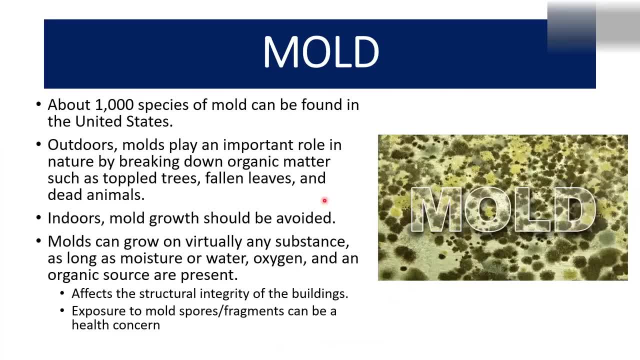 jump rating into mold. so mold- right now there's there's about a thousand species of known mold. uh, in the united states there's roughly about a hundred thousand known species worldwide. um, in outdoors, mold plays a real important role. we would not be alive without mold, let's just put it that way. uh, so, but they are, um, they break down matter. uh, fallen leaves dead. 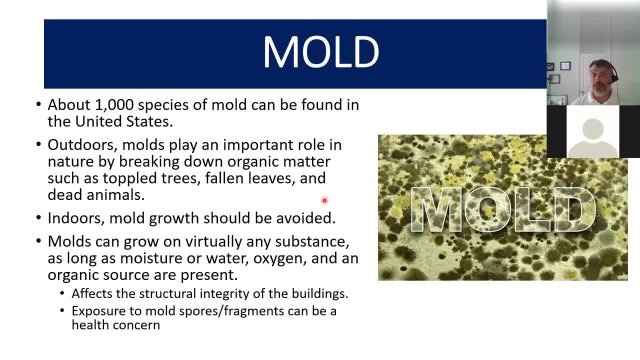 animals, toppled trees, uh, molds are very important too for, uh, for many food production. um, we wouldn't have some cheeses, we wouldn't have some cheese, we wouldn't have some cheese, we wouldn't have some food production. um, we wouldn't have some cheese, we wouldn't have some cheese, we wouldn't have some. 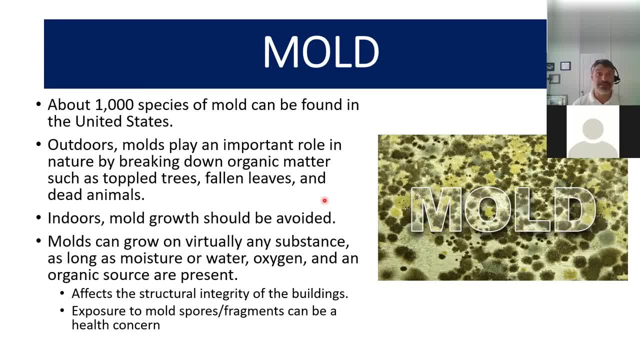 or um some certain medicines, penicillin- is derived from a species of mold, so there are some good things about mold, but we definitely want to avoid mold growth indoors. uh, and molds can grow on virtually any substance as long as there's moisture. moisture or water, uh, oxygen and an 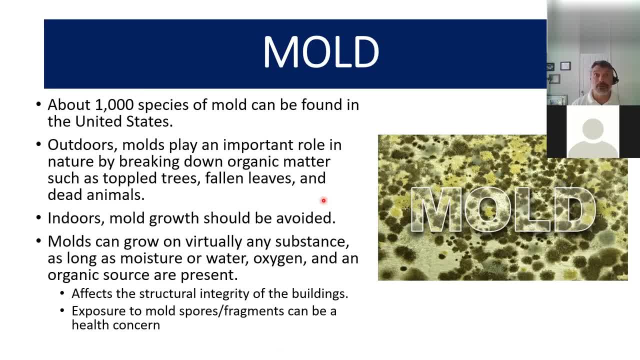 organic source, basically anything that has that's got a carbon compound. molds can feed on on that. mold prefer damp or wet building materials, such as damp drywall, wood, uh, high, high cellulose materials. um. so not only our molds, uh, can't affect our health, but they're also affecting the structural 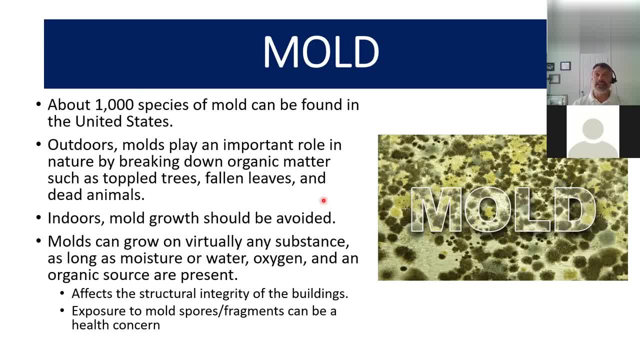 integrity of buildings. just as, just like molds are breaking down the organic matter outdoors, that's what they're doing to the building materials inside of our structures, if it's left unchecked. so molds are eating away at the drywall. at the drywall, and they're eating away at the 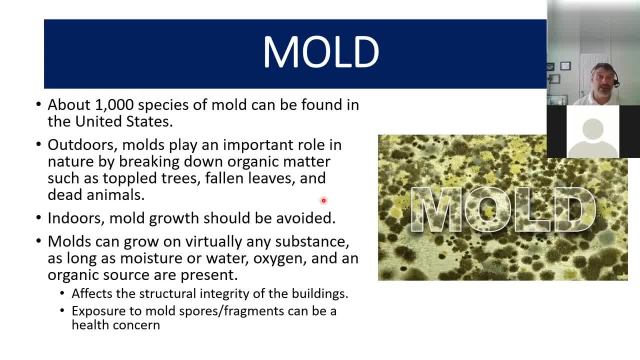 wood. so if you ever see wood rot, well, a lot of that wood rot is because of mold or fungal activity that's eating away at the sugars uh inside the wood. so so again, not only is it important for health purposes, but it's also important for uh to identify any mold issues. mold and moisture issues due to structural integrity of buildings. so mold exposure, mold exposures: about 50 percent of all homes have mold and, whether it's visible or not, on the wall or inside, so there's likely to be some sort of mold in about 50 percent of all homes. uh, 93 percent of chronic sinus infections can be attributed to. 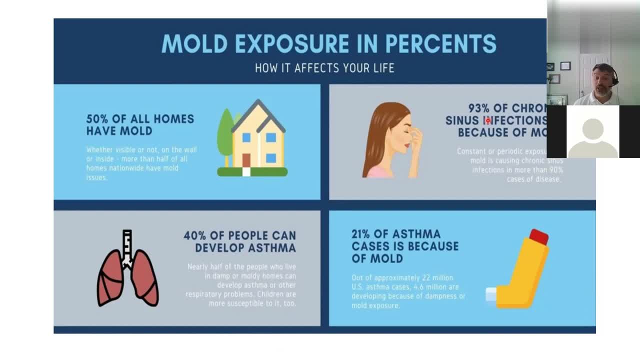 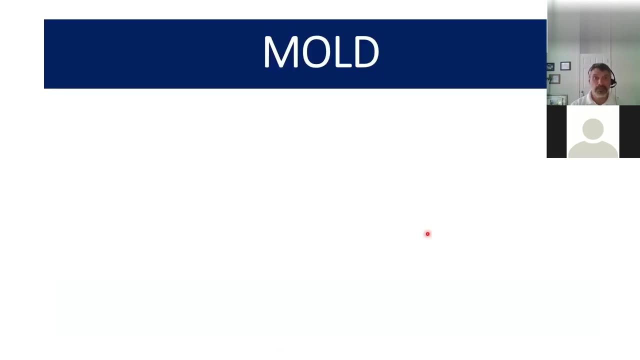 mold exposures, uh. 40 percent of people can develop asthma, uh as a relation, as a as it relates to mold exposures. and then again, 21 percent of all asthma cases is directly related to uh, to mold. so here's some just examples of molds and uh mold growth. again, as i stated before, molds need water. 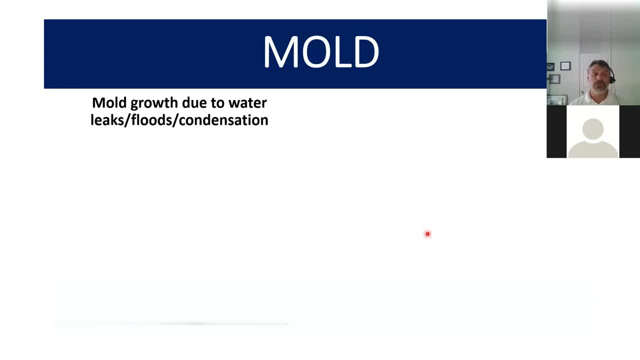 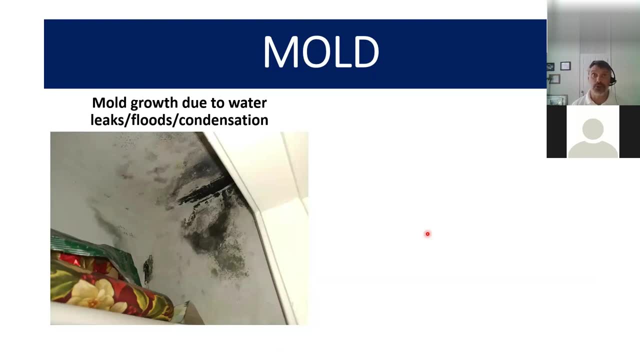 indoors to grow some sort of moisture source. so mold growth due to water intrusion, floods, leaks, plumbing, uh plumbing issues, condensation from metal duct work or or from plumbing. this is what this picture is, typically what we we find it. you get all sorts of molds that grow on drywall. 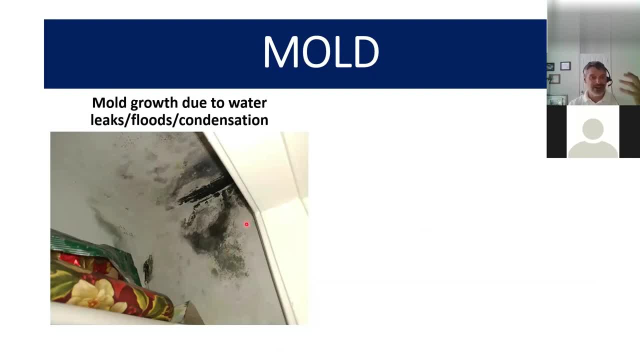 this is a picture that i took from a picture that i took from a picture that i took from a picture from from one site where there was just a chronic water intrusion from. this is in a basement level closet and water was coming in from the exterior wall running in and just causing all this. 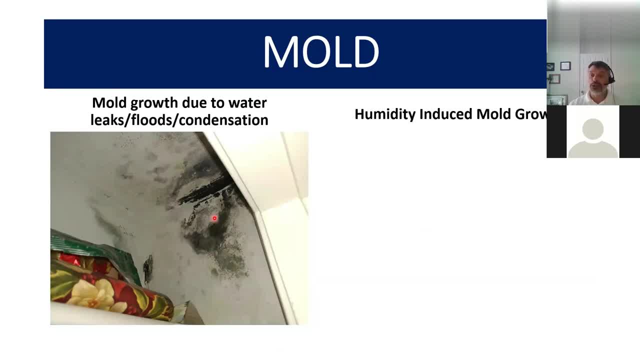 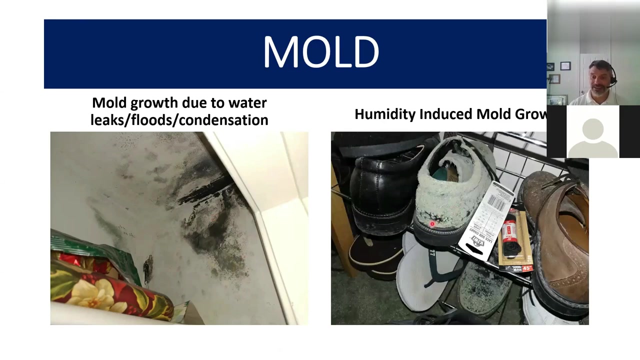 nastiness. then we also have what's known as humidity induced mold growth. so mold growth can grow. certain species of aspergillus penicillium can grow and survive. they're very dry tolerant. so when humidity levels are maintained roughly at about 60 to 70 percent indoors, we could end up with this. this is a very common and i see this. i did. 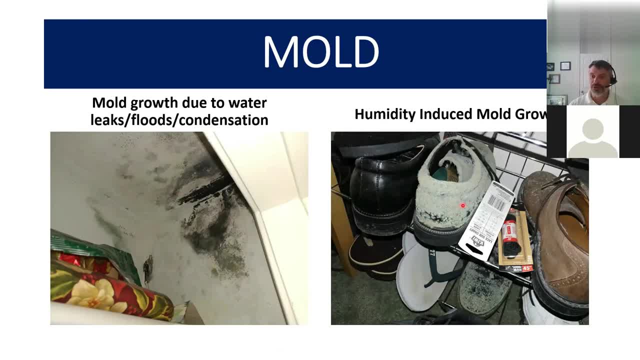 take this picture of a home where you get some mold growth: on shoes, on clothing, on furniture, underneath stairs, so anywhere where there's air stagnation, humidity, so you don't always need a leak or flood to have mold growth. and again, these molds are very common in. 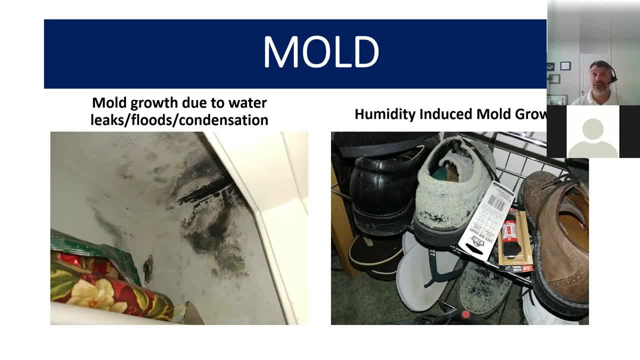 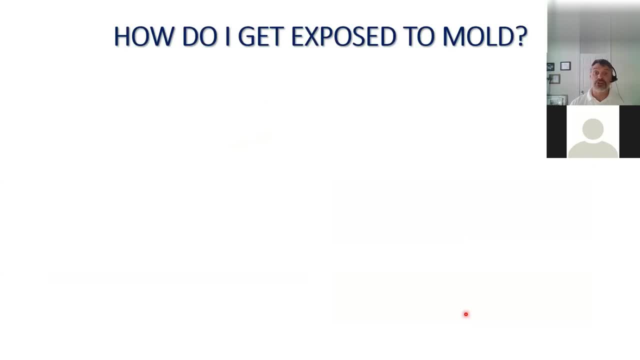 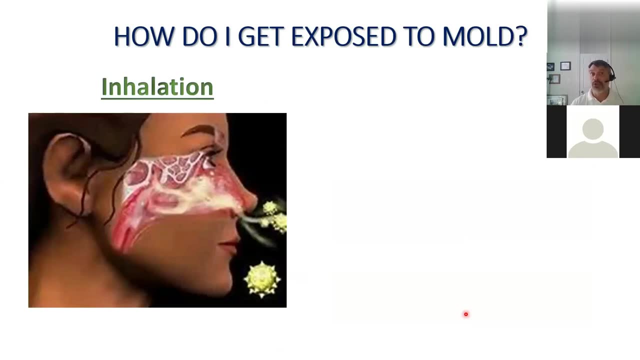 humidity induced, but they can make cause some serious health issues, especially dealing with species of aspergillus and penicillium. so how does how does one get exposed to mold? inhalation is the most common route of exposure. obviously we're breathing in mold spores. we're breathing in mold spores every day. 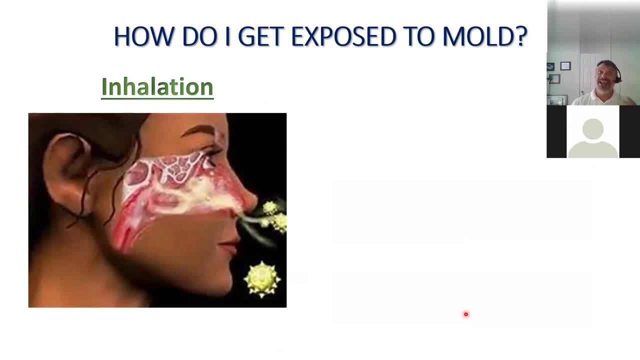 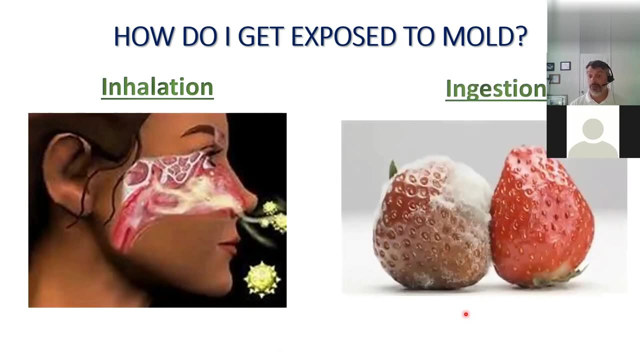 but what you don't want to do and try to avoid is to breathe in higher on high concentrations over extended periods of time. so inhalation of spores and mold fragments- meaning the hyphal elements is what were- is one route of exposure and the other main route of. 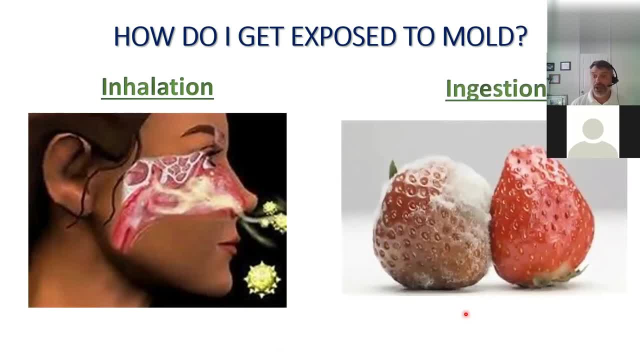 exposure is eating, eating foods that have mold and ingesting foods that have mold, and it's not always fruit. i mean you could have cereal grains that have mold, where you may not actually see mold, but if, if cereals or oats or things of that nature being stored in somewhat more of a damp environment. 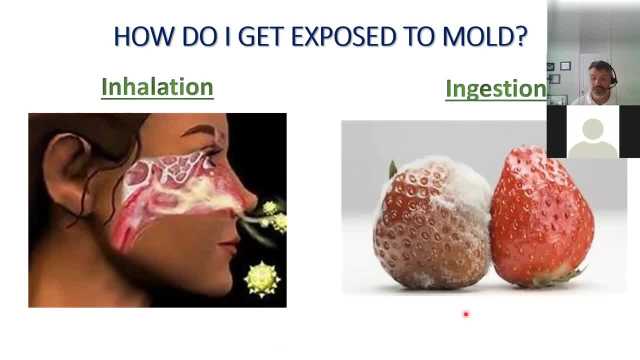 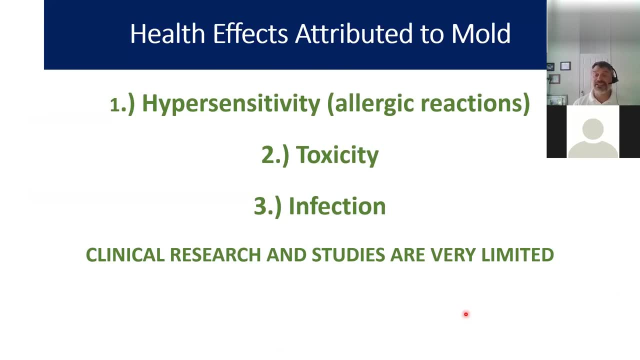 and not a really dry environment, you're going to get some molds that can develop on those foods. so the health effects attributed to mold: uh, we've got hypersensitivity, which is basically your allergic type reactions, toxicity and infections. um, clinical research is still relatively limited and studies are very limited as far as the health effects attributed mold, and there are some. 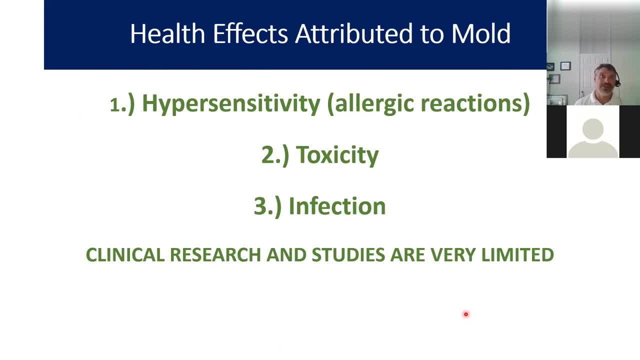 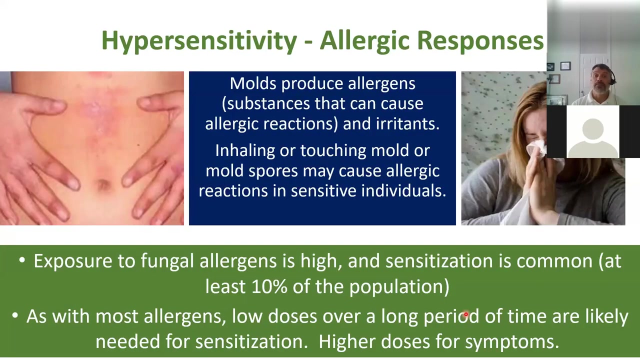 controversies with major organism organizations that say: well, the, how do we quantify? or what do we say? you know the and are there enough studies, clinical studies or epidemiology studies that could definitively link certain molds to certain, uh, certain health effects? so again, that's why clinical research and studies are still very, very limited. but we do know that 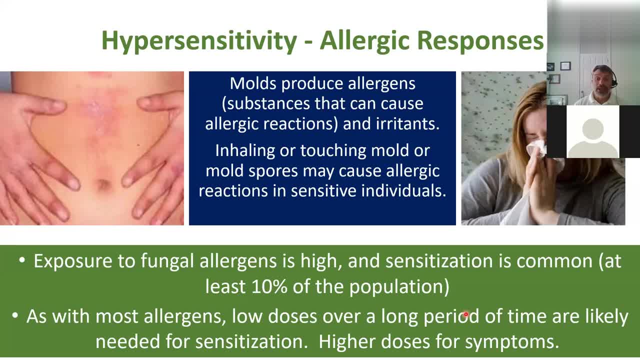 molds can cause some allergic responses um, and they could be from either inhalation or touching molds or eating molds uh can cause allergic allergic reactions in sensitive individuals. exposure to molds uh in sensitive. the sensitive population is roughly about 10 of people who are known to have mold allergies, but with most 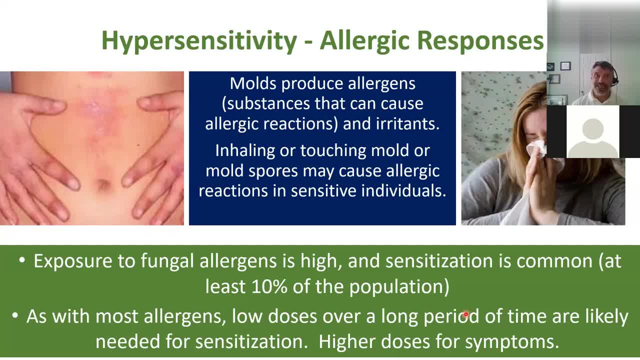 allergens. low doses over long periods of time are likely needed for someone to become sensitized or to develop an allergy to molds, and then higher doses once you become sensitized. higher doses are likely for- uh, for symptoms. again, i'm using the terms likely, uh, um, probably because there is 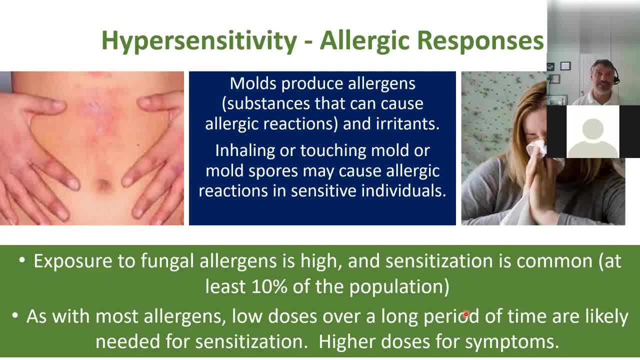 no definitive answer to that question, so i'm going to go ahead and i'm going to go ahead and answer. there are no definitive answers. it's all based on someone's individual sensitivities, their own genetic dispositions, uh. so i'm going to use some generally, uh, general terms that are that we 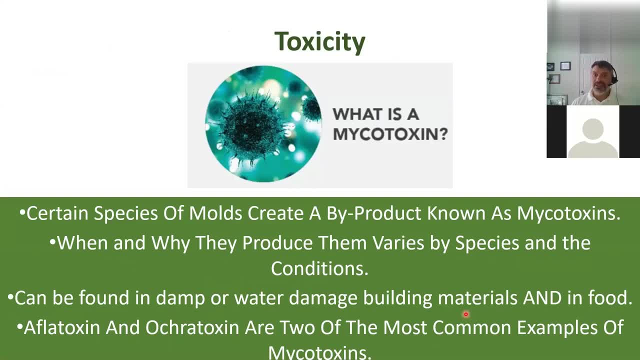 use in the industry, mold toxicity and i'm sure many of you have heard about mold mycotoxins. so what are mycotoxins? uh, certain species- molds- do do create uh bright byproducts of mycotoxins, so they're basically chemicals that are released by the molds and why we. 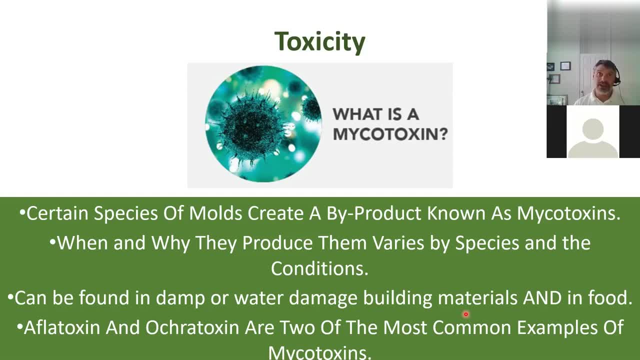 think. what's what we think? why molds produce these toxins are to help fight off other invading species of molds. so there's again, as i said, there's thousands of species of molds and they're all competing for the same food sources. so a lot of these molds produce these mycotoxins to help. 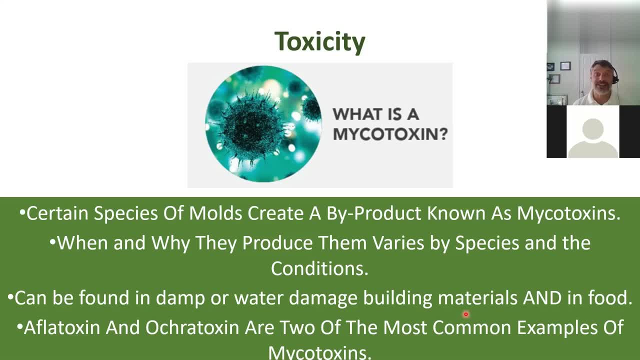 fight off other invading species so that they, so that they, uh, they win out, they, they're on the food sources, uh, and these mold mycotoxins again can be found in damper water and in the water, damaged building materials and food, uh. so again, it's not always mold growth that where you could. 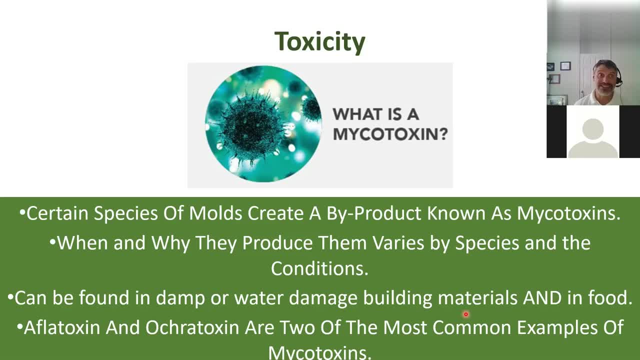 be exposed to and have mycotoxins in your system, as relate uh due to molds on on building materials, but also in foods. excuse me, the most common examples of mycotoxins are aflatoxin and ochre toxins, but there are a lot of other mycotoxins on that that are common in the 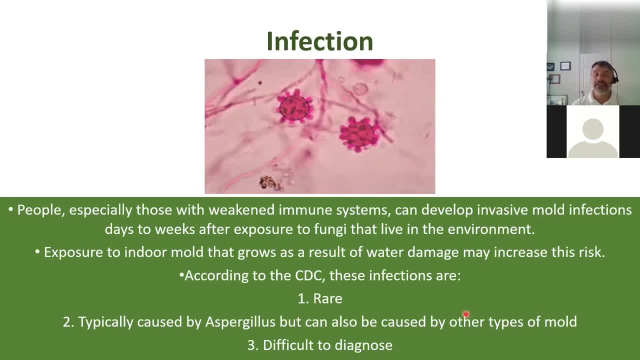 world that are commonly associated with molds, and i'm going to stop just for a quick second and just so everyone who's here knows: at the end i will be answering any questions that you may have, so we're going to hold off on questions until the end. uh, there is a group chat. there's a chat. 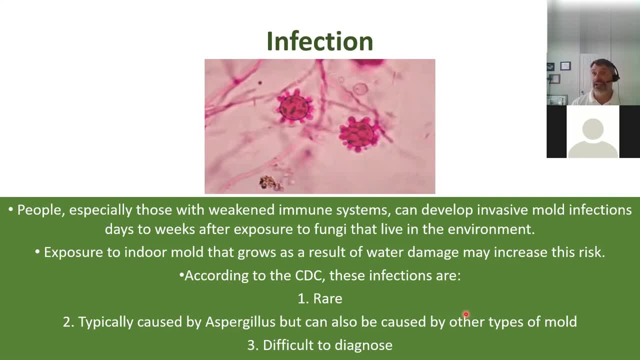 function. so if you want to type in a question, i'll address any questions that i can at the end, at the end of the presentation. just want to get that in there. so if anyone thinks that i'm going too fast or has a question, we will address any questions. 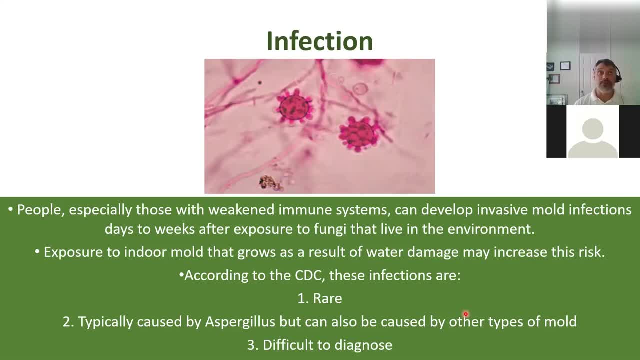 at the end. uh, going back to uh molds and health effects, so another one. in molds can uh there can be fungal infections or mold infections. um, those are especially with weakened immune systems. uh can develop an invasive mold infection either days to weeks after exposure. uh, if they're living in that. 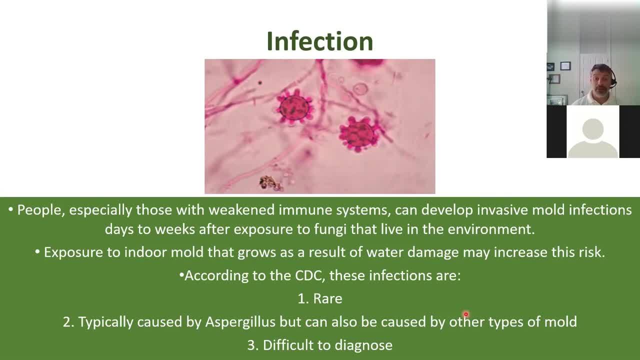 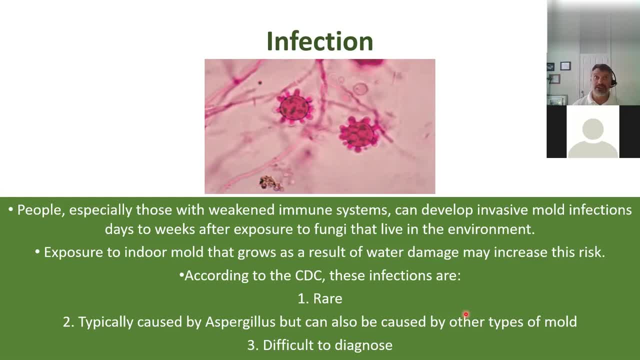 Aspergillus and there are other opportunistic fungal pathogens, but Aspergillus is typically the most common genre mold and there are certain species within Aspergillus that are more associated with infections, but mold infections are difficult to diagnose. 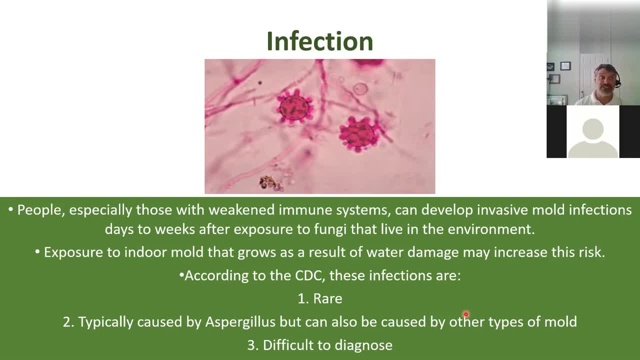 Um, jumping back to Aspergillus, there is an actual specific uh infection directly related to Aspergillus, called Aspergillosis, and that's where the uh Aspergillus can actually grow inside of the lungs. Um, so I know in hospital settings, um, we've been called in or I've been. 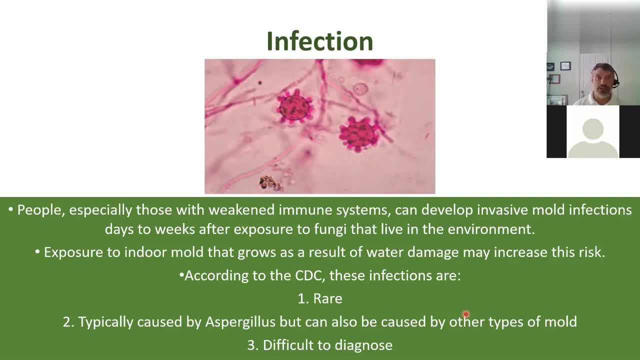 called in to do mold mold inspections into our quality testing and they really want to know what species of Aspergillus may be present. um, in certain, in certain areas. Uh, so, uh, um, but again, infections related to molds are rare. 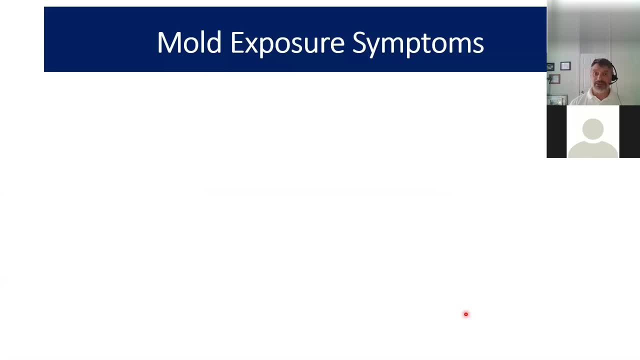 but here are some symptoms, uh, and I'm going to talk about some mold exposure symptoms, but first things first. I'm not a doctor and I don't play one on TV, So if anyone has any symptoms that are that were about to grow up, it may or may not be related to molds- best to consult with. 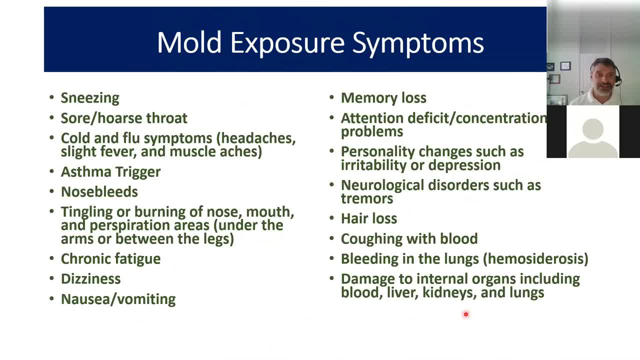 your healthcare practitioner. Um, but these are very common, or most common, symptoms related to mold exposures, And many of you may, may, uh, see a recurring theme here but sneezing, a sore throat, a sore or hoarse throat, cold and flu. 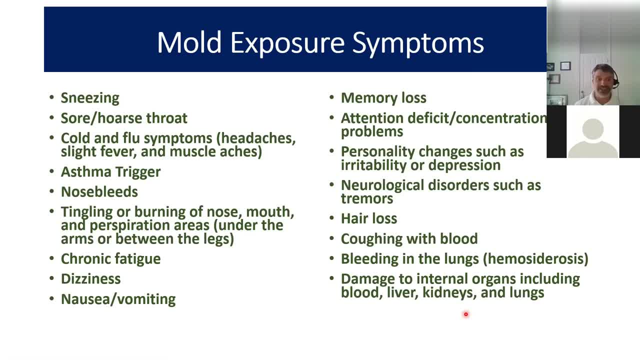 symptoms: asthma, nosebleeds, chronic fatigue, And I'm going to jump through some of these, and some of these you may not be even be aware of, but, uh, some of these symptoms have been linked to mold exposures, memory loss, attention deficit and concentration problems. personality: 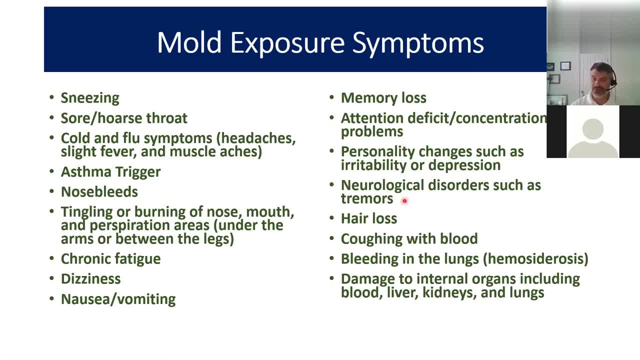 changes, other nausea, Neurological disorder or next orders uh hair loss. I've had clients who have had uh chronic hair loss problems directly related to molds and mold exposures. Um, and those and some of the others uh here are symptoms that are known related exposures uh to mold. So I'm going to 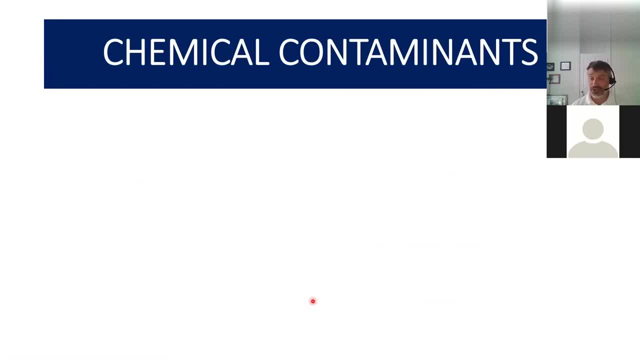 end there on mold, And again I can't address any mold issues, Um, um. so I'm going to get into, uh, the chemical contaminants now as it relates to indoor air quality. So what we'll be talking about specifically are carbon monoxide, uh, or. 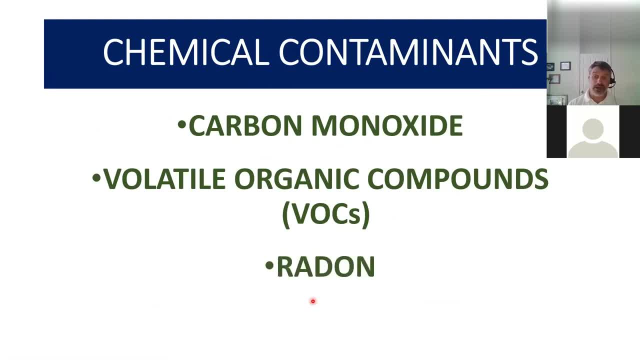 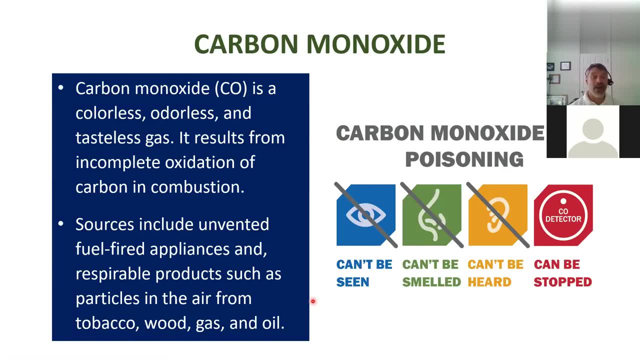 carbon monoxide, volatile organic compounds and radon: Uh. so for carbon monoxide, uh, carbon monoxide is a colorless and odorless taste of gas. Um, and I'm sure many of you- I hope all of you- have at least carbon monoxide detectors in your home, especially if you have any um um gas. 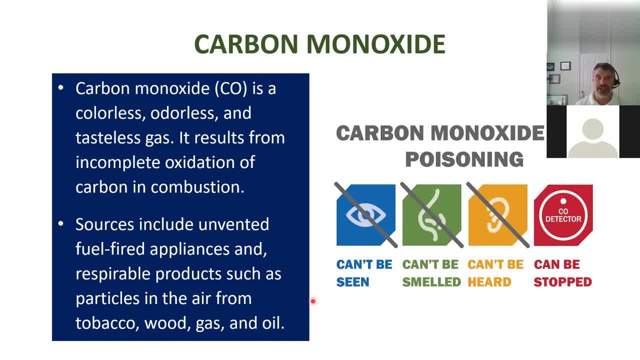 fired or or fueled uh furnaces or homes. Hot water tanks um you should have carbon monoxide um, and sources include unvented fuel. fired appliances uh um and then other uh tobacco, wood burning uh gas, gas uh powered. 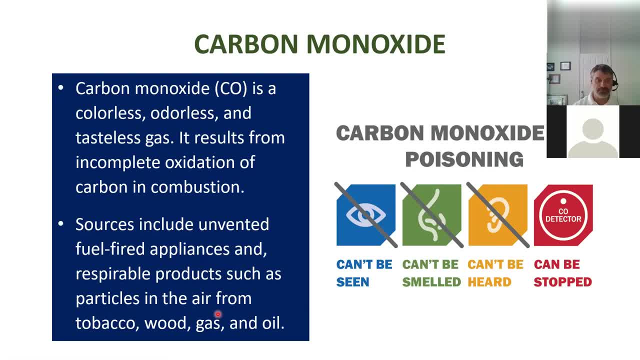 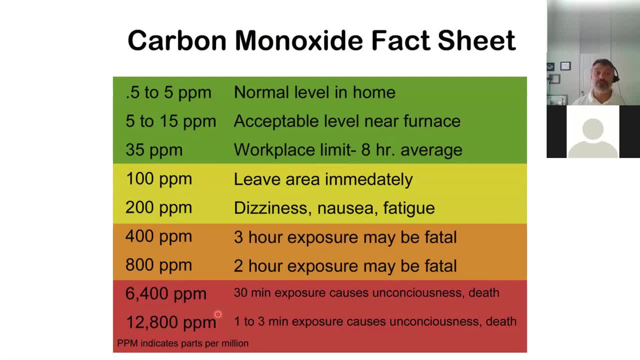 uh uh equipment and oils. So for carbon monoxide, uh, what are typical levels in a home? We could find them anywhere between 0.5 to five uh parts per million. Generally, it's expected and acceptable, if you will, in a properly functioning uh gas fireplace or. 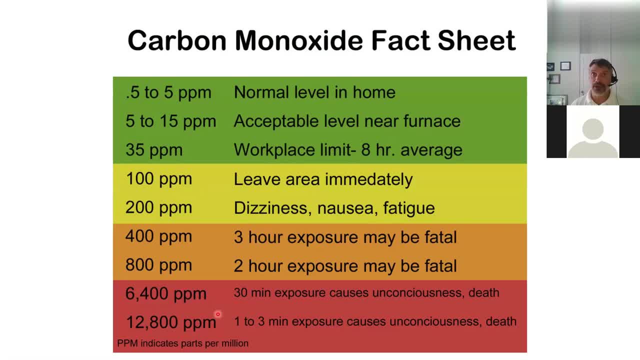 furnace or or even um uh gas fueled um uh appliances to have carbon monoxide levels at about five to 15 parts per million. There are workplace limits uh at 35 parts per million over an eight hour time weighted average. But where we start to see is if, if uh carbon monoxide levels are. 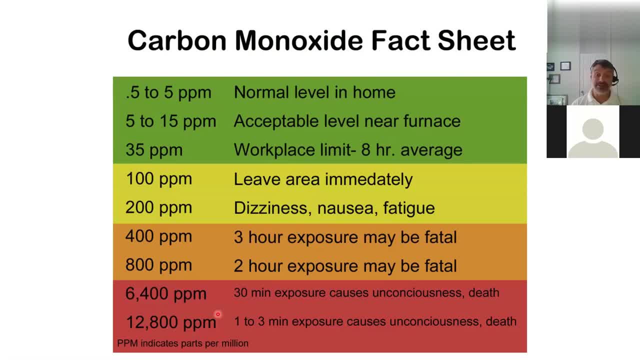 about a hundred parts per parts per million leave the area in ease Immediately. dizziness uh, nausea and fatigue are some of the most uh the initial symptoms of carbon monoxide poisoning, And that's where you when levels are at about 200 parts per million. 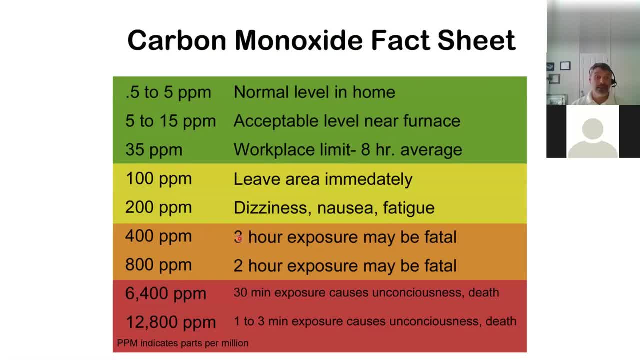 And then, as you can see, the higher up we go, uh it. carbon monoxide poisoning can be fatal and relatively quickly. Um so, again, as I get into the what we could do to improve it, one of the things is to definitely get carbon monoxide. 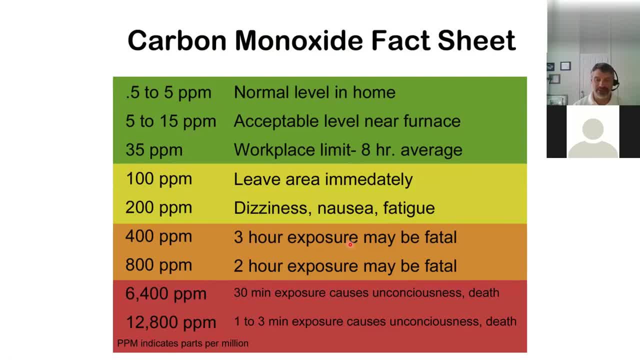 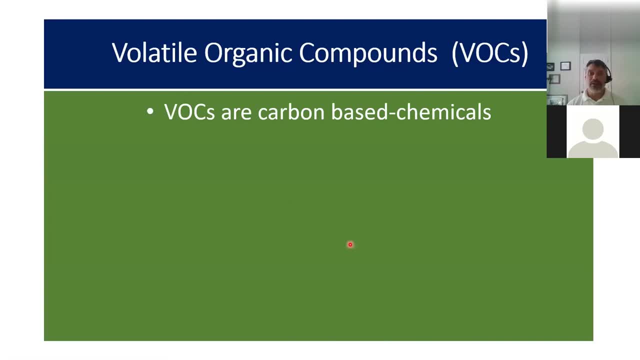 especially if you're using any gas, uh, gas appliances. We're going to go into volatile organic compounds. So volatile organic compounds are all carbon-based chemicals, Uh, there are thousands of VOCs. they're naturally occurring or synthetic, uh, and they're typically higher indoors than outdoors, And for a couple of reasons. 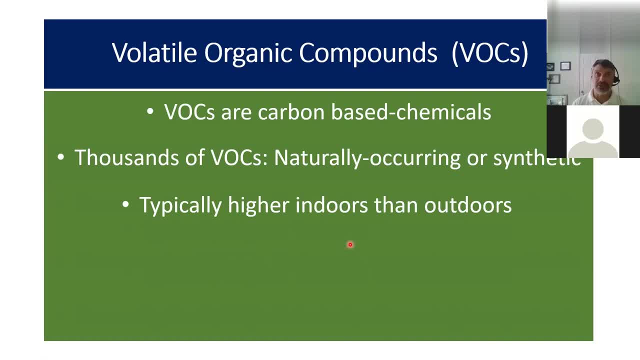 obviously we've got VOC sources and I'll get into the sources indoors. but why we? not only, uh, because outdoors, uh, we've got a lot of VOC sources, and I'll get into the sources. indoors there's a lot more air, but as far as concentration goes, but also because they're 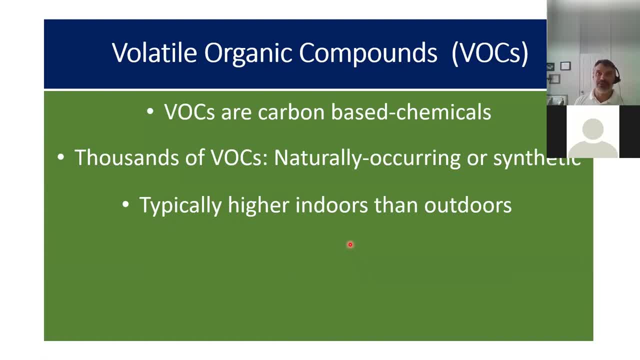 carbon-based uh UV helps break down those carbon uh binders in the chemicals. So once it's out, once VOCs are out in sunlight, those, those VOCs, or those chemicals uh break apart, if you will. Some volatile organic compounds are highly toxic. Others can be moderately toxic. 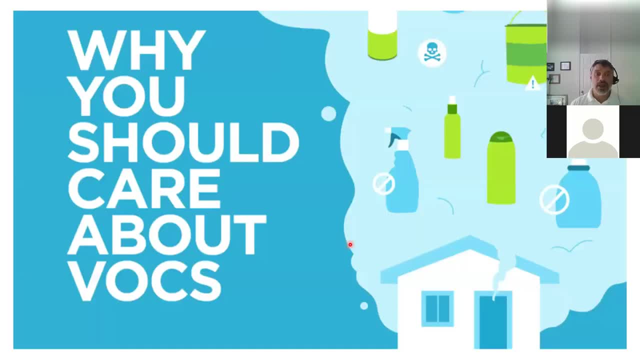 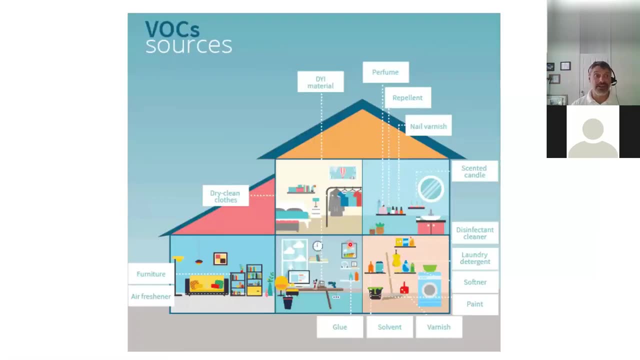 and then some are just mildly toxic. Uh, so why? why should you care about VOCs? Well, VOCs in homes, there's many sources. Uh, we've got paints and paint strippers and other solvents. We've got, uh, um, some clean and I'm not sure. 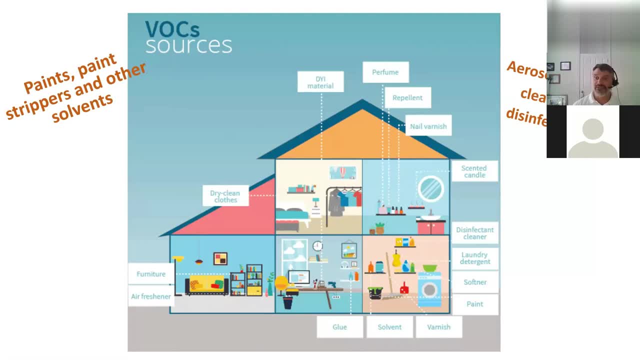 if I can move this at all. Uh aerosol sprays, cleaners, disinfectants um detergents, air fresheners, perfumes, scented candles, potpourris, hand sanitizers- They all emit uh volatile organic compounds. 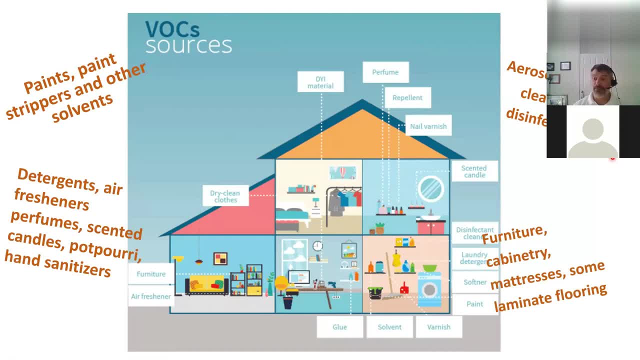 Uh, furnitures, uh, cabinetry mattresses, some laminate flooring products, So building materials that are installed or or furnitures that you buy, those all emit or can emit some volatile organic compounds. Um, we often get called in, uh, with complaints after a remodel. 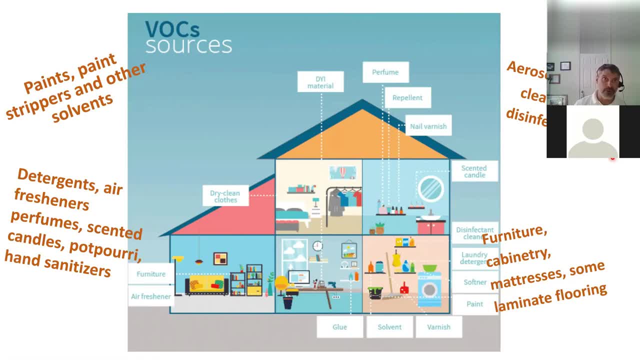 in a home, furniture has been installed or, uh, new flooring or cabinetry has been installed, And some of the occupants, when they come in, uh, especially if they're if the house has been sealed up for a while- start complaining. oh, I'm getting these. 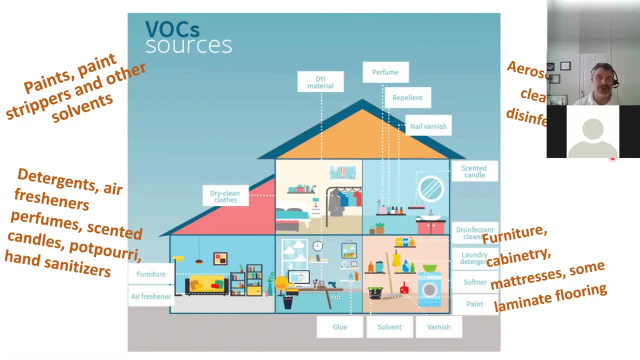 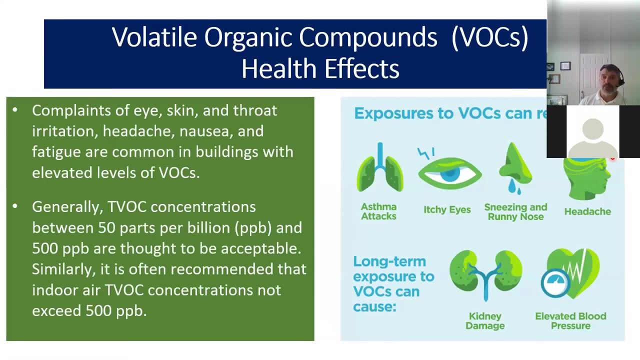 these odors or I'm getting headaches And I don't know if it's because of the furniture or carpeting or whatever the case may be. So that's not uncommon, an uncommon complaint that we get called into to help investigate, uh, those issues. So the health effects related to carbon, uh. 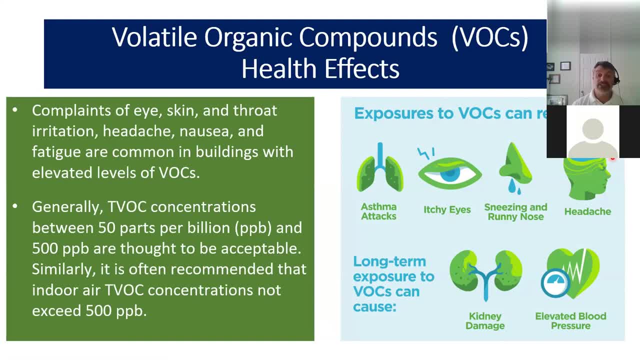 I'm sorry- to volatile organic compounds. um again, asthma attacks, itchy eyes, running nose, headaches- noticing a theme here With some of them, both with molds and with VOCs. um, but again, uh, irritation. 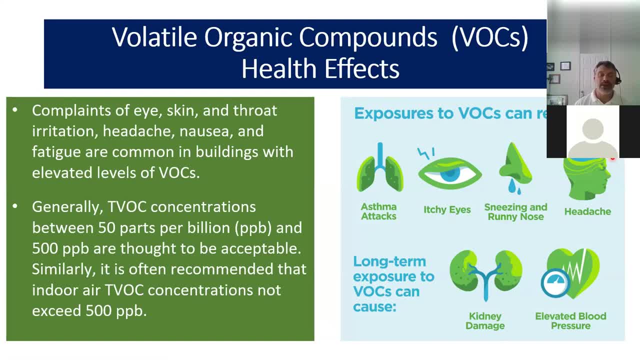 throat irritation, headaches, fatigue are just common- uh common- complaints that we receive that may be a result of volatile organic compounds. in a typical indoor environment It's not uncommon. It's generally found to be acceptable where VOC- total volatile organic compounds are generally in between the 50 parts per billion range. 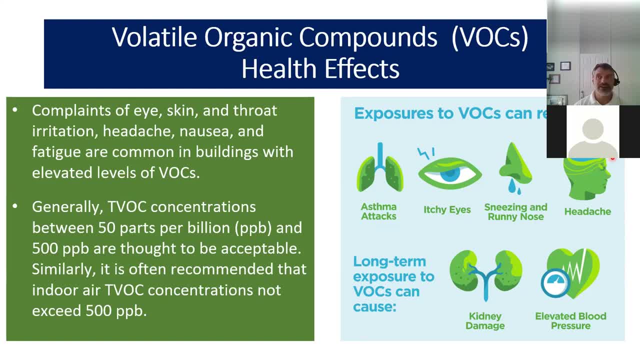 And 500 parts per billion range. Once we start again seeing levels above that- 500 parts per billion- as a total volatile organic compound level, that's where some red flags start to start to pop up. Um, uh, when we're doing an investigation. uh, long-term exposures to VOCs. 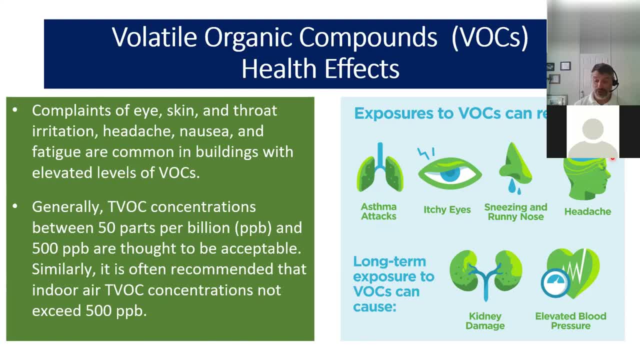 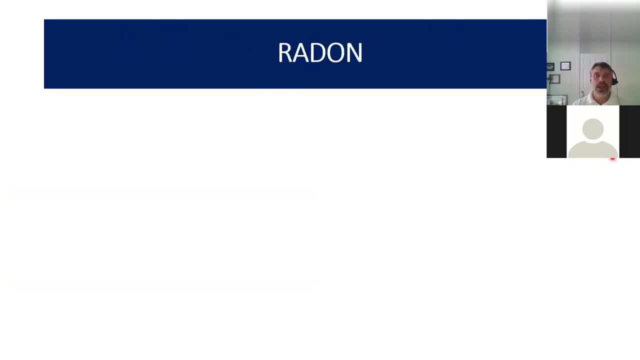 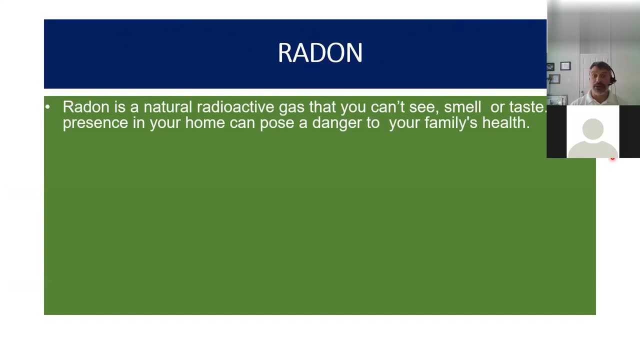 uh to volatile organic compounds. And we're going to move on over to radon now. Um, radon is a naturally occurring gas that you can't see, smell or taste. Uh, its presence is in your home and it certainly can pose a a a danger. And radon is formed by natural, natural radioactive. 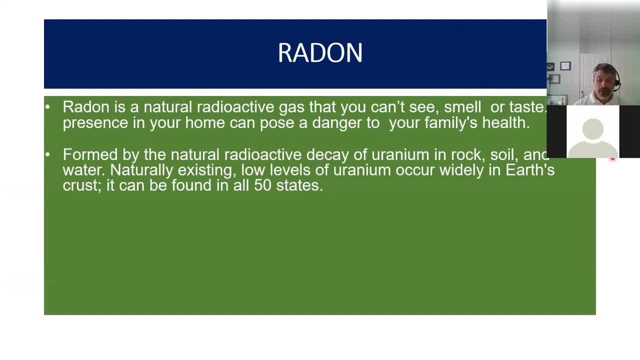 decay of uranium in rocks in the earth's crust, Um and it is found in all 50 states, Um. radon is the same as radon. It's the same as radon. It's the same as radon. It's the same as radon. 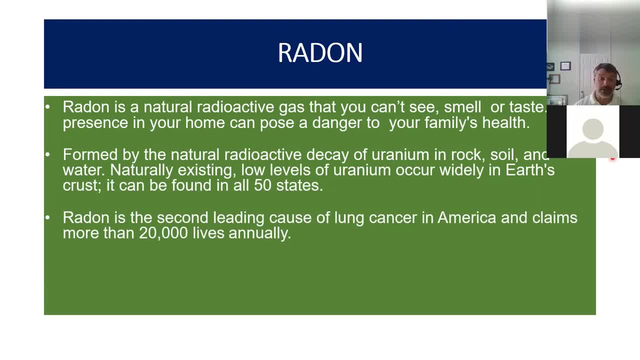 Uh, radon is the second leading cause of lung cancer in America and radon- uh related lung cancer, excuse me, uh- does claim more than 20,000 lives annually. Uh, radon is the leading cause of lung cancer among non-smokers. So, and that is a national stat that is a leading cause. 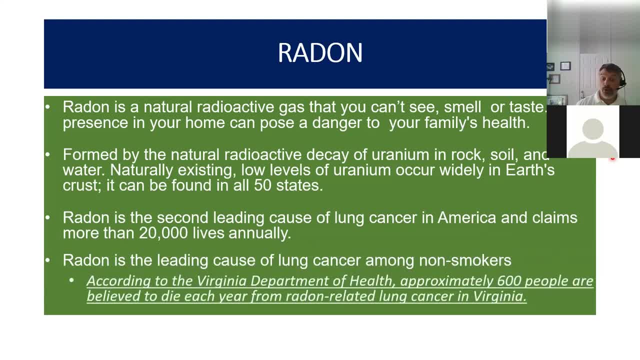 of lung cancer among non-smokers And, according to the Virginia department of health, approximately 600 people every year are believed to have died from radon related lung cancer. And that's a in Virginia And I'll just pop up a map here. Uh, this map is courtesy of the US EPA. 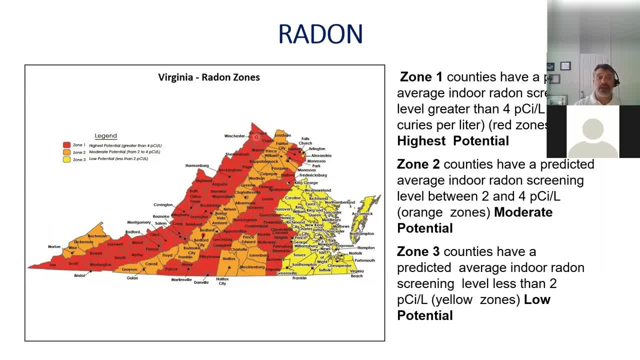 and it gives zones of the highest potential for uh, for, uh, uh, for what EPA says is the screen level of four picocuries per liter or higher. Uh, so, as you can see, we're- most of us are- in. 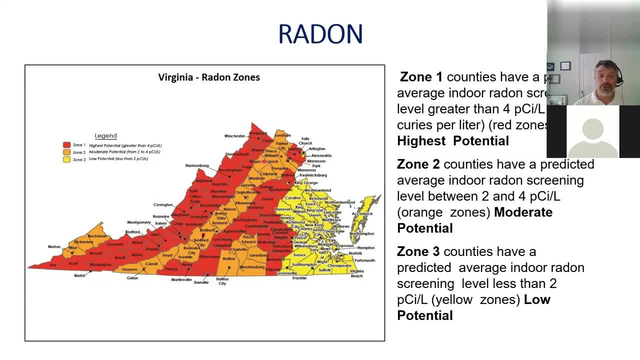 the Winchester and the Northern Virginia area. We're all in the red to red to orange zone Um which again, our counties that are known uh to have uh, relatively uh uh, there's a high potential or moderate potential for uh for radon to exceed the EPA's guidance levels of four. 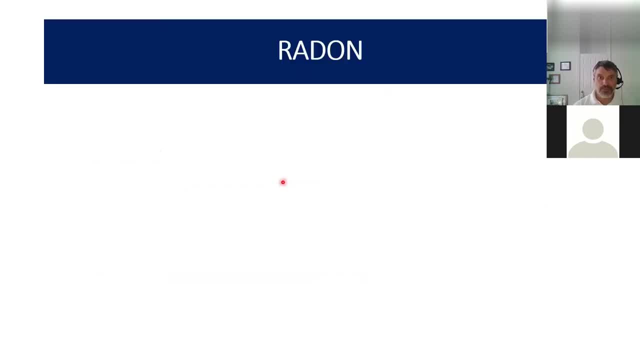 picocuries per liter. So why again? why is radon a concern? radon decay product uh. radon decays into radioactive particles known as radon decays. So radon decays into radioactive particles known as radon decays. So radon decays into radioactive particles known as radon decays. So radon decays. 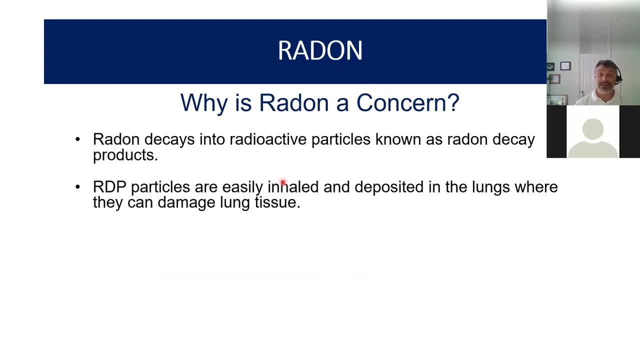 products. uh, these particles are easily inhaled and deposited into lungs, So it's not the, it's really not the gas radon, if you will. that that we're that we're concerned about And that's what we measure And if, if radon is tested for, it's measuring radon levels, but it's really the. 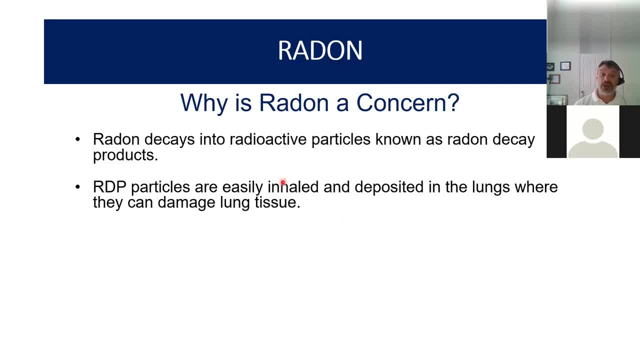 decay products uh that are inhaled and those lungs or those decay products damage the lung tissue. Uh, so the radon uh decay products decay into uh plutonium 218 and plutonium 214, and they emit alpha particles And 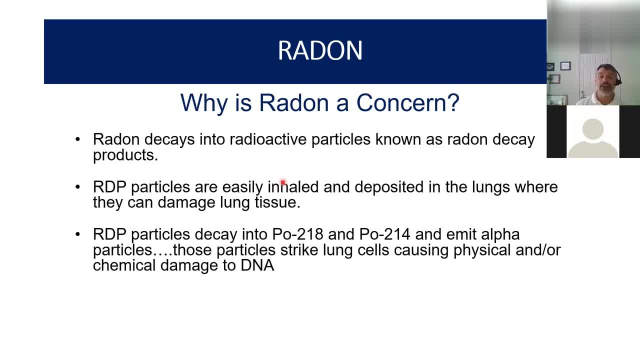 those particles are just constantly striking the lungs and they cause physical and chemical and physical damage to the lungs and can actually cause damage, uh, chemical damage, changing the DNA, Uh. so that's why radon is definitely a concern, especially in this region. 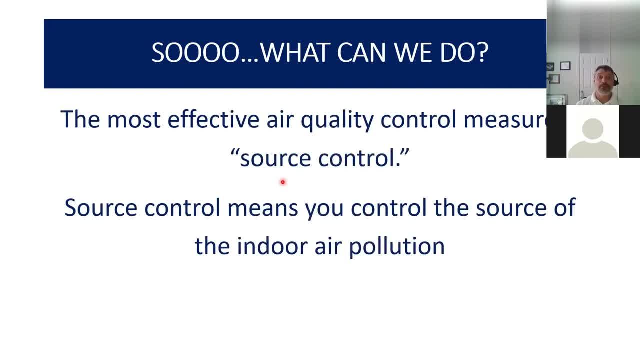 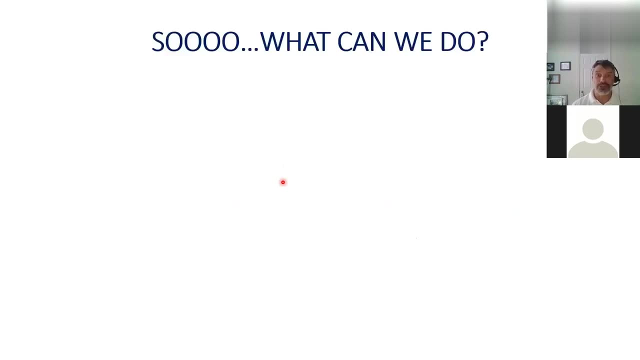 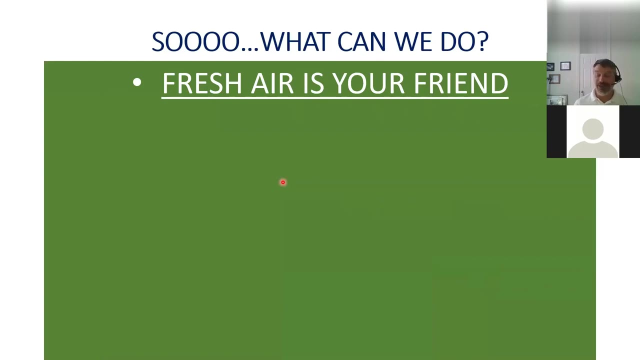 So what can we do? Well, the most effective air quality control measure is source control. We have a lot of control as to what we're being exposed to, Um, so you are in control as much as much of the indoor air quality pollution. First thing that I always tell: fresh air is your friend on days where it's clement. 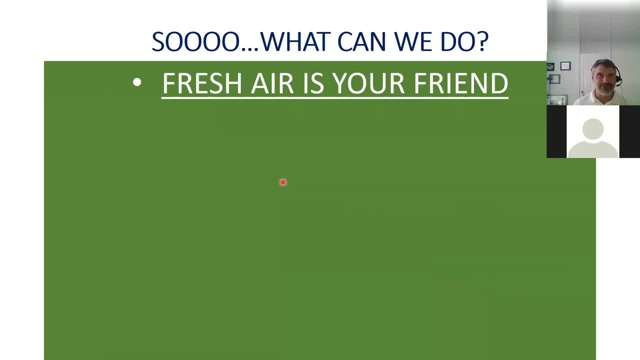 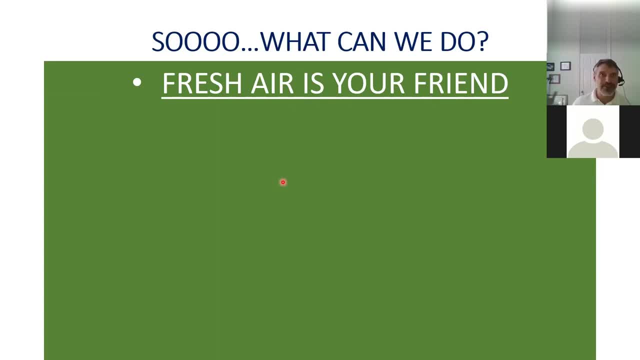 it also allows just common particles and stuff that has built up to to exhaust out. You're getting cross breezes, You're getting a ventilation of of the structure of your home. So fresh air is your friend, correct? all uncontrolled sources of moisture? Uh, so what that means is, if there, 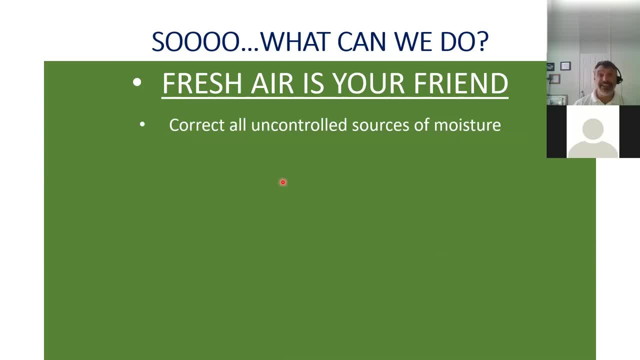 are any plumbing leaks or if you're having water leaking in your basement. even if it's an, even if it's occasional, uh dampness in your basement, it's coming from somewhere. So you have to really identify to correct. 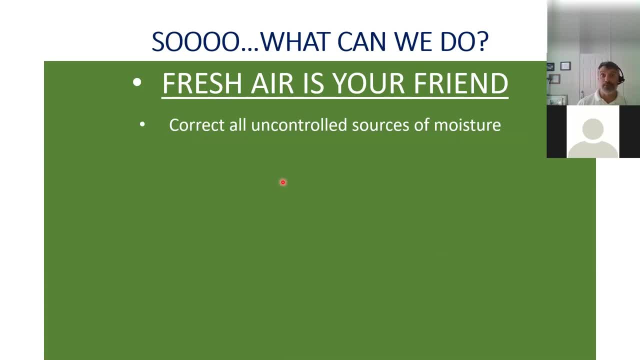 To not only prevent damage to the structure but also prevent- help prevent mold growth. um maintain humidity levels. again, between that 30 per 60% range is recommended. Ideal is at about 50% or below at all times If you're going away on vacation or taking a two week vacation or a. 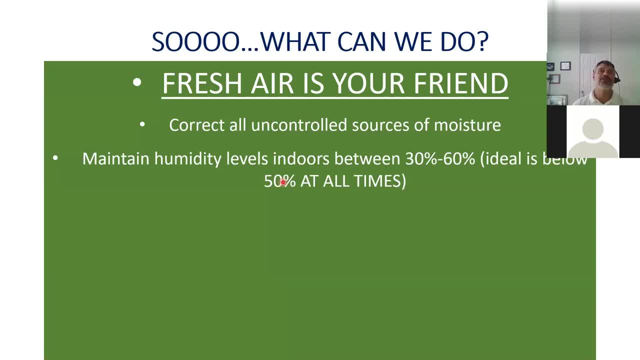 three week vacation, especially in the summertime. don't shut off your air conditioning, let it run. Um, I've been involved in way too many uh projects where people have gone away on vacation- summer vacation- for two weeks or three weeks, and they shut off their air conditioning and they come home and lo and. 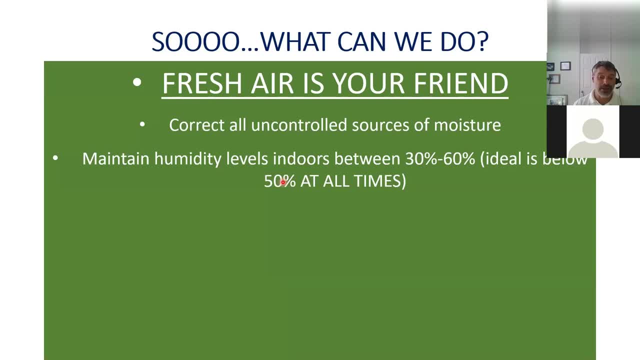 behold, there is mold growth everywhere throughout their house because they didn't keep their air conditioning running the humidity inside their home. We're in Northern Virginia. It gets humid here, It gets warm here. You've gotten new food sources in your home- Perfect environment for. 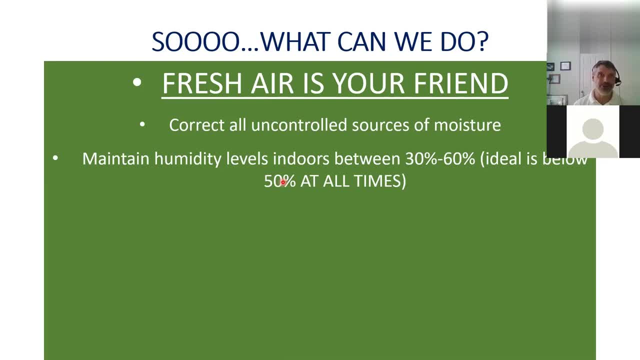 mold to grow when it's warm, humid, no air movement And you get uh. so please, if you're going away or um um, uh, keep that humidity uh at, or below 50% at all times. maintain good housekeeping. get into those hidden dust reservoirs, uh move. 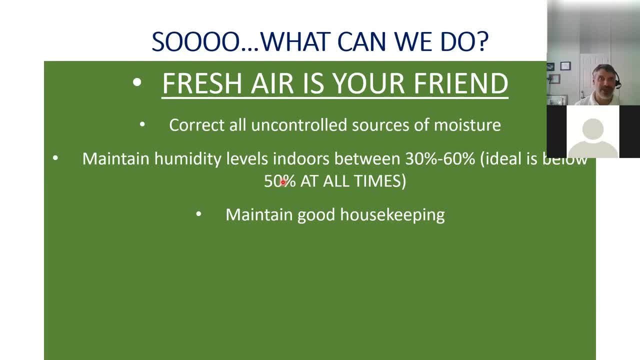 occasionally move your refrigerator, move your stoves out, vacuum up all that dust and junk, that that kind of gets hidden. but maintaining good housekeeping is really a major function of of of keeping uh, of improving your air Quality, making sure your exhaust vents, your dryer vents, your bathroom vents, your kitchen. 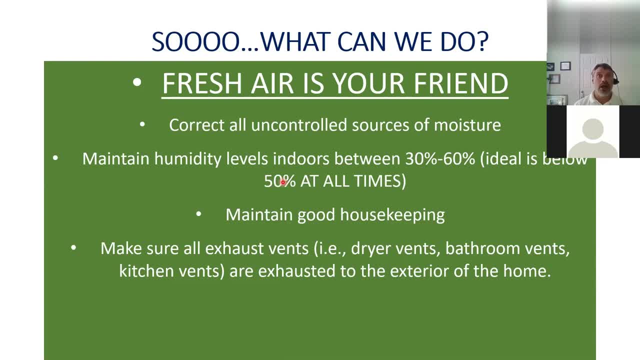 vents are all exhausted to the exterior. Um, and a lot of times they can be your uh, especially dryer vents. uh cause dryers do vibrate and they can disconnect. when dryers are running there, They're trying to exhaust out all that water, if you will. So it's just hot, moist air. So if your 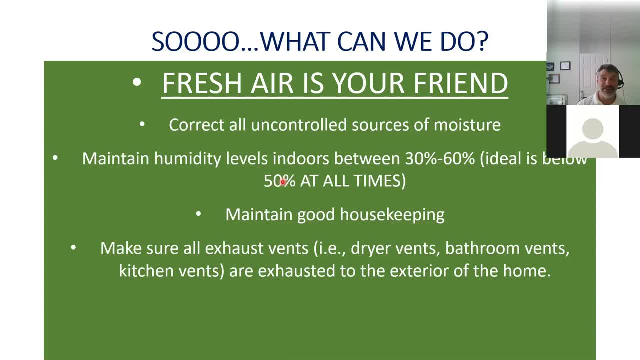 dryer vents are disconnected if they're running through- uh, I've been in homes where they're running through. uh, I've been in homes where they're running through. uh, I've been in homes where they're running through the basement. And if you're starting to see dryer lint all over the 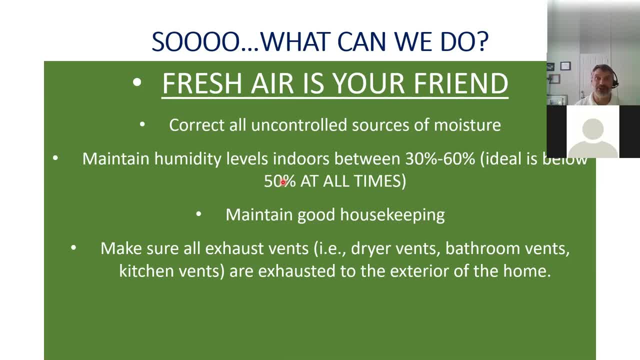 place, then that probably means that there's a disconnect somewhere in your dryer vent. Uh, so making sure your exhaust vents are are connected and exhausted to the exterior. I've gone into attics and older construction standards were different, You know they. they didn't necessarily. 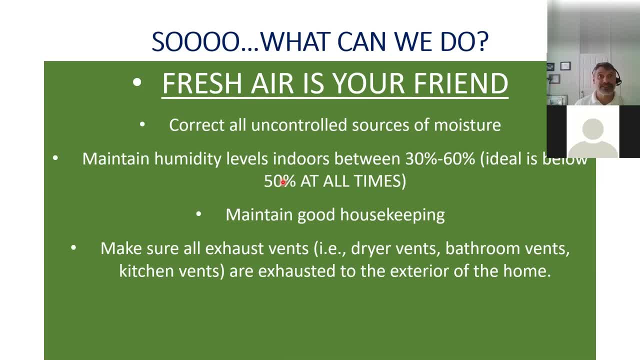 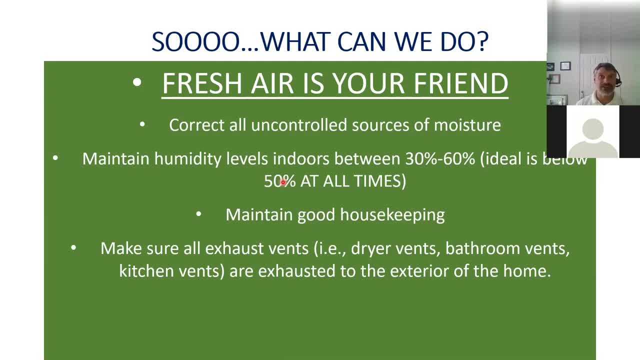 dryer vents and and and a bathroom exhaust vents or kitchen vents, just exhausting directly into the attic. Well, lo and behold, I've gone up in. in an attics There's mold growth heaviest, especially heaviest, right where the dryer or right where the vents are exhausting. 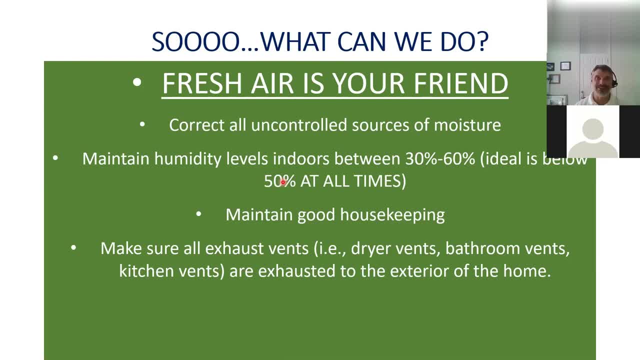 all that moist air um right against the uh, the roof sheathing or the roof boards, And you get a lot of mold growth and, lo and behold, uh and long-term, some structural damage. Make sure your gutters are routinely clean and your downspouts are extended away from the. 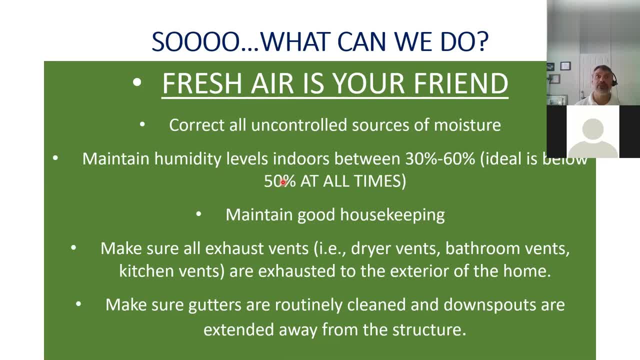 structure from your home. Uh, and that's a very, very common way that moisture gets into the structure. If, if your gutters are not routinely clean and you got water, uh, uh, jumping over or coming over your gutters and water is just penetrating into the foundation, your the. 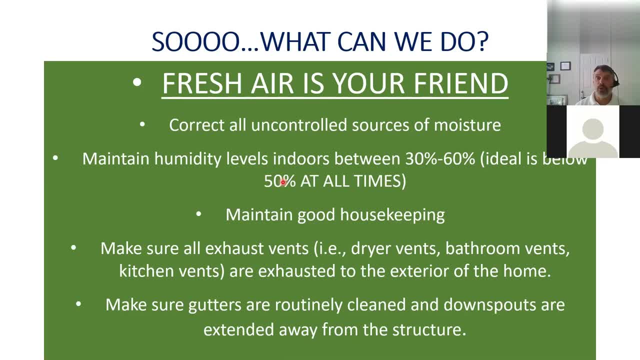 corners of your downspouts. making sure that they're extended away from the structure, Um, generally about three feet or more, if you can, is good, but making sure that, if you have gutter extenders, get them onto your gutters- Um, if they're, I'm sorry if they're not directly. 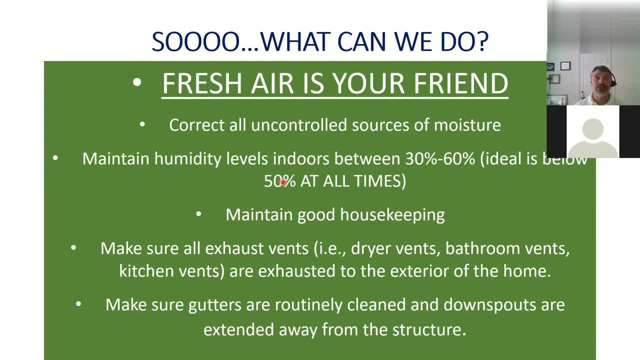 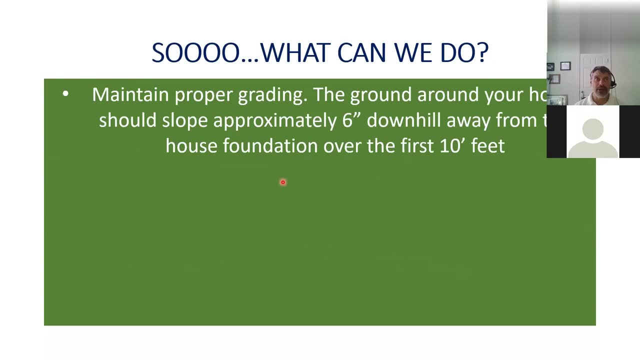 depositing into a drainage system. uh, just get them into. uh, uh, extend those, those downspouts away from the home to stop water, to help stop water from soaking against the um, the foundation, maintain proper grading, And that's another area again of. 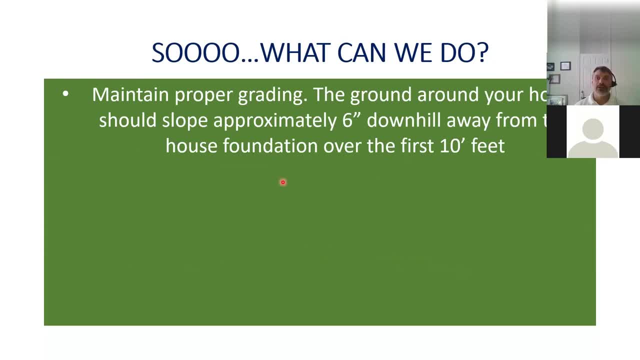 to prevent water from coming into the structure. Uh, so your home really should be sloped approximately six inches downhill away from the foundation over the first 10 feet. If you're not sure that, talk to a landscape architect. yes, Um, increasing your, your um, your um, your soil or? 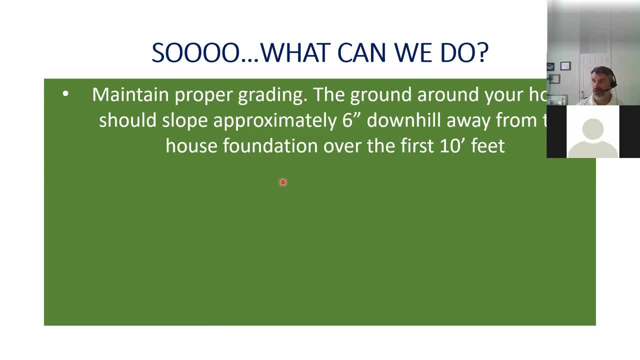 your um uh, if you have landscaping around your home, uh, your mulch can help um keeping uh. keeping your, your plants, your root structure away from the foundation can also help Um, but really keeping the grading, uh make uh try to. 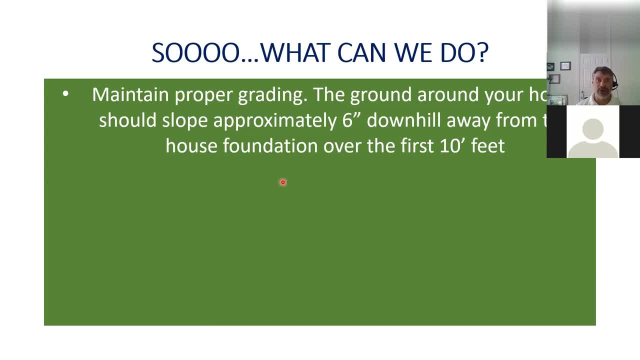 examine to see if you have any neutral or negative grading. So grading around the house helps move water away from the structure. Eliminate or reduce the use of scented fabric sprays, air freshener, plug in stuff Again. uh, those all are emitting volatile organic compounds and people like 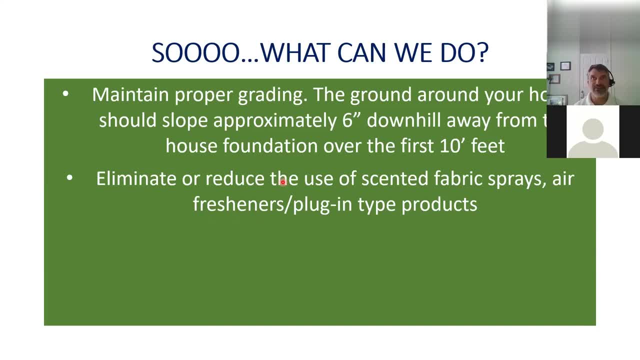 like, sometimes like the odors and like those sprays or those scented stuff. But a lot of them, a lot of them are synthetically made and even some of the natural ones, or some of the uh that uses central oils, can emit some uh do emit some volatile organic compounds which 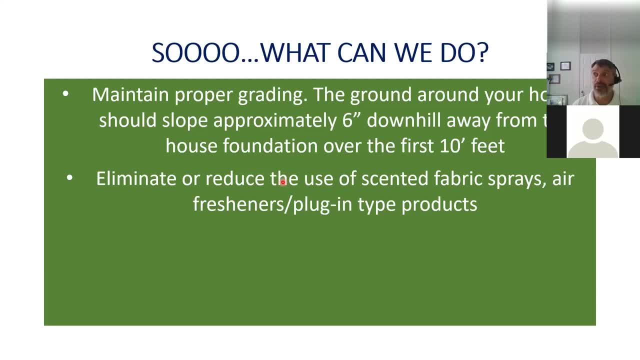 some people are very chemically sensitive and can be- can, uh, that can be a function uh uh or negatively impact the indoor air quality, especially to some individuals. I know I'm very chemically sensitive. I can't even go to a flower store, um, especially florists. 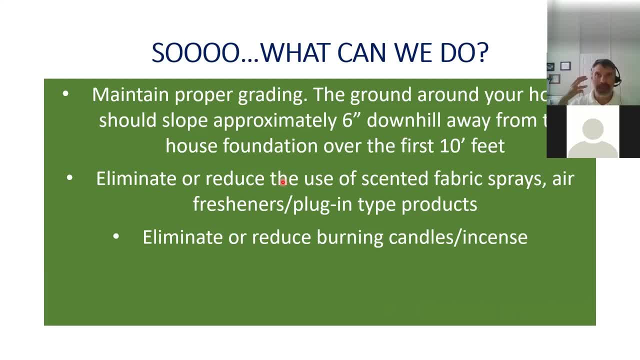 even if they're natural, I immediately my- uh, my head just clogs up almost instantly. Um, if I go into a home that has scented candles or, I'm sorry, those plugin devices, I almost can't go in. Um. 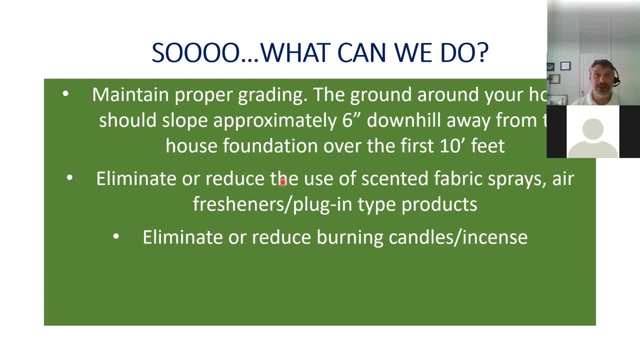 my throat tenses up or tightens up. It's pretty bad. I actually went to visit my mother. I'm going to go off in a little a little uh side story here. Um went to visit my parents and you know. 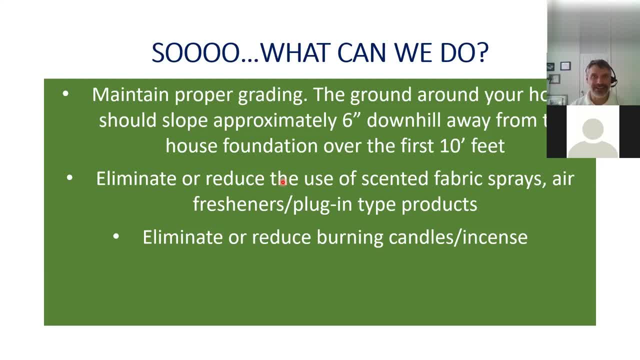 in their guest bedroom. I lay on their bed And the second I lay on the bed. my throat swells up so bad that I I couldn't sleep on the bed. She had used got a coupon for some ball to drop into. 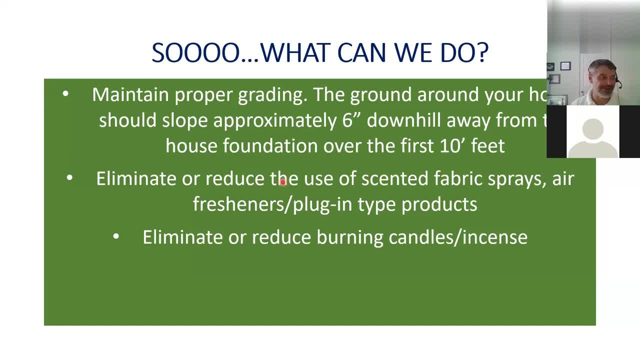 the into the laundry to help make their laundry smell better. Well, that didn't help me very much And, uh, I could not sleep in that bed at all. Uh, it was pretty bad. It was an immediate response. As soon as I laid on that bed, my throat swelled up and I I had trouble breathing. Uh, so uh. 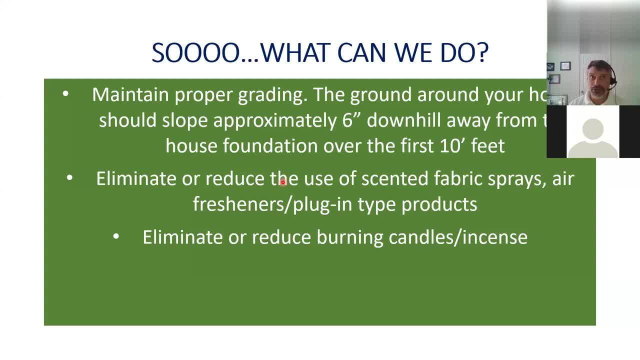 so those types of scented products are uh, do emit VOCs and can elicit uh those types of responses. Eliminate or reduce burning candles or incense? I know many people like to burn candles and you certainly can if it's not affecting you immediately, affecting you or anyone in your 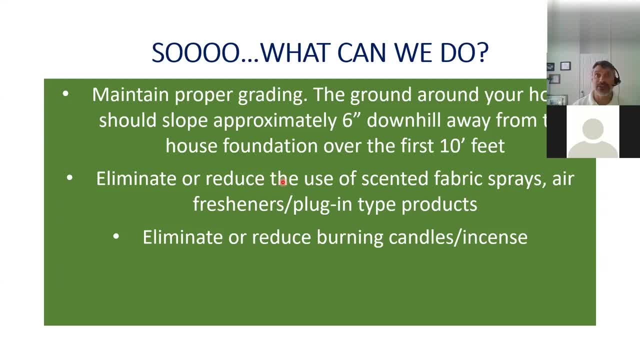 household. you certainly can, but I would certainly reduce them. Cause again, not only are the odors, uh, if you're, if you like, scented products, but also the particulates, the combustion byproducts, if you will, um the smoke. 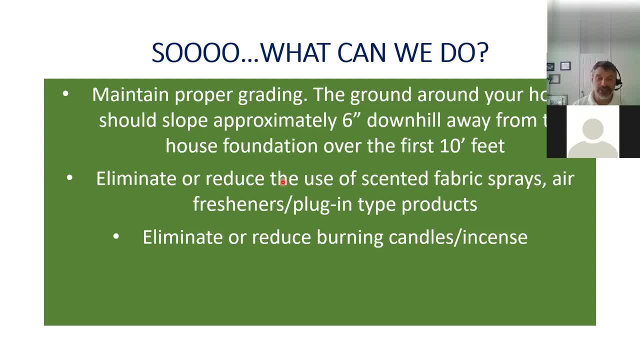 That can linger Um and um, so that's something just to consider. Uh, you also want to consider buying either non-toxic home furnishings. There are plenty of of of resources out there that can offer furniture, mattresses, um or or other. uh. 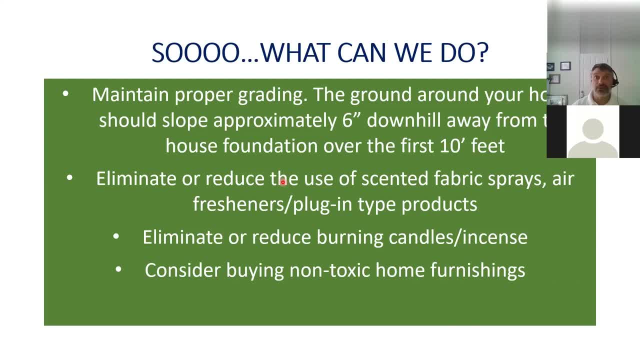 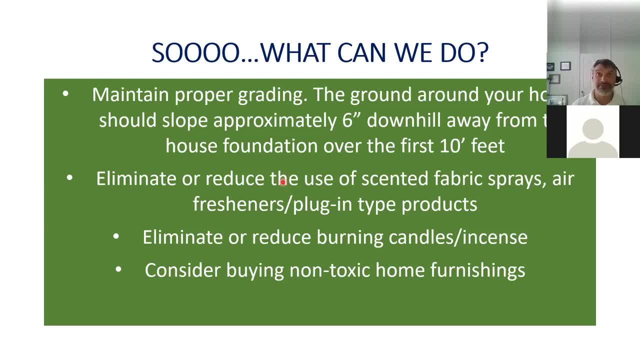 and good, good choices out there. Um, do I have any that I specifically recommend? I really don't have any particular manufacturer, but there are a lot of good sources out there. Um, if you're painting or or refurnishing or or uh uh, refinishing your home, use either zero VOC or 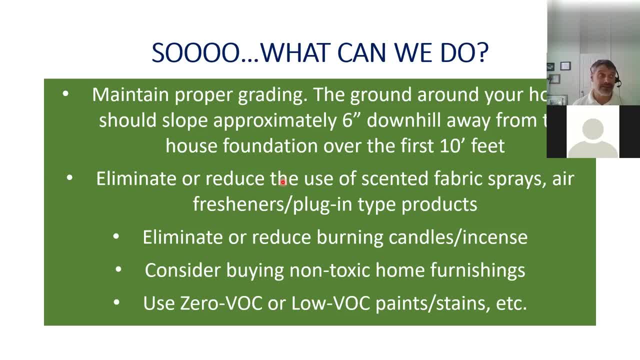 low VOC paints or stains. I can tell you that even if something is labeled low VOC or zero VOC, it's not. that's not always, uh uh. it doesn't mean that there is absolutely no volatile organic compounds, So it can be the base that may have zero VOC and they could actually say zero VOC. 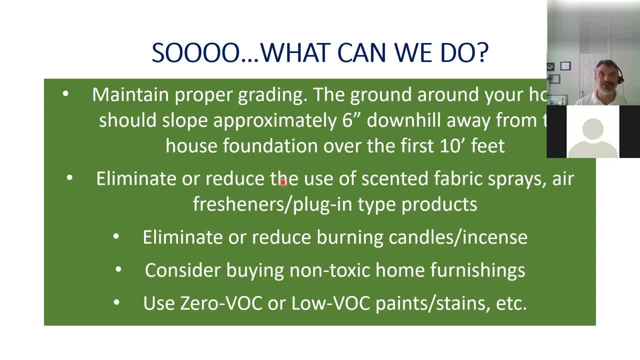 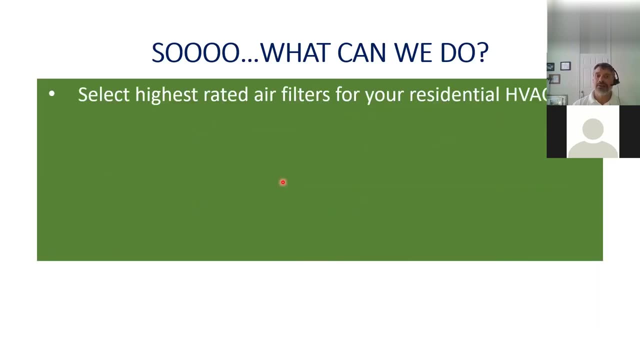 but if pigment is added to it or different paint is added to it to add color, those can have VOC. So so you could reduce it or or reduce your risk as much as possible by using zero or low VOC paints and stains. Uh, you also want to select the highest rated air filters that you can for your residential HVAC. 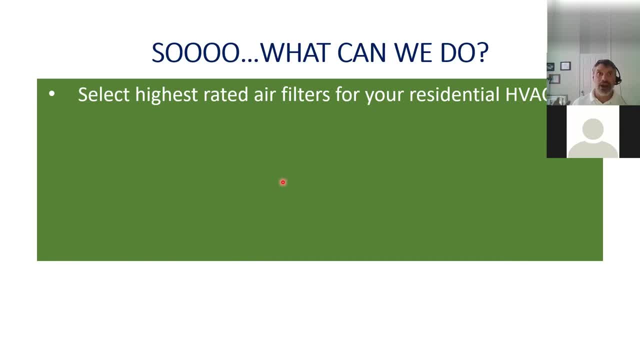 unit. Residential HVAC units are not, are not fitted for HEPA filters, Um, but you can use higher rated, uh, high rated HVAC. I'm sorry, air filled air filters for your home. You really should consult with an HVAC professional, uh, to evaluate your air handler unit, and they should. 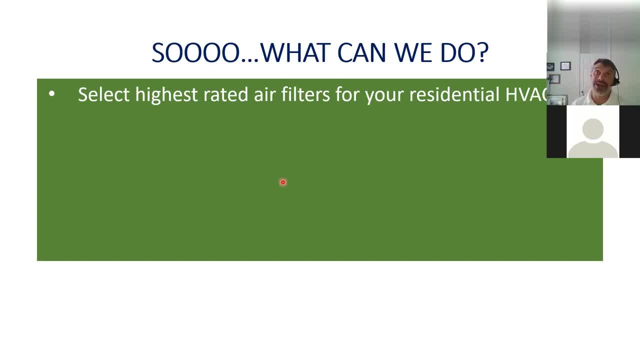 be able to. to tell you, uh, what is the highest rating rated um filter that you could use. The reason for that is is, if you use a filter, that that may be that, uh, that may be too tight for uh, uh, too tight of a filter. 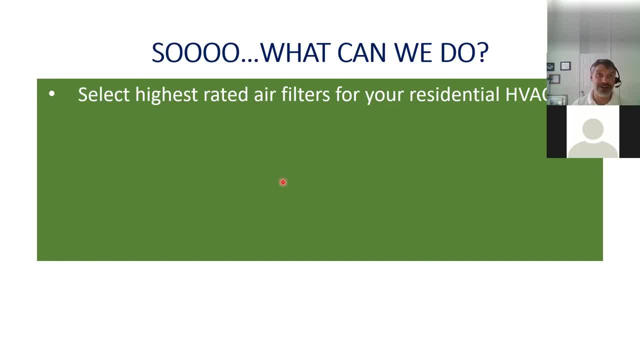 it could actually impact the functionality of your air handling system, Uh, your fan, and it can actually cause premature wear and tear and and and burn out the fan If the fan is trying to draw air through and suck air through that filter and the filter is. 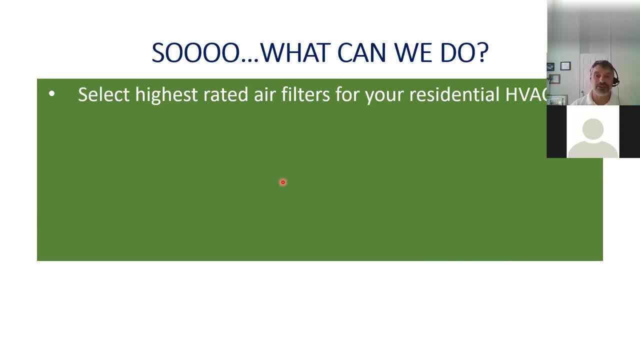 tight. So, uh, but use the highest rated filter that you can for your uh, for your HVAC unit. Most of them that you can find in Lowe's or Home Depot, you know, the highest quality filters are are suitable for most, if not all uh residential HVAC units. But I would certainly 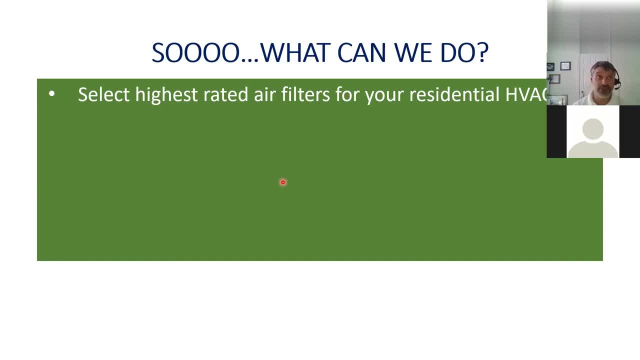 advise. you know uh speaking with with an HVAC professional um standalone air purifiers or HEPA filtered um uh standalone air purifiers certainly do help and can help uh and do re do reduce airborne particulates viruses um uh bacteria things airborne. 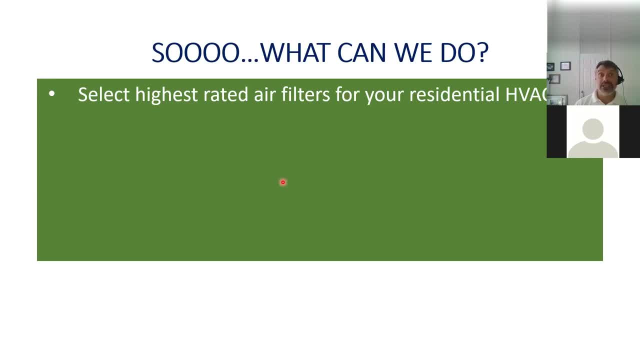 particulates of that nature, for VOCs and or mycotoxins, Um, uh, if you want to use an air purifier, or if you have an air purifier, um, that has a HEPA filter, it should also have a carbon. 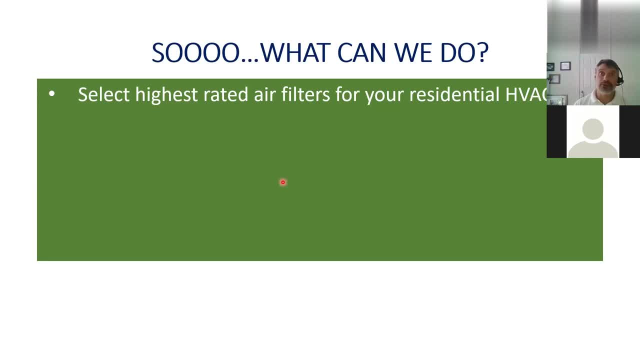 filter. Uh, so the carbon filters help attract those chemical compounds from volatile organic compounds And mycotoxins, Um so, um. so those certainly do help reduce. You'll never have zero stuff in the air. There's always going to be something in the air, and that's very typical and very normal. 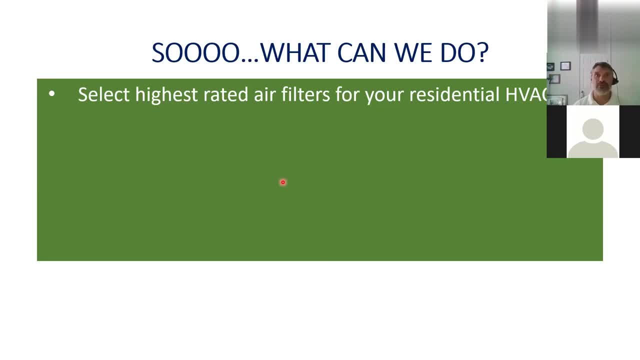 And we should uh, but you can certainly reduce the amount of particulates and and contaminants in the air by using those types of devices. Um going back to carbon monoxide, install low level carbon monoxide monitors. You can find them, Um. most of them that are sold in in the stores are uh have a, uh have a range. 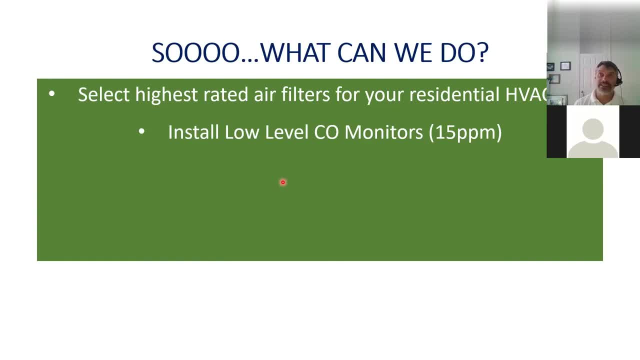 of about 30 parts per million. Try to find one that that is sensitive enough to 15 parts per million. Um, they tend to be a little bit more more accurate And um so um, I would certainly advise buying low level carbon monoxide monitors. Ensure that your sump pumps if you have a sump. pump, um, make sure that they're all in the right place. So, if you have a sump pump, um, make sure that they're all in the right place. So if you have a sump pump, make sure that they're all in the. 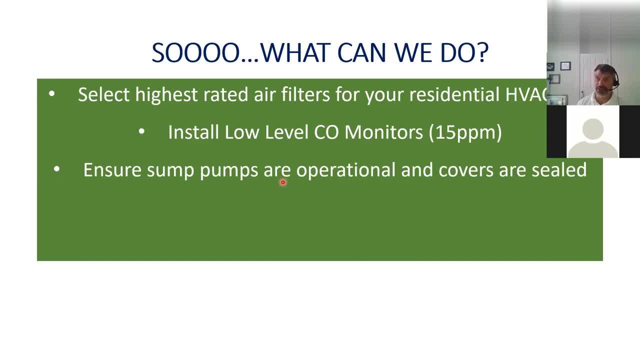 right place. So if you have a sump pump, make sure that they're all in the right place. So if you have operational and that covers and that, uh, the covers are sealed. Um, so for two reasons: not only for to evacuate water out of the structure, but also radon can does penetrate through uh. 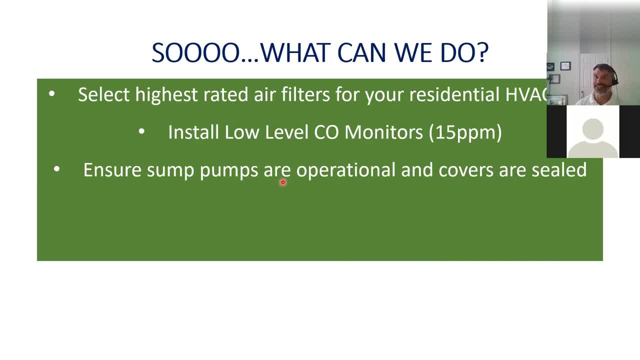 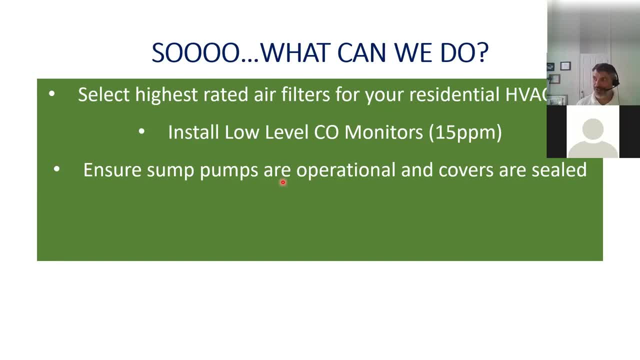 in closets or or in a small built-in cabinet area where sumps are are. uh, sumps can be located Well, that water can evaporate And I have seen molds, mold growth, start developing in enclosed closets or cabinets that are covering those sumps that don't necessarily have covers on. 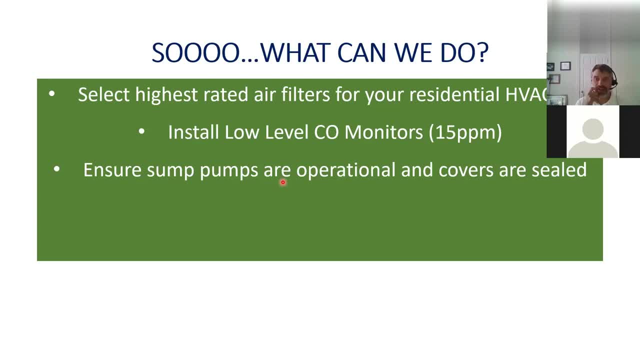 them So that water is just evaporating up and then causing, uh, causing mold growth onto those building materials. So, uh and uh, again dealing with radon, again sealing cracks or openings in your foundation walls or your slabs. Again, you can, you can do. 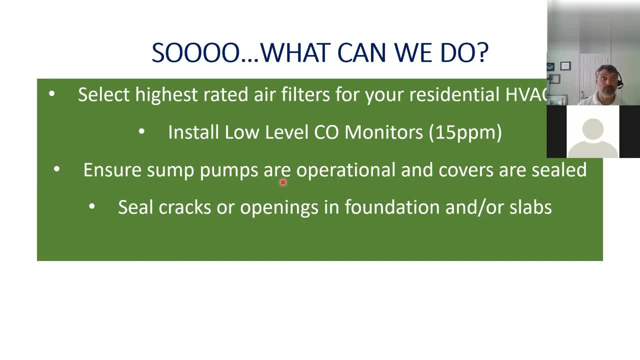 it using a silicone caulk or or other sealants that are rated for either foundation uh, concrete or cinder block. Again, it's best to to uh speak with a renegade um, a radon mitigation specialist uh to evaluate, but there are simple things that you could do to help. 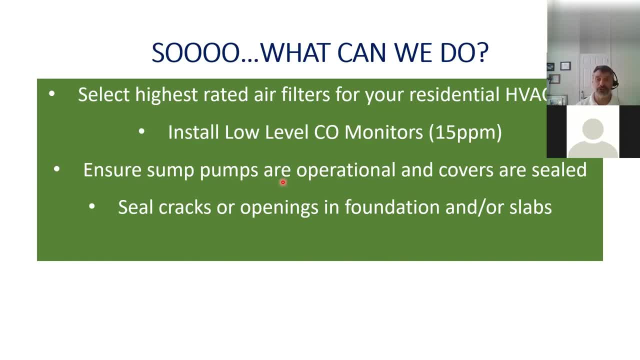 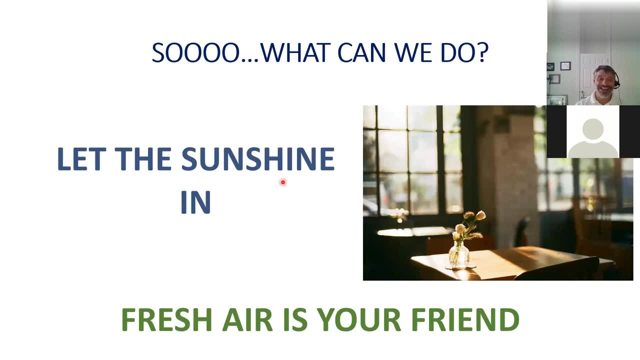 reduce radon from entering into your structure. Last thing that I'm going to say is: uh, let the sunshine in and also fresh air. Again, fresh air is your friend. open windows whenever possible, And that will certainly help reduce and improve the indoor air quality. Uh, here are some. 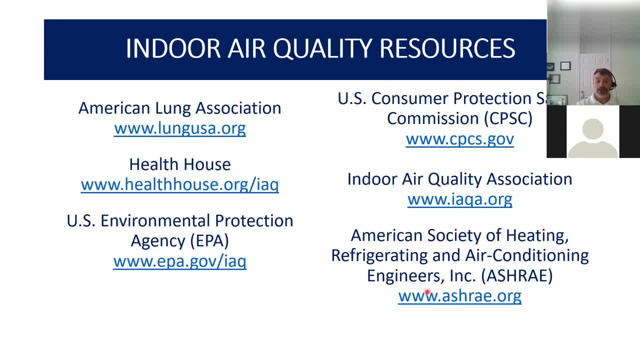 really good resources and I'll keep this up on the screen, uh, to find out more. And let me take this laser off. I forgot I had it on um, American lung association, health houseorg- that health houseorg certainly provides a lot of resources And I'll keep this up on the screen to find out. 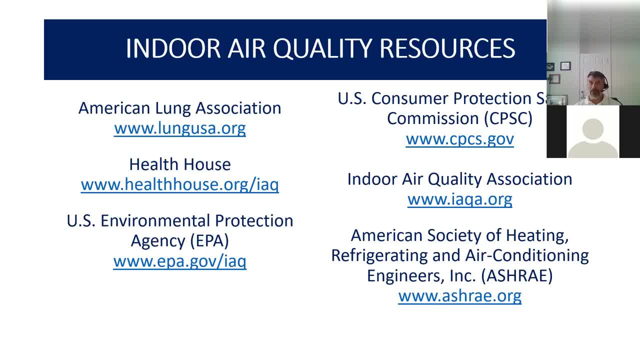 more about the resources, especially for for furniture furnishings. Um, and then you may want to look into EPA, has a lot of good information about indoor air quality, consumer protection safety commission, uh, indoor air quality association, which I am a member of. Um, there's. 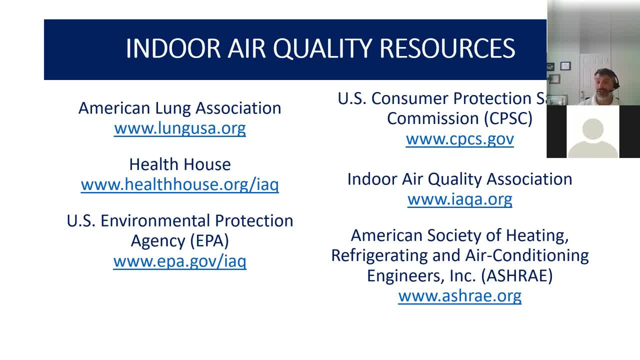 a lot of really good resources on on their website. Asherah, the American society in heating, refrigeration, air conditioning, engineers- these all have really good resources uh for for consumers and general users. So thank you, Thank you. 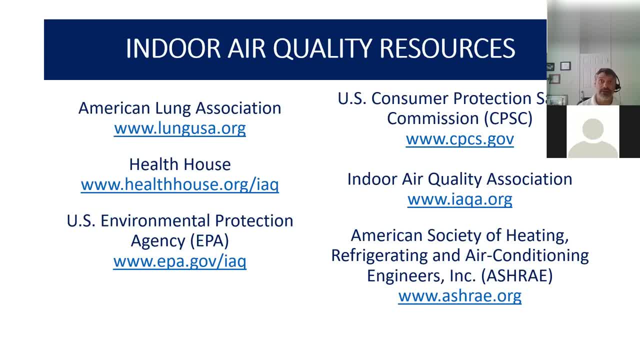 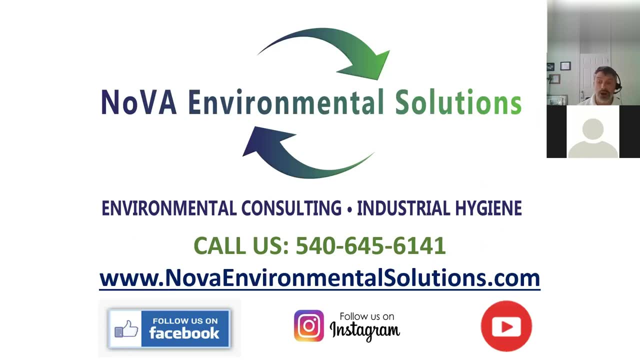 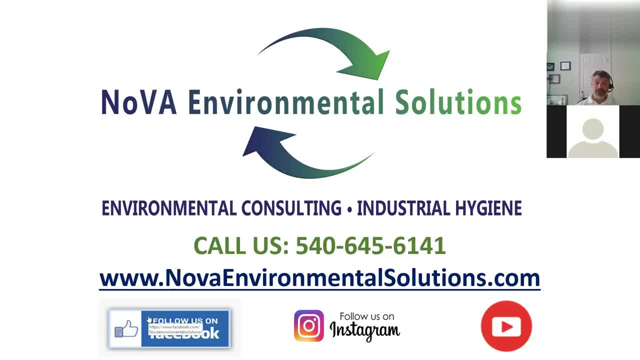 but our phone number's on there. Our website is novaenvironmentalsolutionscom. We are on Facebook. We've been posting a lot of good information, a lot of tips and other information. We are on Instagram And we just started a YouTube channel. 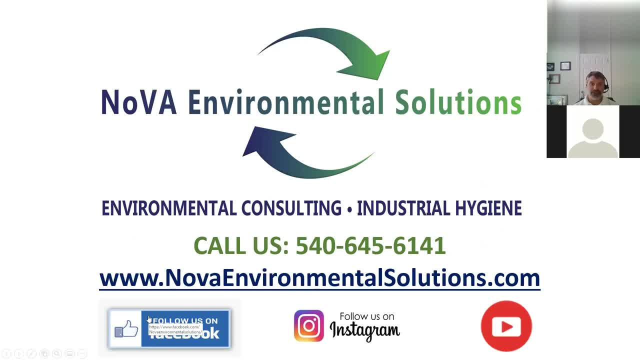 I am going to at some point upload this presentation to our YouTube channel, But we also are going to be adding in. we do have a few videos up now on our YouTube channel, but we're going to be uploading additional videos dealing with not only mold but other indoor air quality. 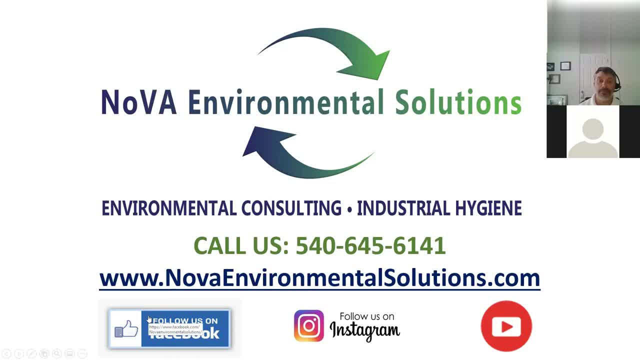 more specific indoor air quality testing and things of that nature. But at this point I'm going to open it up to any questions that you know someone may have And let's see if I can. I'll start with a question to get things rolling. 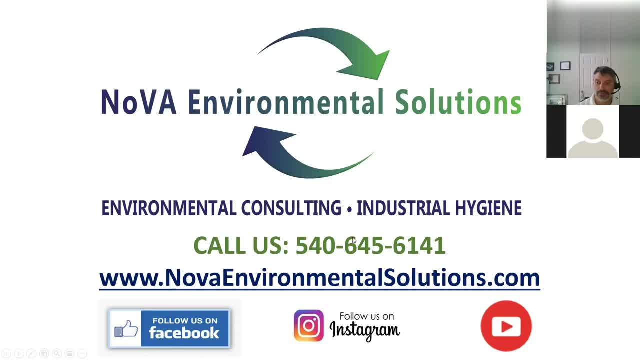 You had said during the last lecture that you will sometimes let your fan go in your basement to keep air circulating to prevent mold. I was wondering if you still recommend that. Yeah, so, especially if it's an unused or an unfinished basement and you don't have air conditioning vents. 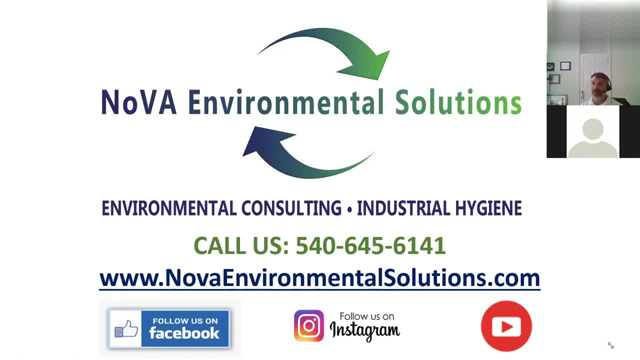 or air circulation going. running fans in a basement is a good way to keep air movement, And so what air movement does is it helps prevent or it helps allow for evaporation of moisture, so of dampness, humidity, but it also keeps air movement going. 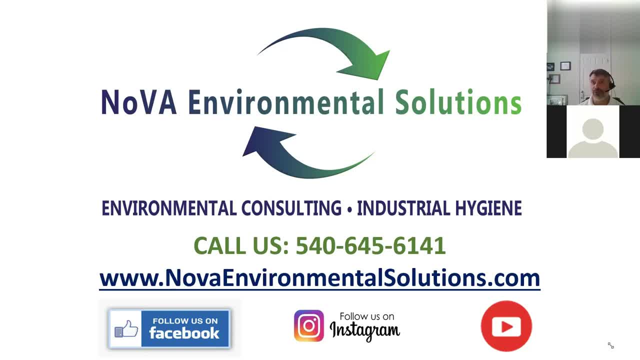 So keeping air movement is really key, Keeping your vents open. so it's not So if you're in rooms a lot- and that brings me to another good point- is in your house. I've been in many houses where they say, well, we don't use this room. 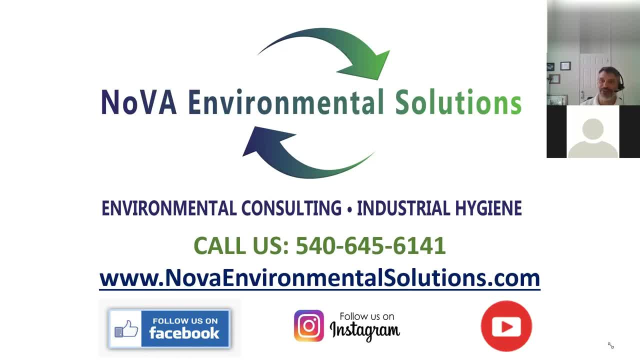 so we're going to close the vents, or we don't use the basement anymore and we're going to close all the vents. Well, that's not necessarily the best thing to do. Again, air stagnation can help promote or allow humidity to build up in those areas. 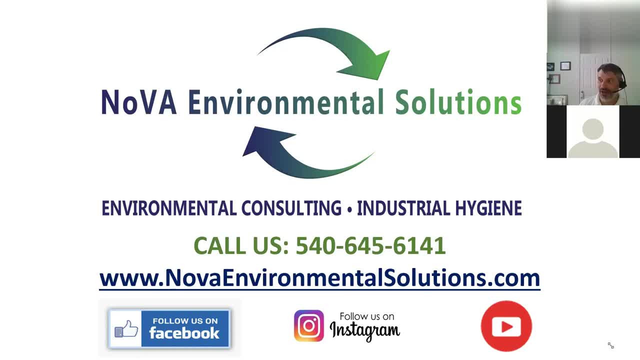 especially at this time of year, And that humidity lack of air movement can allow for, for that moisture, that humidity to absorb into the building materials, whether it be drywall wood framing underneath stairs to allow for molds to start growing on ceiling joists. 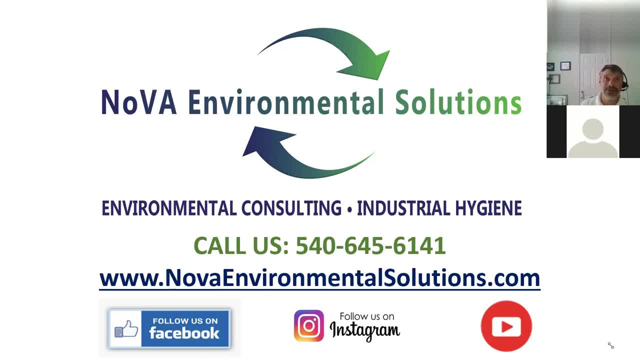 If you have a crawl space. I know many homes in this area and many homes in the region were built with the crawl spaces that are vented, with the theory being: well, you're going to get air movement and it's going to help dry things out. 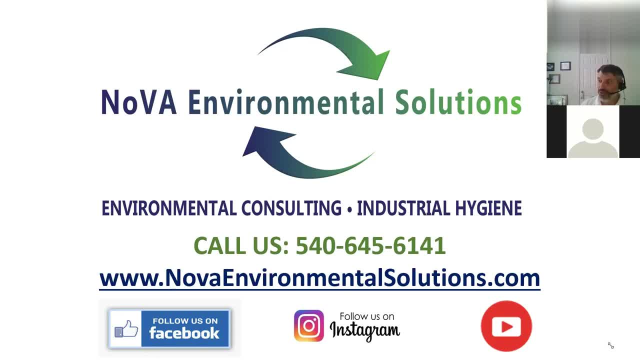 Well, new research and new standards are beginning to change, or standards are beginning to change where it's now best that crawl spaces should be sealed and be climate controlled With vented crawl spaces. that's allowing the humid air to come in And if you have a soil floor. 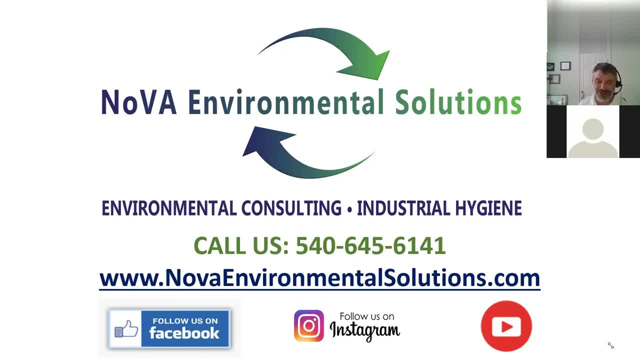 even if you have a vapor barrier installed on your crawl space. crawl space issues are very, very common And contaminants that build up in crawl spaces can permeate into the living space and can affect the indoor air quality. So and we get into. 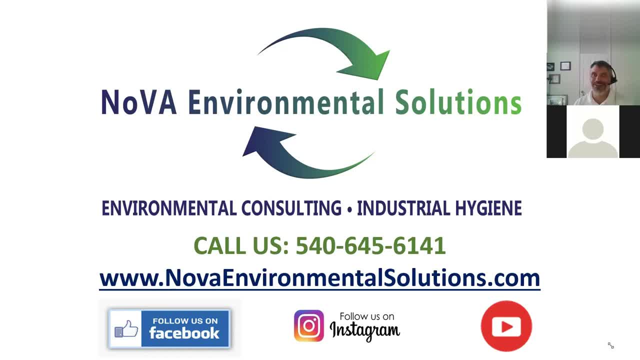 into crawl space issues at another time. but. but I hope that. but yes, so running fans, keeping air movement going, is really a really good preventative measure, a way to help to help control or to prevent moisture from building up on building materials. 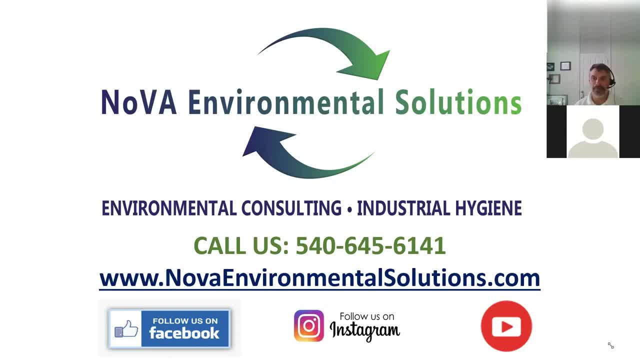 What if you have a crawl space and you have a moisture barrier? what would one do, You know, if you say they have a 120 year old house with a crawl space and a brand new moisture barrier? what else can you do to prevent mold? 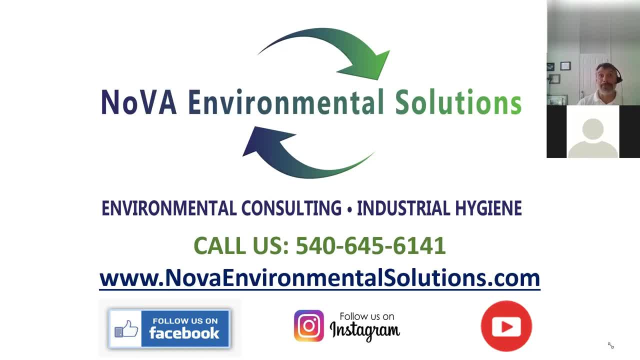 Yeah, so they well. vapor barriers are the evaluation of the vapor barrier. So really, vapor barriers, vapor retarders are two different things. but vapor barriers should be staked down to the ground, They shouldn't be loosely laid run up the foundation walls. 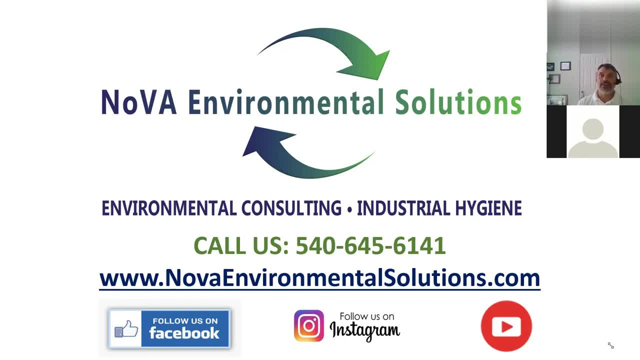 run up the columns and be sealed. But if it's still a vented space you may want to consider having it sealed And I do have have resources that that do this type of work, that do enclose that that crawl space and and install mechanical 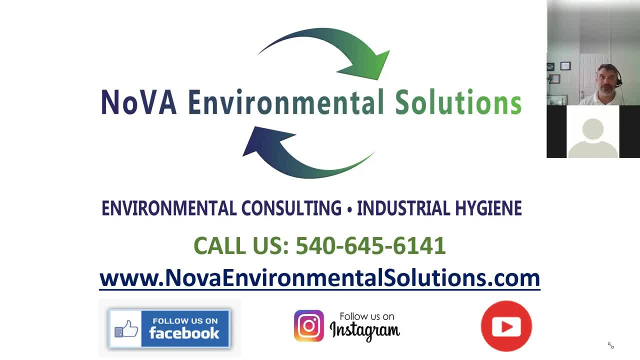 mechanical devices to climate, climate climate control and dehumidify that space. Vapor barriers do help prevent moisture from permeating up from from groundwater, from the evaporation of water from the groundwater, But again we're also talking about moisture. 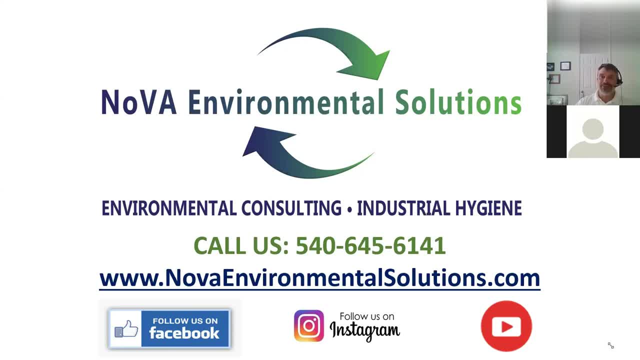 that comes in from humidity from the vents. Some studies suggest that if it's, if there's relative humidity between 60 and 70% outside, that humidity inside of a vented crawl space can reach between 90 and 100%. So it's anyone else have questions and let me stop. 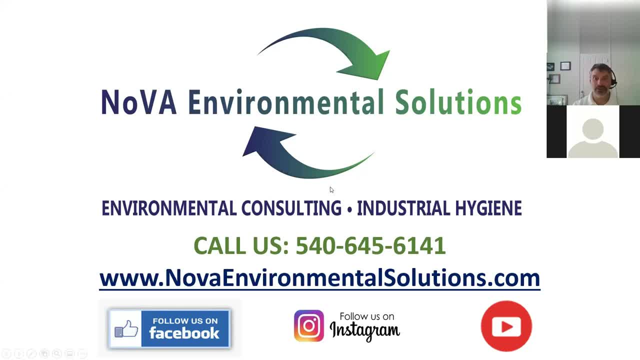 I have another one if no one else is going to ask chat. Oh, I see a chat from. should sink in shower drains be clean somehow to avoid black mold collecting? So I'm going to address that. So not all molds that are black are the black mold. 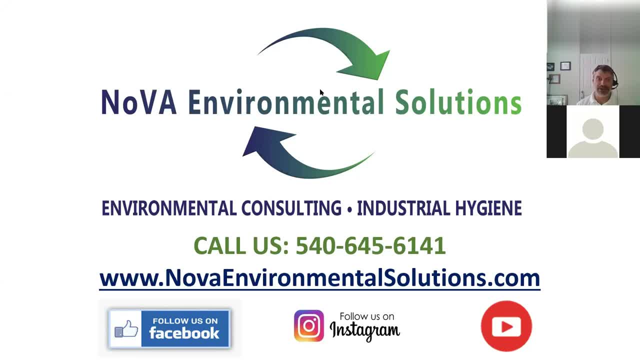 There are several molds that are black in color, So what we take typically found around in shower drains or in sinks, um in in in bathrooms. yes, there can be. it can be black in color, Uh, but most of the time 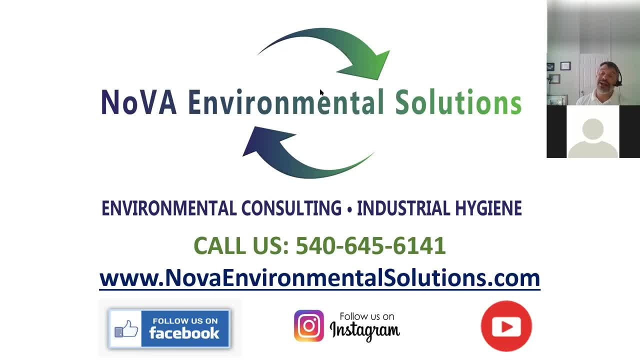 the vast majority of the time it's a. it's a relatively a cosmetic mold called cloud, a spore um, which does have a blackened appearance. It really likes just soap scum and another. you know, just the natural, organic manner that builds up around the drains. 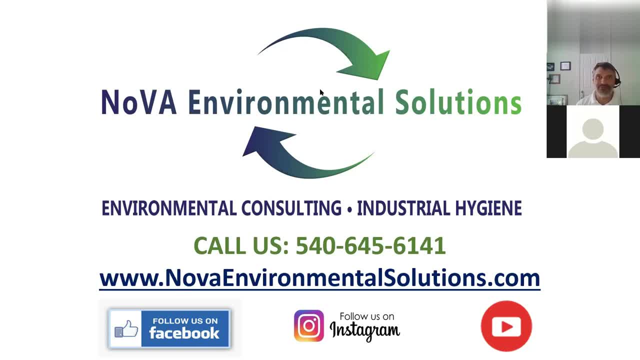 and showers. Once it starts building up, it can be very difficult to to completely remove. remove constantly without thorough cleaning every day. If it's on grout or on caulk lines, which is very common, routine cleaning can help it. But if it's just an annoyance and you want, 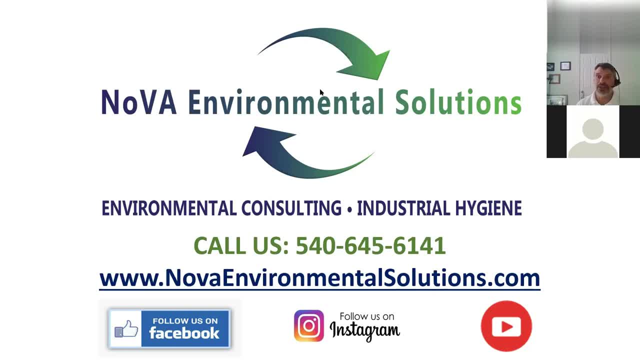 to get rid of it. you may need to replace the caulk or grout and redo it that way, But it's really not generally a health concern because it is not going to be- quote unquote- the black mold that everyone hears about. That is black mold. The one that is most concerning is a mold type. 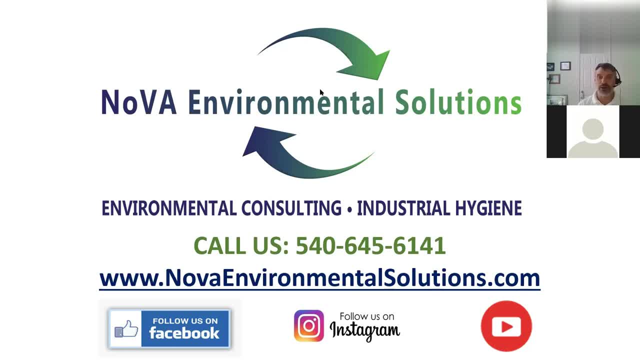 called stachybotrys. You're not going to find that on shower drains or sinks, So it's difficult to have it. stop from collecting, if you will, around the sinks and the drains. It's more just a cleaning maintenance. Yeah, it's ugly And sometimes it can stink, But there's really. 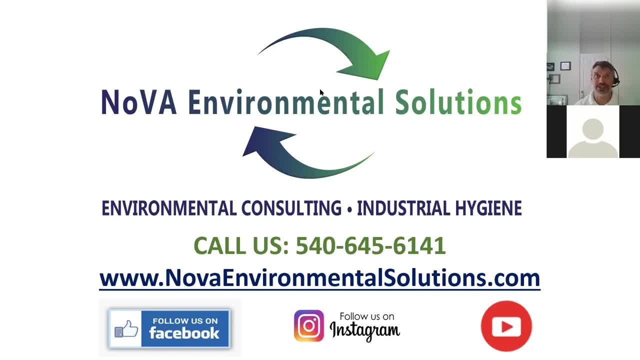 no, No special formula other than routine cleaning. Not one particular product that I would say cleaning agent works better than the other. A good scrubbing, cleaning just really is the only way to maintain that. I have a question for you. Yes, About three years ago, well, about four years ago, we bought a house And shortly after we 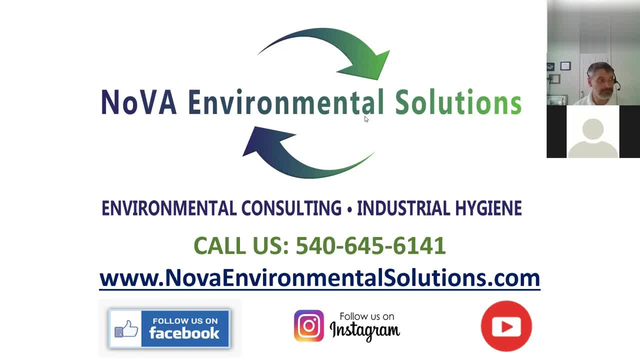 discovered. We have a full built-out basement. It's in the green And our kitchen is downstairs And the other side is two bedrooms And we were trying to do some remodeling. So we pulled down paneling and discovered a leaky window and mold on the. 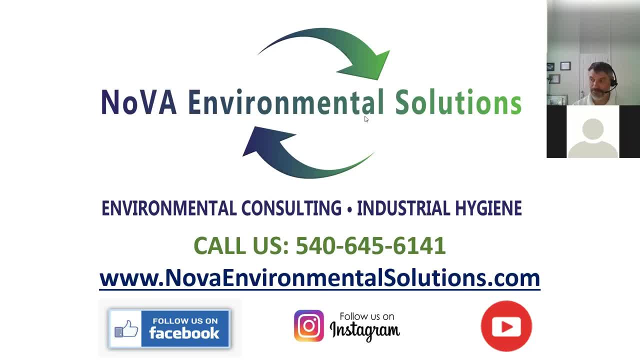 foundation. So we had a company come in and do remediation. Everything was stripped down to the foundation And essentially even studs replaced almost in those two rooms, But the kitchen wasn't Pulled back off the foundation. Now they said that they only found mold on those, And I know you. 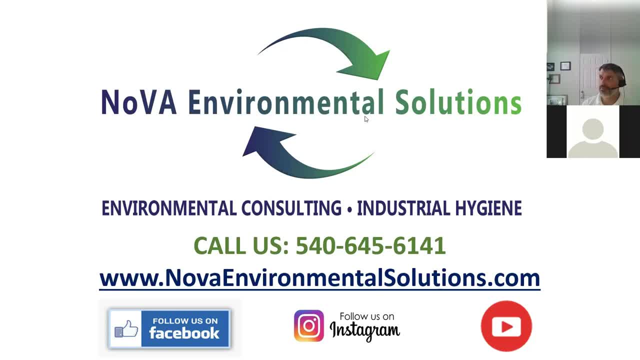 guys didn't do it, But they saw the mold and they cleaned it up along the foundation side and the side And they dug out on the outside of the house to redo waterproofing and put in the new drainage system. Yep, So then they also Because I was concerned about the kitchen walls. 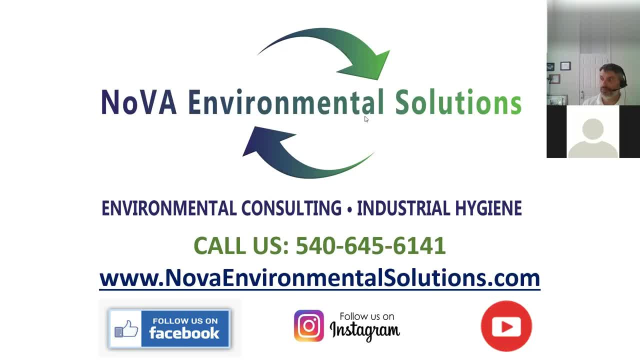 we couldn't take it apart. So they said: said they came in and sprayed some stuff like in the whole house. it's almost like they fumigated the whole house. yeah, fogging was right, something like that, but for to try and kill everything, that. 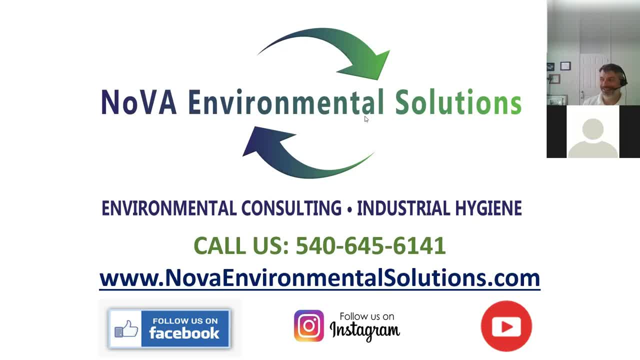 might be growing. is that effective? no, unfortunately it really isn't. um and here's a couple things. so, as far as killing mold and or removing mold, the objective first of all for any remediation work should never be to kill mold. dead mold is still allergenic, toxigenic, it could still become airborne. 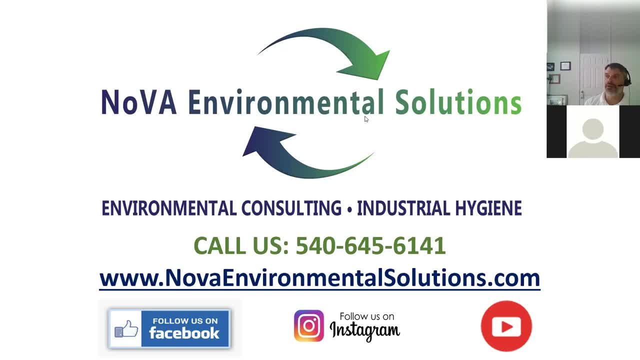 um, but um. so there are the professional standards call for the removal of mold. but spraying and and fogging, what the theory is? and yes, it can denture some airborne spores. when the fog part, when the fog, uh fog- is in the air, settles it to the ground. 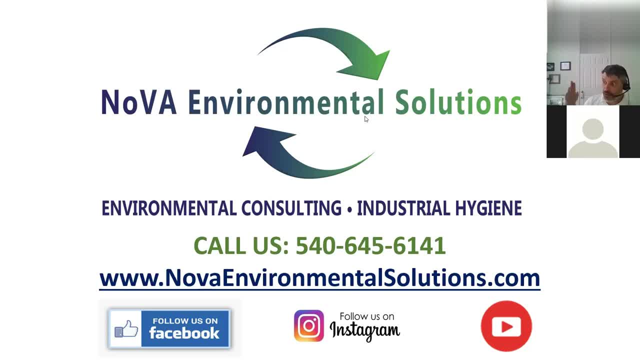 is it going to get and be effective at quote-unquote killing inside cavities and inside spaces? no, i i have not seen it. i know most professionals in our industry have not seen really good research that shows that it's really effective to do anything. um, even if they claim it. 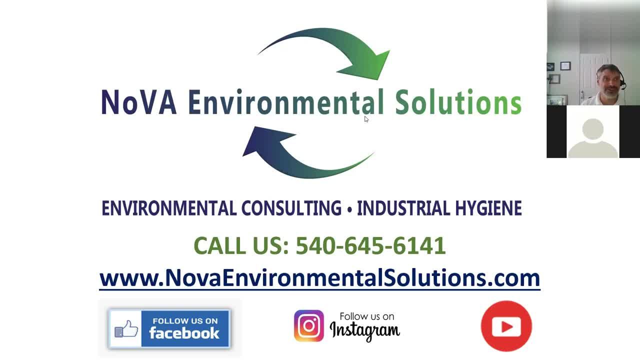 kills um um 99.9 percent of all molds and and biological contaminants. well again, killing isn't the objective, it's removing it. and secondly, uh, you mean to tell me that you can leave a little bit is okay. well, i, i just, it's just not real effective. so, but what i can say is from what you described. 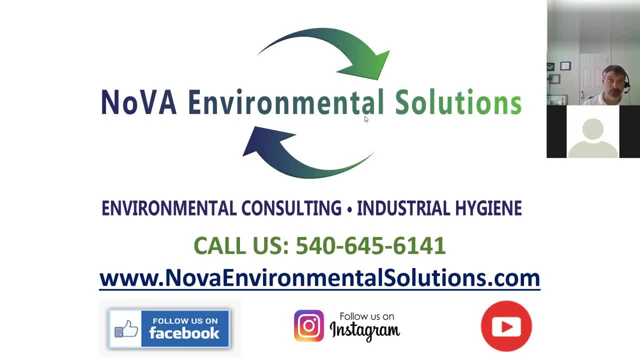 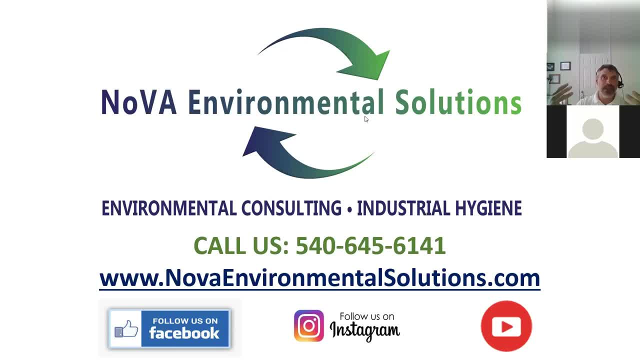 originating around around a window frame or a leaky window. anything below that has is more likely to be uh to be affected, and the lower the water traveled, the more likely it is to be affected at the lowest point. so typically if there's leaks around windows or or from or from flooding or 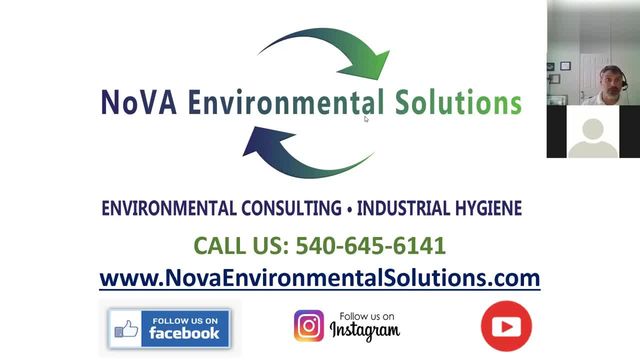 or things of that nature. we tend to find the worst of it and we tend to find the worst carbon level, the mold growth around the bottom foot to two feet of the affected wall, and it gets less than the higher up it goes, um more. just from capillary suction water will only suck up, so so far, and then 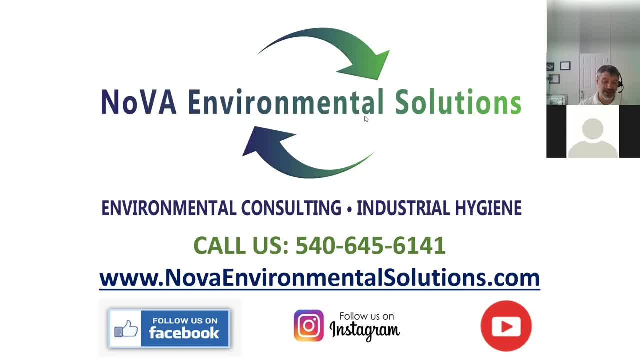 conversely, when water comes in, it's gonna, it's going to travel and get to the lowest point that it can. but could could there still be molds present? uh, behind that, behind your kitchen wall, you know it, it's. anything is possible, and, and especially if i don't know if there was any- 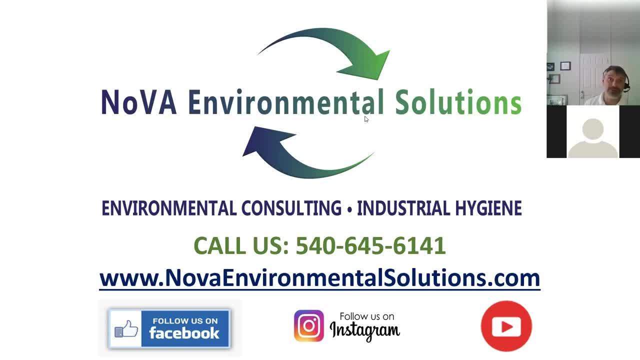 if any sections were of that kitchen wall were opened up to investigate or any any specific sampling methods were used to investigate at that time. maybe or maybe not, but again, um, you typically try to go where the evidence is pointing to and where the trot where water travels to, um, and that's typically what it's going to be: the most affected areas. 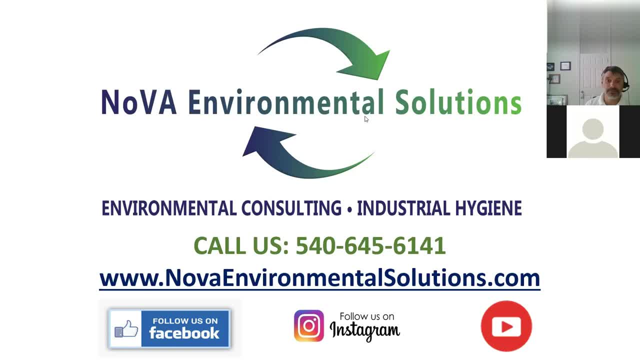 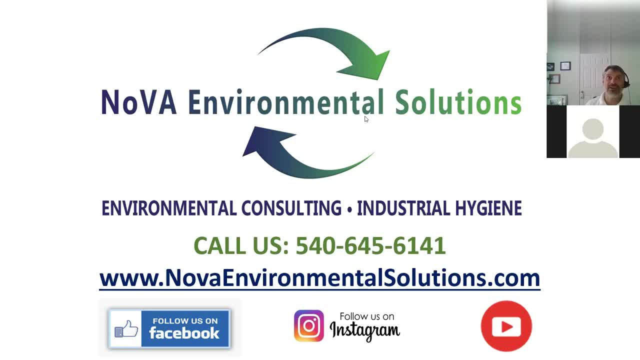 and i do write up remediation protocols, uh for remediators to follow that. it's a benefit to both the homeowners, or the building owners, and the remediators. they're getting an independence based on of, based on an actual assessment, identifying the known areas but citing 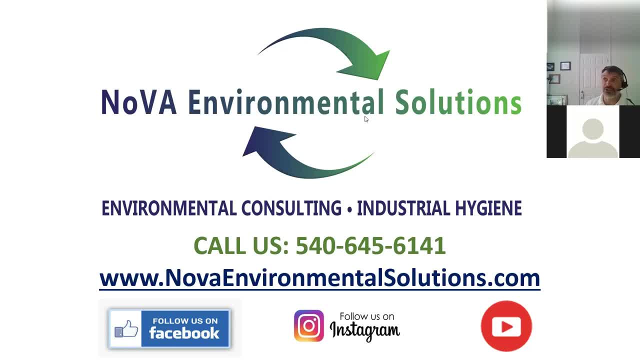 professionals, the, the professional sources or the industry sources, uh, of standards that you know, spraying, fogging, killing mold is is not remediation work. um, so if someone was, because there are companies that say we will come in and remediate by spraying and fogging, well, they're not doing remediation work. so, and i've, unfortunately i've been involved. 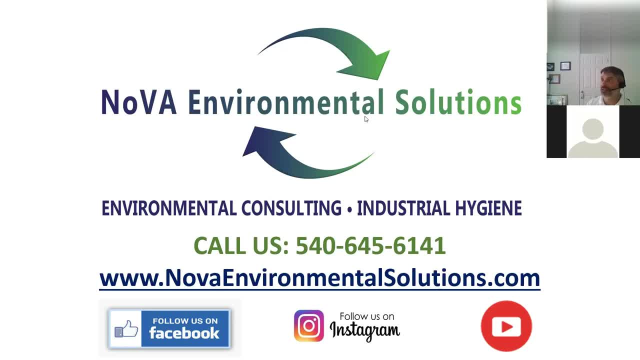 with a lot of, with several clients who hire these companies and spend thousands of dollars. didn't they come in and spray their house with a false sense of security that that they got rid of all the mold, and when they really didn't? and they're still reacting and still having similar, similar? 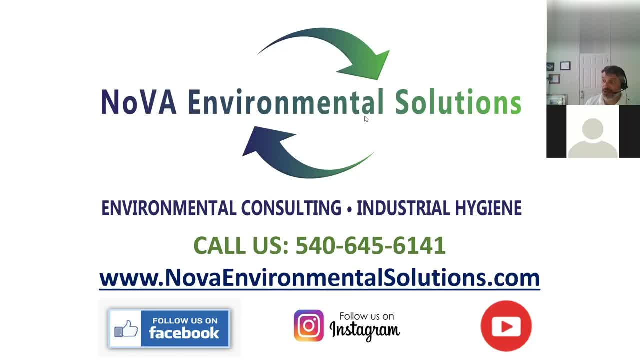 symptoms once they're back in the house. and i pointed out- so we'll look at all this mold that's still here. it's visible, we can actually see it and it extends into invisible areas by certain testing that we do and they're still responding so um so, if spray, but i have seen that spraying or fogging- many remediators will add that on. 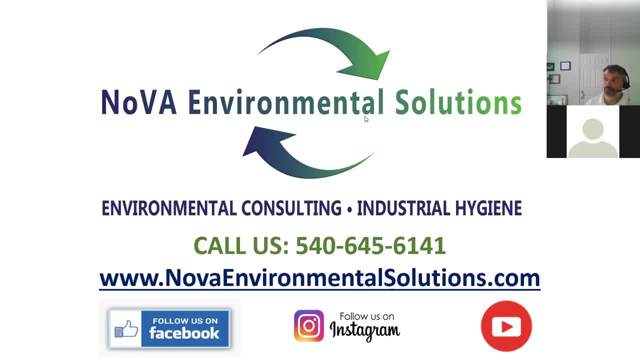 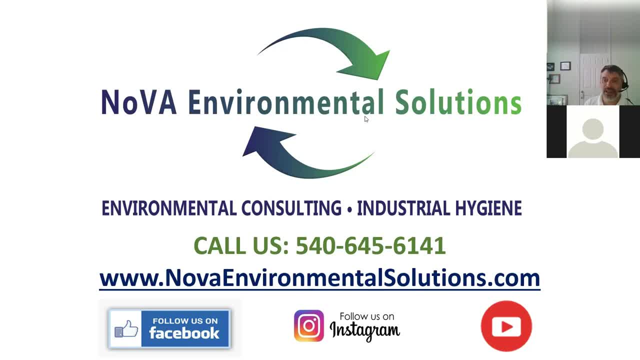 anyone else. i have one. what would you um recommend for folks that are like wanting to one purchase a house and to have their house tested? you know they don't have any great concerns but they're interested in having somebody to look to see if there's mold or 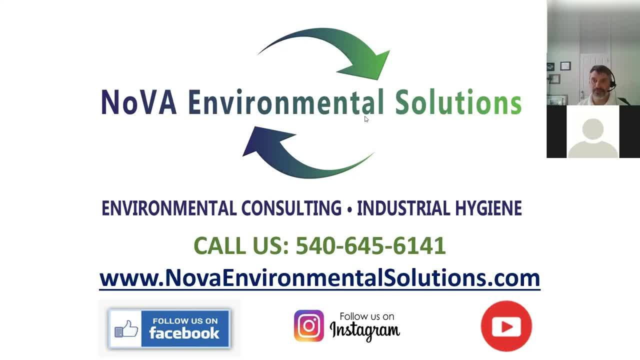 if there's things that are in place that could potentiate or or lead to mold, right, yeah, so i'll jump to that one first, or even as a pre-purchase. so, and this goes with any air quality, uh, testing or assessing testing alone does not tell the story. there are companies out. 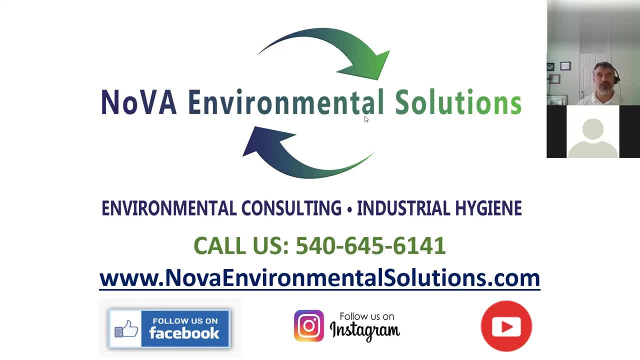 there. there are people in there. yeah, we could do mold testing. well, are you doing an assessment? well, no, we're just doing the testing. testing and sampling alone does not tell the story. it's a piece of the puzzle. so any assessment, whether it be for mold or other indoor air- 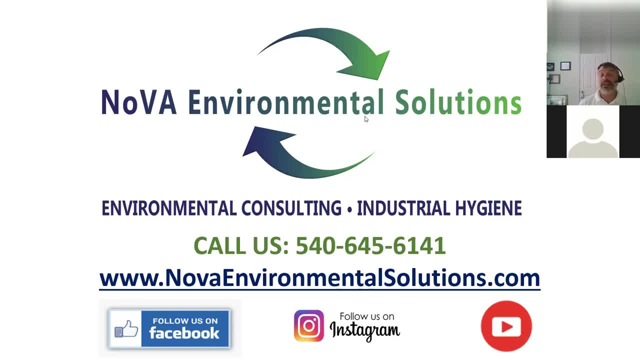 quality contaminants should involve a good getting as much background as getting as much history as possible, uh, of the structure, uh, you know, as far as you know, water intrusion, previous floods, leaks, things of that nature. a good, thorough visual inspection by someone who's trained and knows what they're looking for, using devices like thermal imaging. 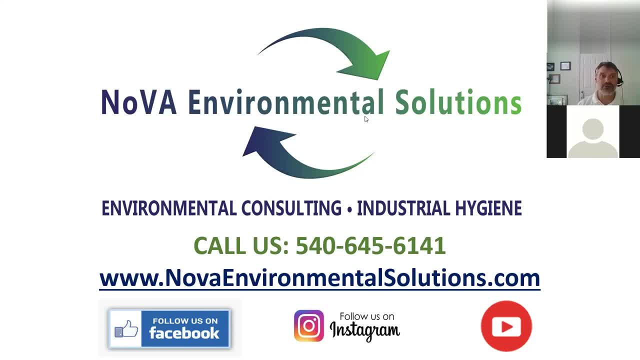 which we use in other moisture meter devices to look for areas, not only if there's any current moisture retention, but thermal imaging also could show where, areas where there may be, you know, gaps around windows or doors or missing insulation which can lead to water, then that can penetrate. 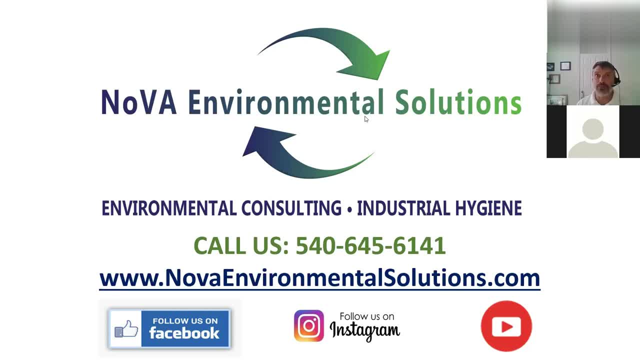 in from from an exterior window or areas where there where materials can condensate, um measuring levels of temperature and relative humidity. so those should all be functions of a good assessment, in addition to sampling, and the sampling should have, should be a hypothesis driven. uh, uh, uh. 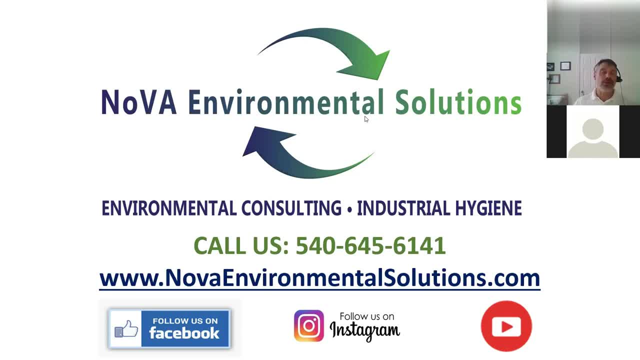 sampling strategy. so why are we sampling? what are we sampling for? what are we comparing against? what information are we trying to gather to to help us, uh, um, come up with any conclusions or opinions about what we're, what we're investigating. so all sampling should have, should be a: a. 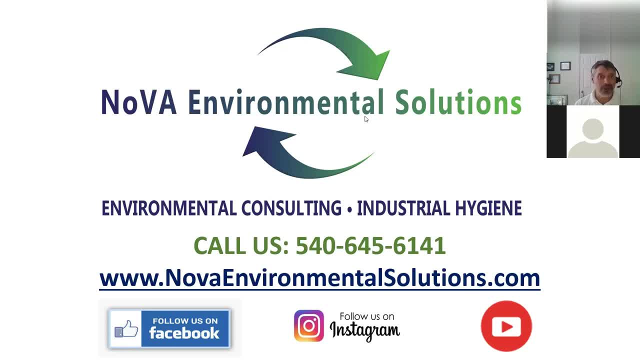 hypothesis driven, uh, sample strategy again. so i know people who- and i and many of you may, have done it or have been advised to do it- do a hurts me or an ermie, or do a petri dish. well, what is that? telling us? not much. it really is not telling us much, um, and if you have done an ermie or it, 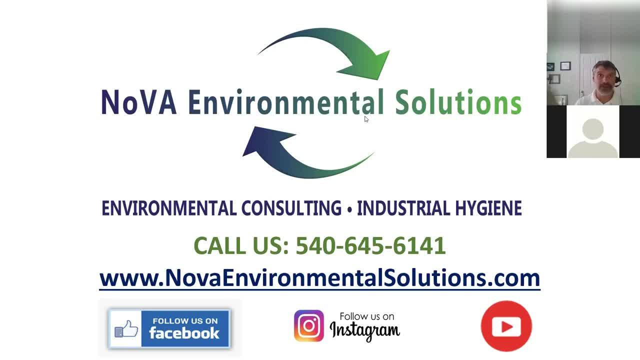 hurts me and have just done a swiffer on several different surfaces throughout the home. you're not getting a lot of good information other than, yeah, there's some molds in your dust. well, i could say that in a hundred percent of all structures there's going to be some mold. 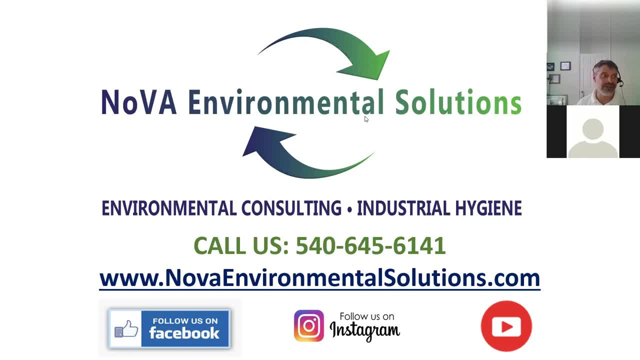 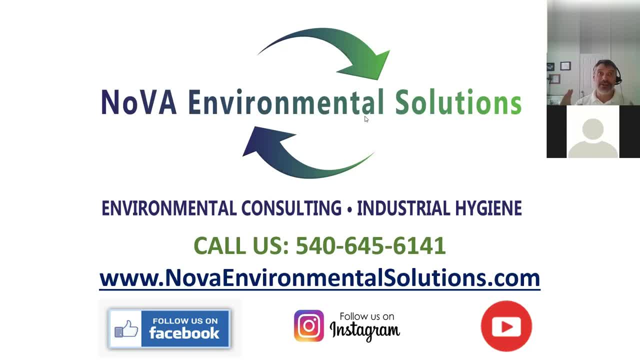 method. that's supposed to be a environmental moldiness. uh um, uh, uh. whatever the acronym stands for, it's off the top of my head. it's getting late in the day. uh uh, an index. it was developed by the us epa for a specific study that they were doing. it was, and the epa even said it. 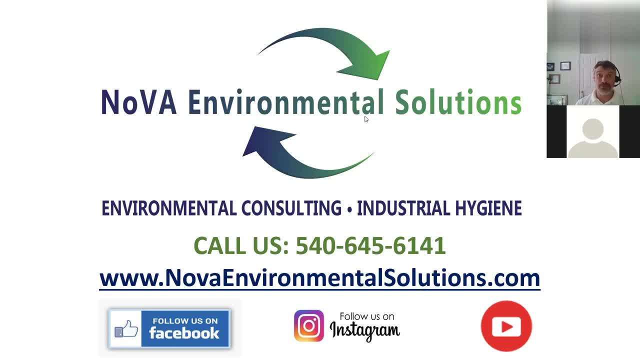 was never intended for public consumption but to get a. many people still want an ermie score to see how moldy is my home, how moldy is my home. to get a true ermie score you have to use the correct ermie sampling method. i have done ermie. 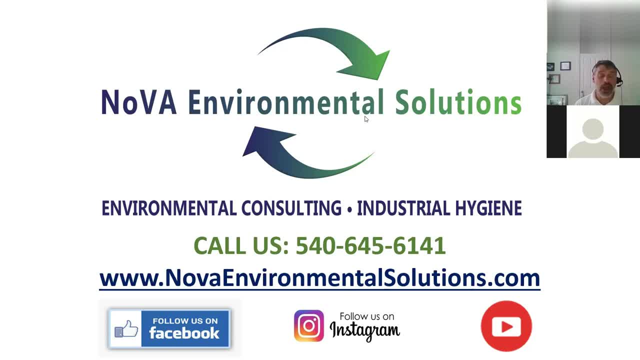 sampling for clients that that really want it. um, but it has to be vacuuming from carpeting only in living room and in a bedroom. that is the only way to get a true ermie score. it is comparing that sample, or those samples, to the index that was developed by set, by sampling. 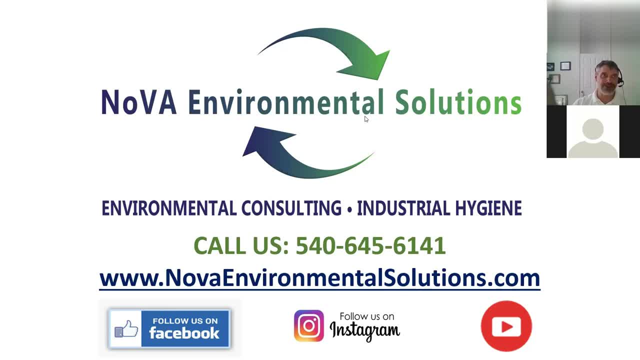 in a living room and in a bedroom it can only be on a two square meter- uh section of the carpeting- and for five minutes. that is the sampling method to get a true ermie score. um, i know there's a lot of companies out there that are offering that and people say, yeah, get it. it hurts me again, ermie. 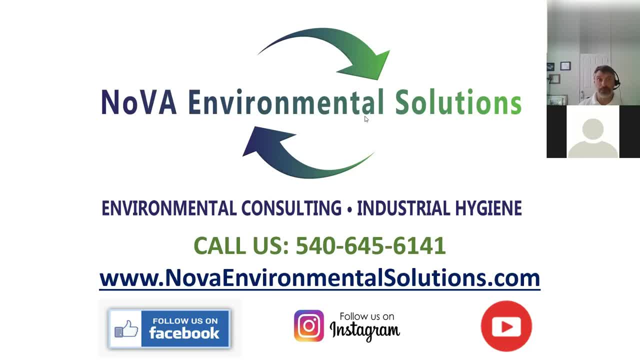 yes, again, it does show you what molds are present, and can it give some historical information to an assessor? it may, but it really does nothing as far as the sample is concerned, as far as evaluating the structure to determine if there's actually a growth source in the structure, 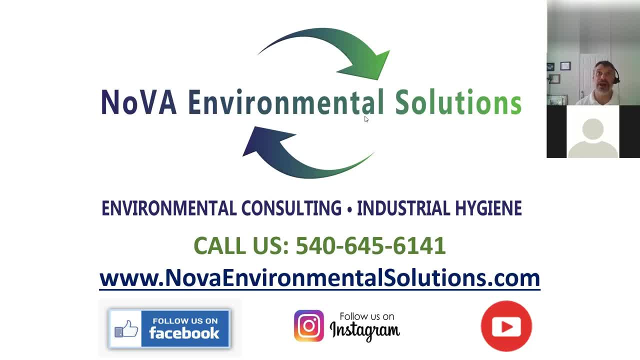 um, so my best advice is i, i personally, and- and i i have not advised that for clients or potential clients- just because from my perspective there's the data that we're receiving doesn't provide much information and it's really not not giving anything as far as uh. 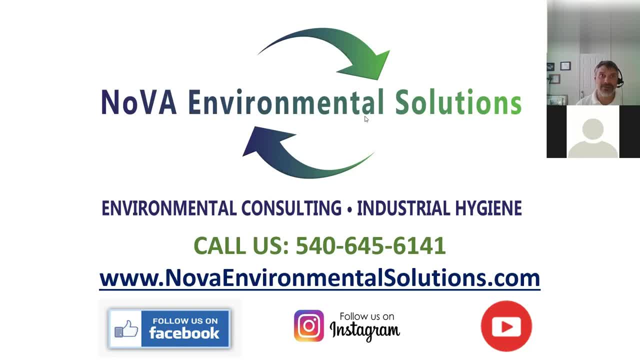 much more added value other than, um, you know that alone just doesn't tell any stories, so i went off my little tangent there. but if you've done it- and you and i don't want to make anyone feel bad- if they've- they done it, you know, and you may get some satisfaction with it, um, but again it, and it's something where, um, i'm 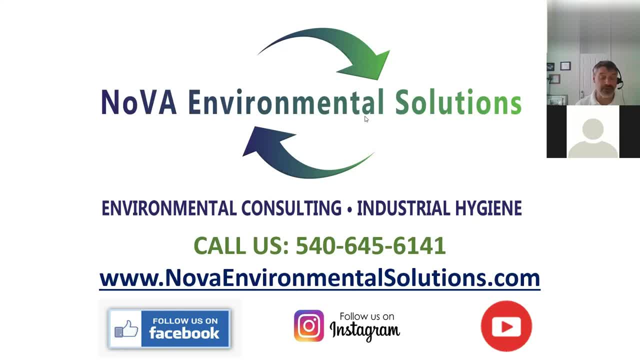 happy to you know speak with you one-on-one and feel free to call me or email me directly if you have a specific concern or question, even after this, and i'm happy to you know speak with you. i'm happy to go over no obligation, no, no, you know, no fees or anything like that. you know that's. 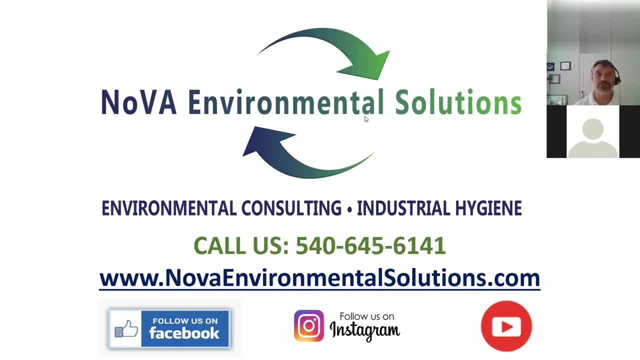 that's ultimately what i'm here for is to, and what i strive to do is to at least provide potential clients, or or even just anyone, information, you know, then that's that's reasonable, and and to allow them to make decisions. that's right for them. any other questions? i know we're getting past people's dinner time. 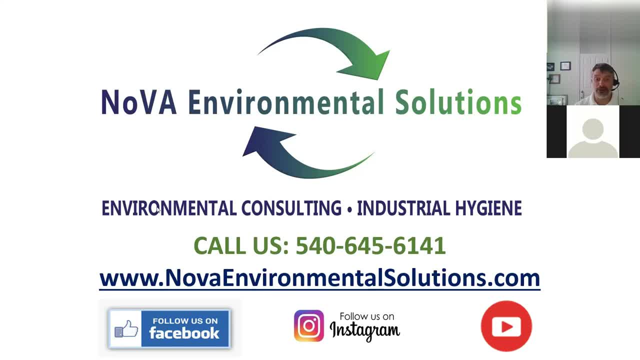 and if you all have again my, my phone number is up there. our office number is up there. um, if you want my email address, specifically, if you have a pen and paper, i could write that down. um, it's paul, my first name p-a-u-l at and it's my company name shortened up, so it's. 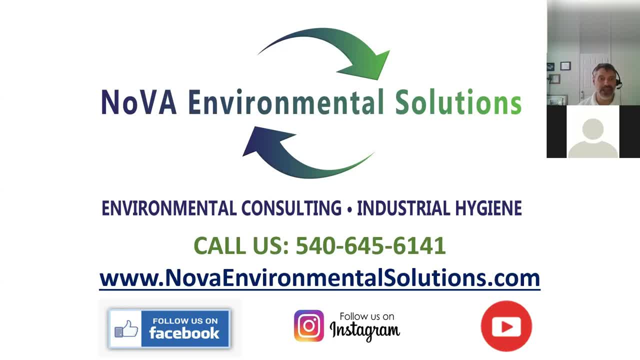 paul at nova n-o-v-a-e-n-v-s-o-lcom. well, paul, thank you, uh, for taking the time to talk with us. um, i know, i know that, um, i appreciate it and i know that everybody else does too. so, um, thank you again and um, if anybody, nobody else has, 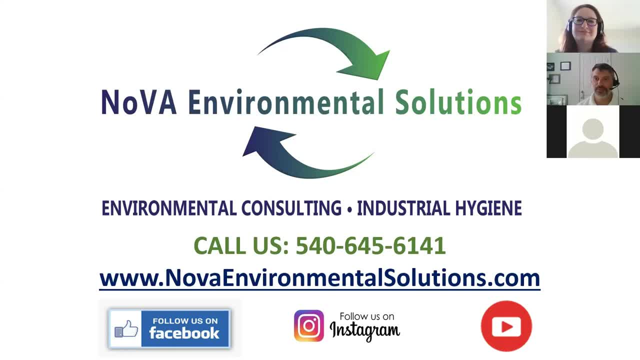 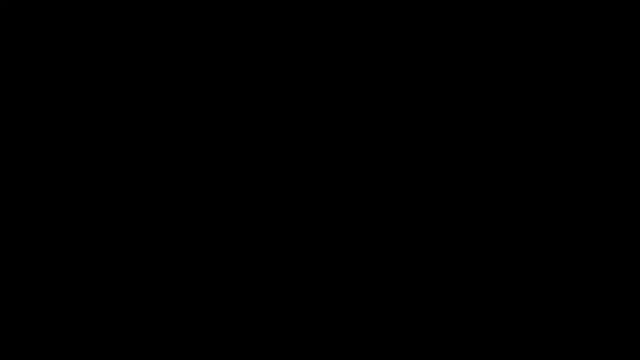 any other questions? we'll, uh, we'll close the. the zoom call sounds great. thank you everyone for attending. i really appreciate it. bye, everybody, you.